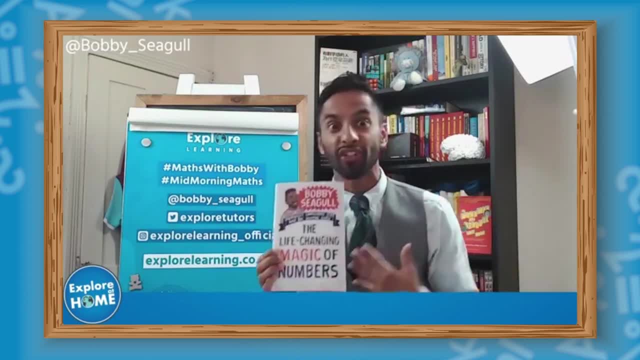 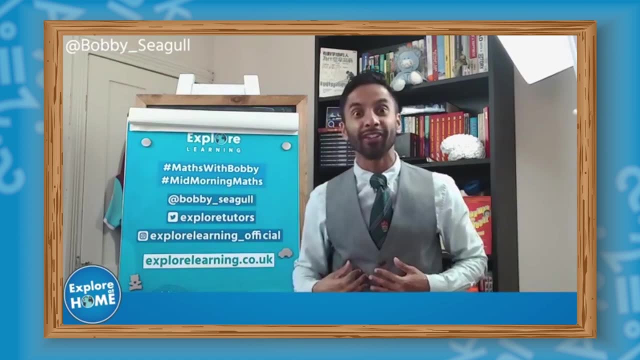 I'm also a presenter of the BBC TV series Monkman and Seagull's Genius Guide And we've got an announcement by next week. I'll be able to tell you when the new series is out, So I'm really excited. So I'm here with Explore Learning's, Explore at Home, And we're supporting 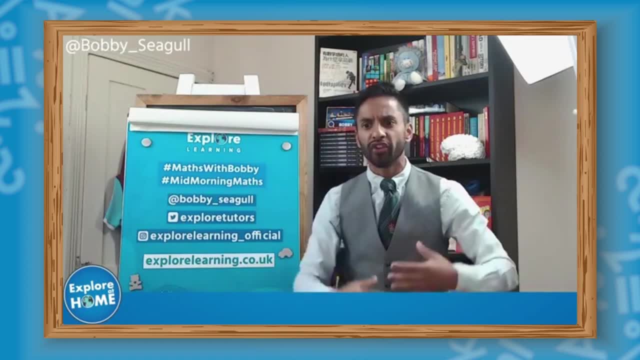 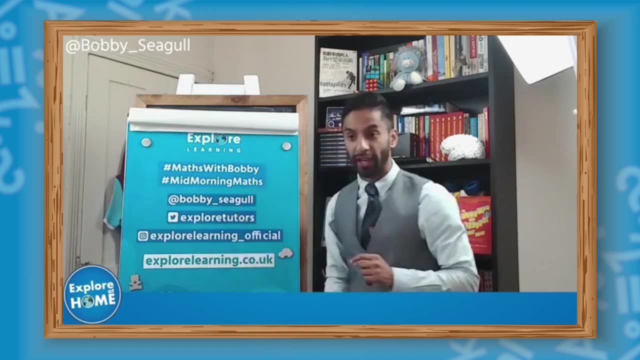 their mission to keep education going during these difficult times, And if you want to find out more about this, please visit our website, Explore Learningcom, And if you want to find out more about a free trial, go to ExploreLearningcouk. And we love social media, Ellie. 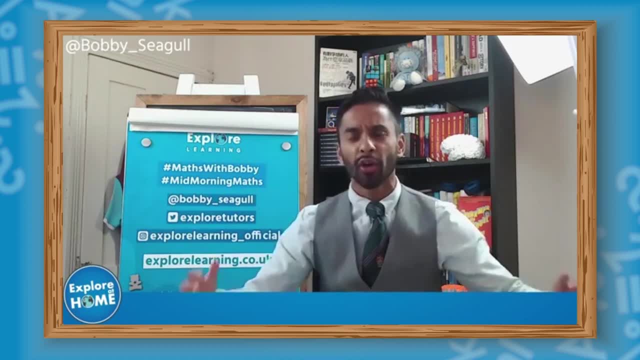 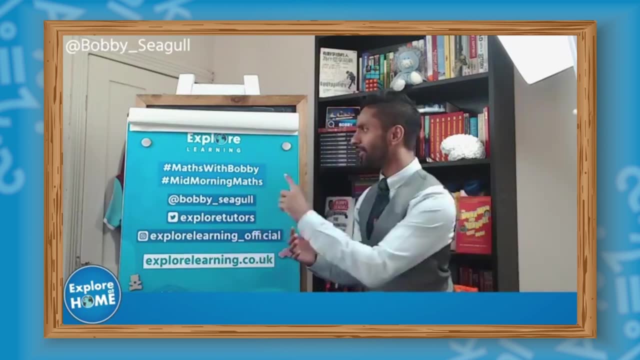 Age Six Findian, Charlton, Casper and Southend. We all love social media, So can you. if you're enjoying the lesson, enjoying bits of homework, can you message us? Hashtag Maths with Bobby. We're on Twitter at Bobby underscore Seagull: We're on. I'm on Twitter, Instagram, TikTok. 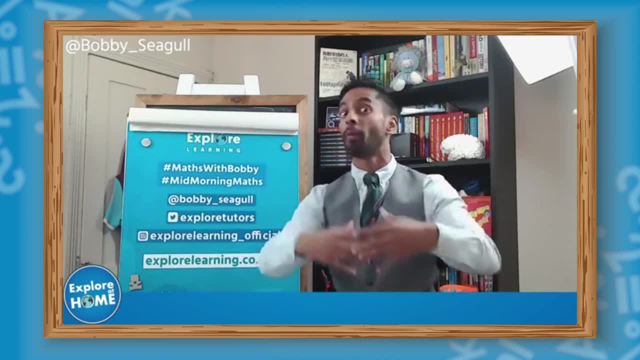 YouTube and Facebook. If you want to follow me to find out more about maths, go to Facebookcom- forward, slash, Bobby Seagull. So Facebookcom- forward slash, Bobby Seagull. Give me a like and then you'll be able to keep up to date with all my maths activities. 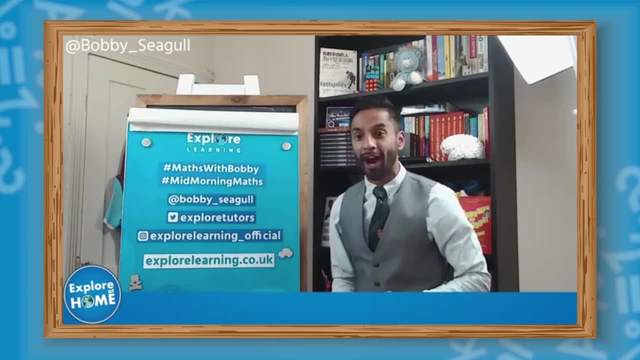 But also we're Explore Tutors on Twitter and Explore Learning underscore official. Hello Bo, Good morning to you. We're very excited. So today is going to be about something: patterns and sequences- But before we do that, we're always going to do a little maths mantra. 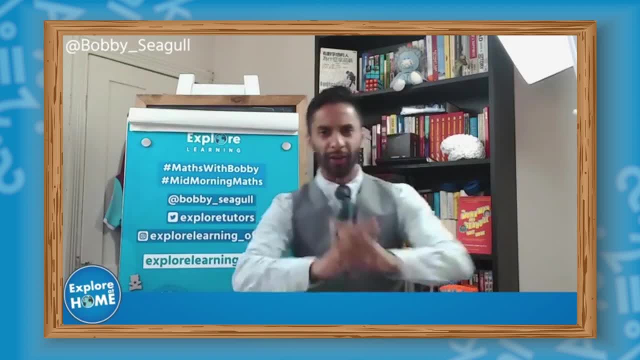 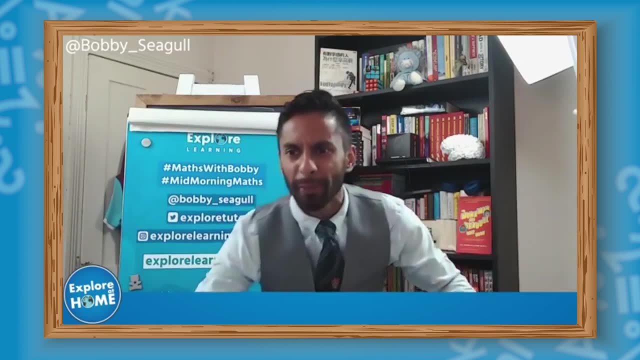 yeah, Maths mantra, Here we go. So remember, people come to me and say: Mr Seagull, I can't do maths, I can't do maths. But Bo, we know people can do maths, can't we? Shivan? we know people can do maths, So, Shivan, this is what. 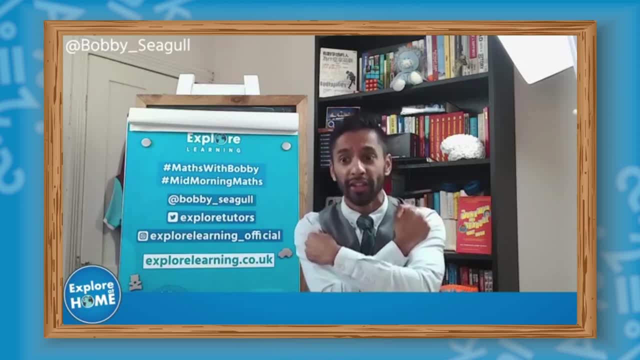 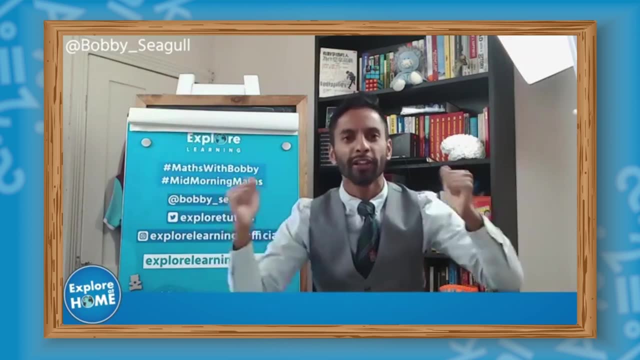 we do, We put our hands up. Emily and Holly, One, two, three go. Yes, I can do maths. Yes, I can do maths. Yes, I can do maths. Come on, Gabriel and Alexander, let's do that together. 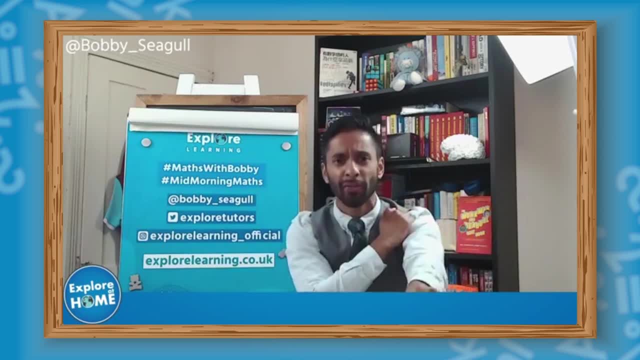 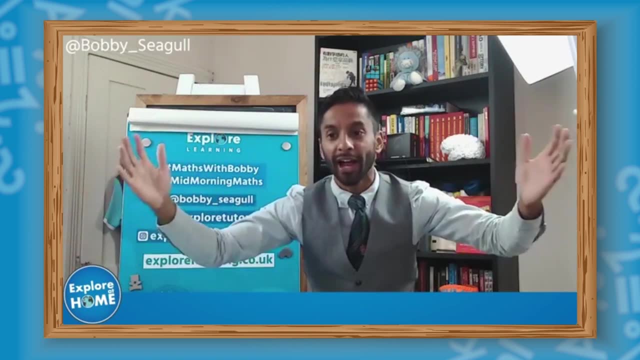 Come on, One, two, three go. Yes, I can do maths. Yes, I can do maths. Yes, I can do maths. Thank you, We've got people from Aberdeen and Sophie. We're all ready to go. So what is today? 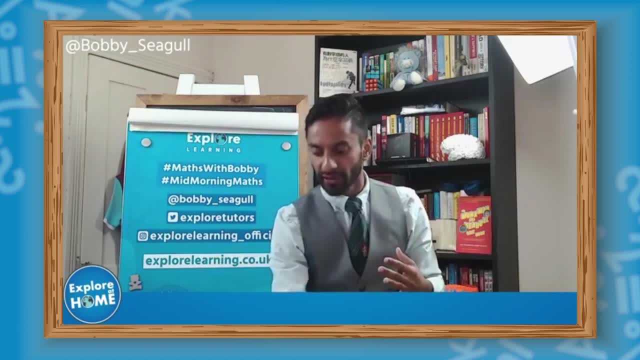 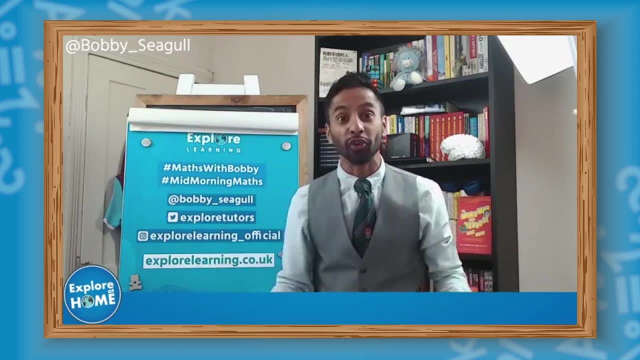 about. So today is week five- patterns and sequences- And next week we've got a special. Next week is actually going to be National Numeracy Day- National Numeracy Day, So it's almost like World Book Day, but a national celebration of numbers. So we're doing a. 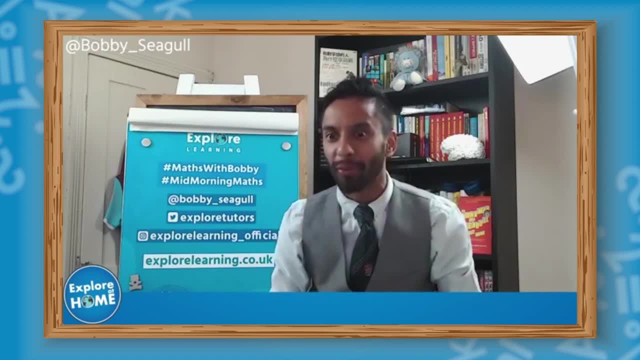 special lesson on how you can be smart with your money using maths. So that's National Numeracy Day next week, So the lesson is for those who aren't new, we've got Abel Abel. the lesson only works: 30 minutes of me teaching you a topic, working together, being interactive, And then a few. 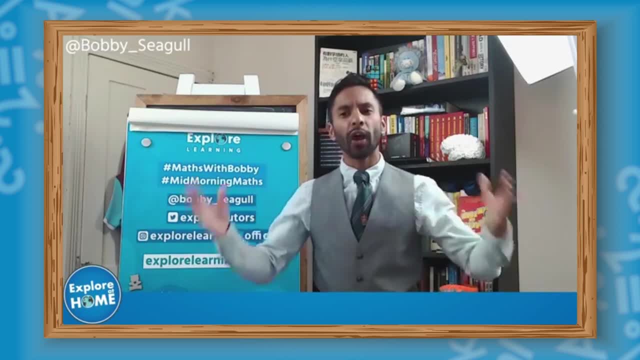 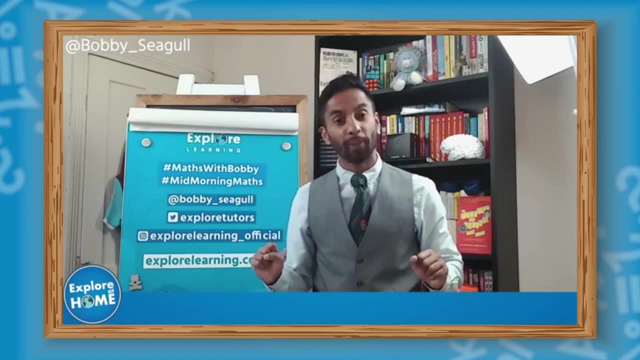 minutes of thoughts of Mr Seagull- positive ideas and how you can think in a more constructive way about the way you think about life. And then normally I have a few questions from parents or adults or carers and I'll try and support you there. Then we'll end the. 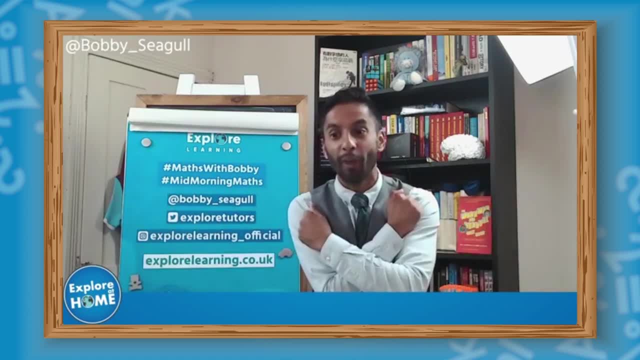 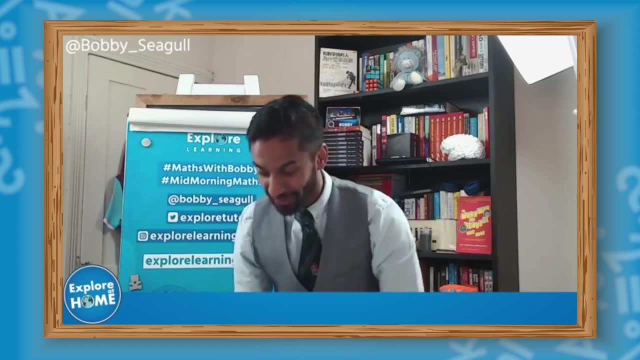 lesson with our maths rap. with our maths rap. How's the lessons? Hopper's eight years old, which is two times two times two. There we go. So we're about to start a lesson. Who is excited for some maths? Who is excited, Thomas, are you? 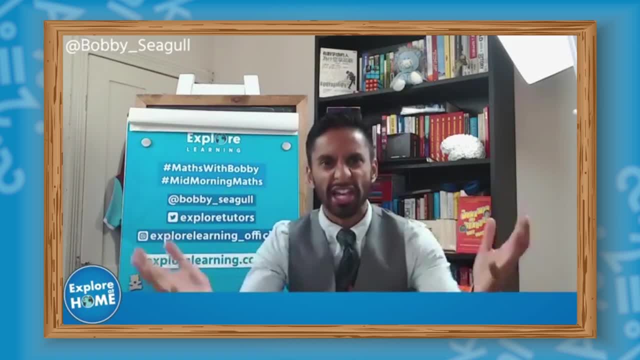 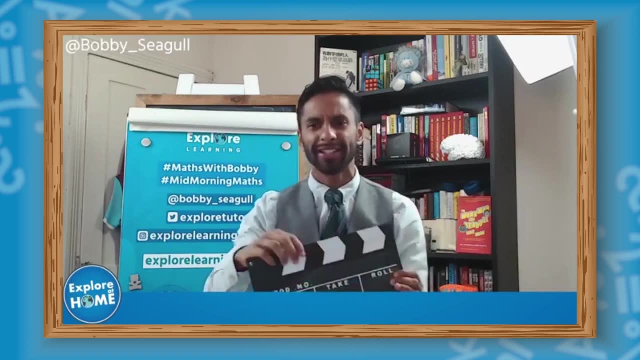 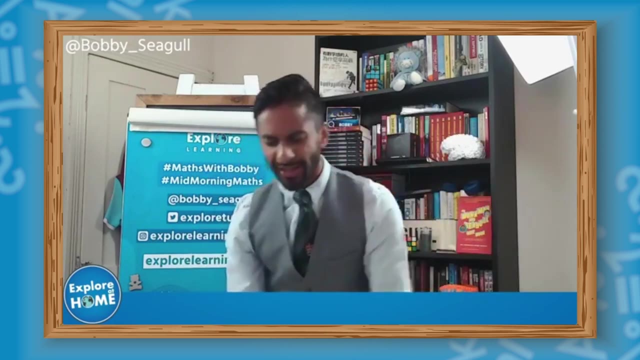 excited. Raj, Are you excited? Come on. Yes, Come on and give me an excitement. Yes, I'm ready for maths. The winner. We're going to get the party started. We're going to get the maths party started. Yes, Shivan, We're going to get it started. Here we go, Okay, So today's lesson. 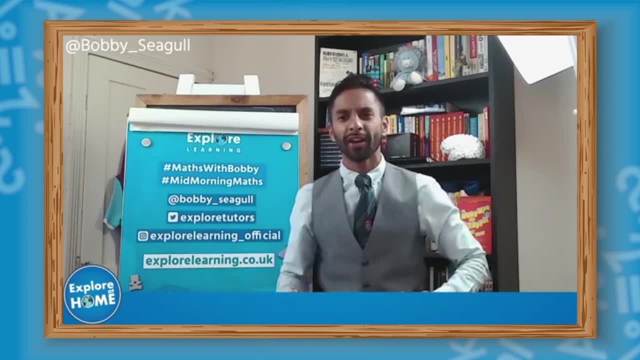 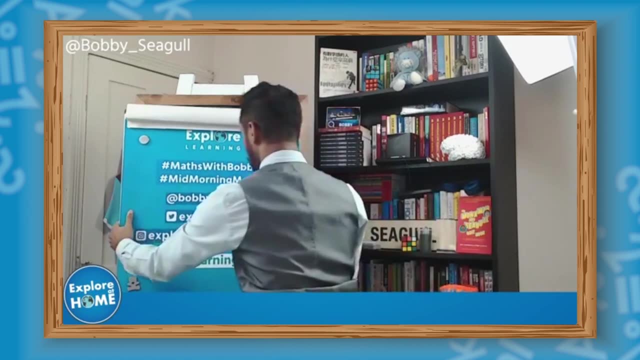 is all about patterns and sequences, but we're gonna, you know, fever. neither i like getting guests involved, and today we're gonna go to the boxing ring. i'm gonna move this out of the way. i'm gonna move this out of the way. i'm gonna go to the boxing ring and i'll 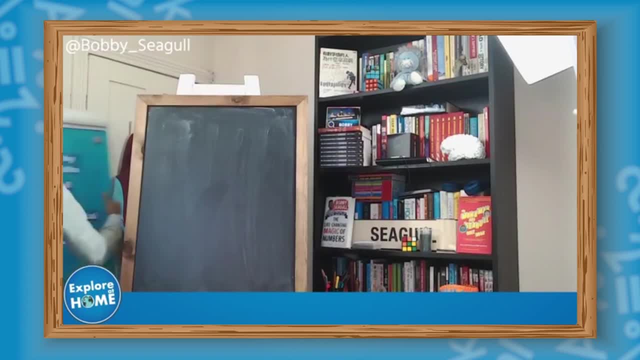 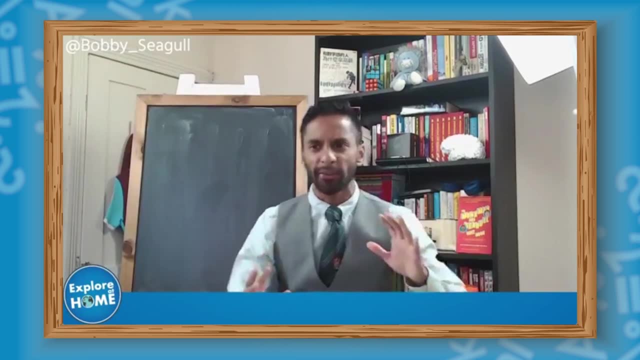 tell you why patterns and sequences are all about. i'm gonna move this way out of the way about reacting, about reacting to these, and boxers are quite good at reacting. they- they sometimes go up, sometimes they go down, sometimes they stay still. so let's get some boxing stuff on. i'm 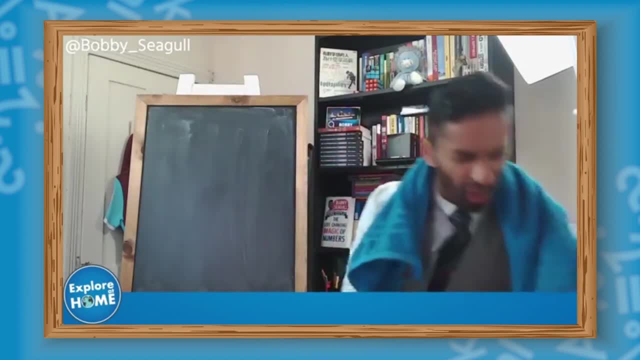 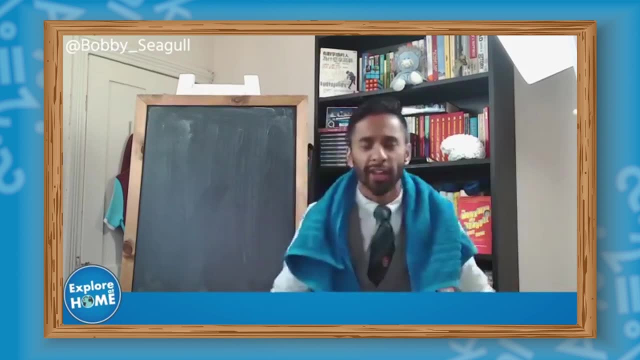 gonna get my um boxing towel. got my boxing pad. got my boxing pad hold on, hold on. got my boxing pad. are you ready? mr seagull is going to be your trainer today. yeah, yes, i can do maths, because today we're going to be looking at patterns. 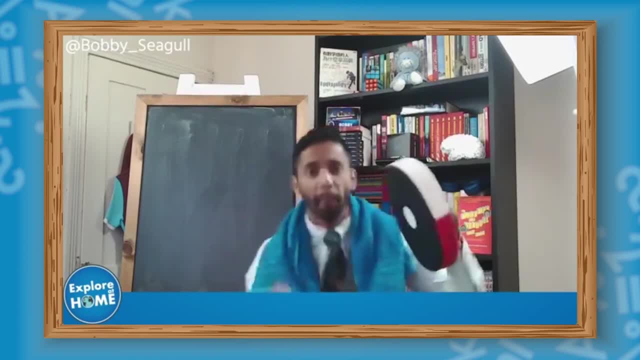 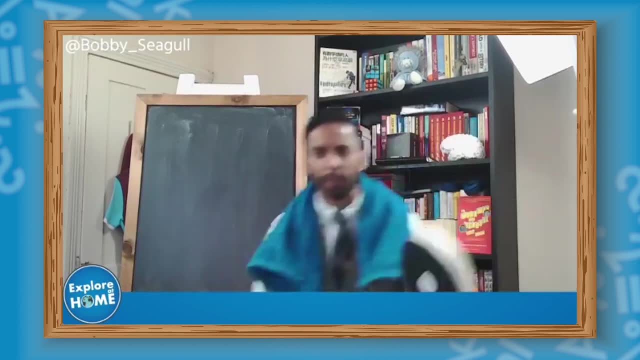 and sequences, and in the sequences things can go up, things can go down, they can stay the same, they can do anything, and boxers are people that have got to be nimble because in their game you need to be able to go up, down, stay the same, move around, it's all about. 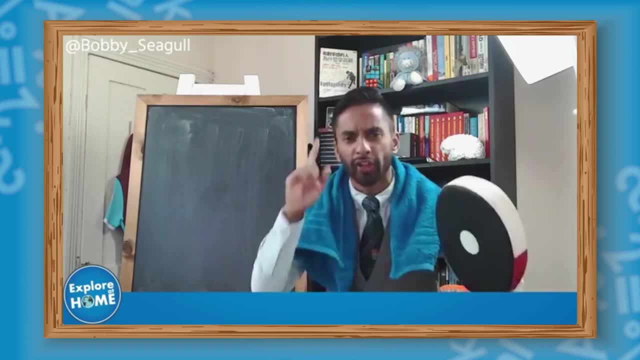 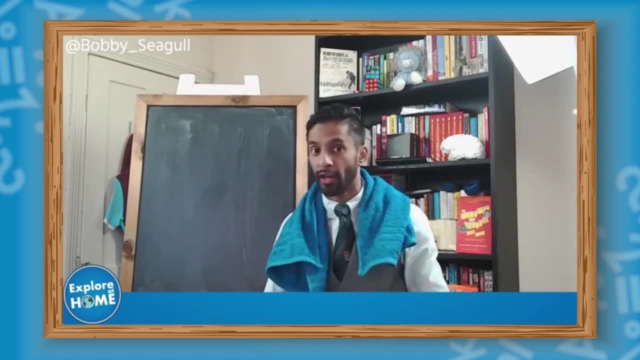 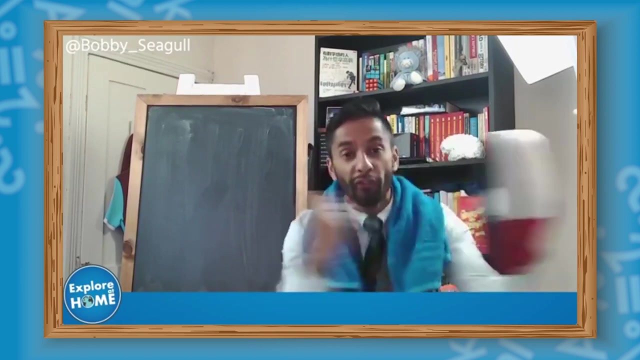 being nimble. so here we're gonna go. so i'm gonna. i'm gonna do a sequence of punches, okay. firstly i'm doing one, two, three, three punches, okay. and now one, two, three, four, five, six, six punches. now one, two, three, four, five, six, seven, eight, nine. 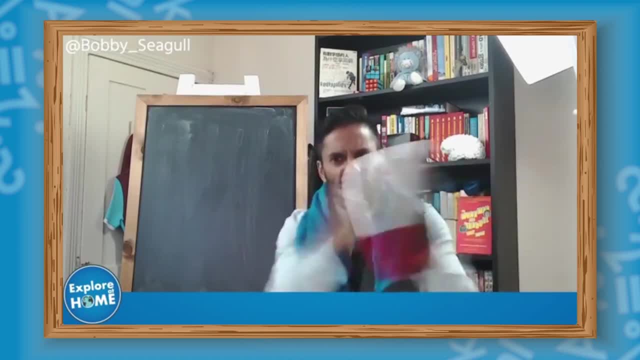 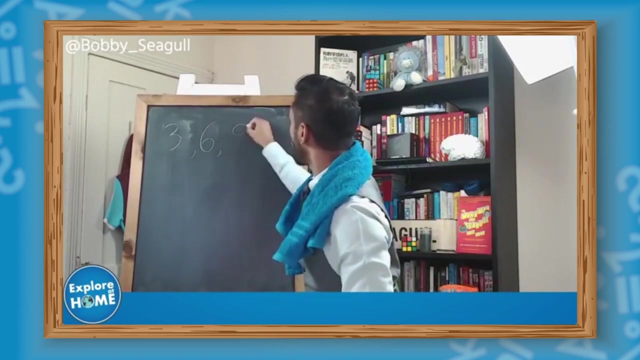 nine punches bow, and the last one is one, two, three, four, five, six, seven, eight, nine, ten, twelve, twelve punches. we're getting ready, so let's have a look at that. we're gonna start basic, we're gonna move on. so i did three punches first of all, then six punches, then nine punches. 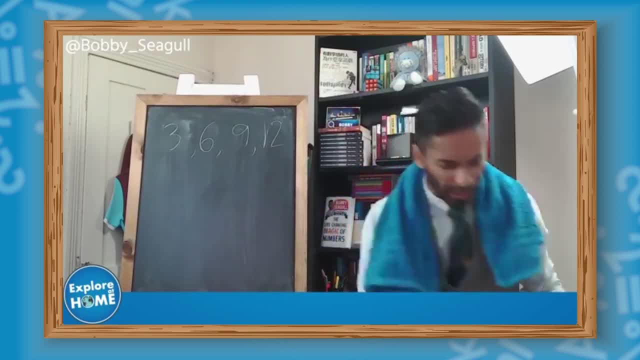 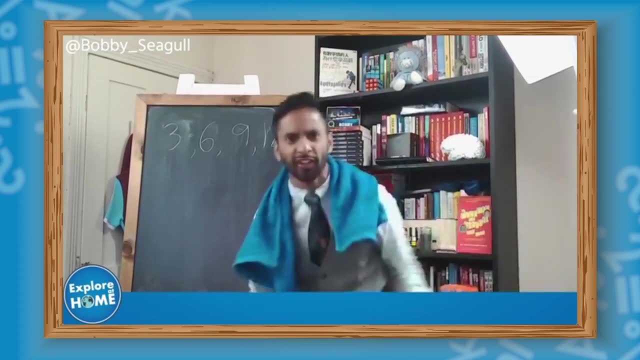 then twelve punches. come on. where do you think we're gonna? where do you think we're gonna end up after that? three, six, nine, twelve. you can chat in the put in the box there. come on, i'm waiting. i'm waiting for you to give me instructions. how many punches do i need to do next? i've done. 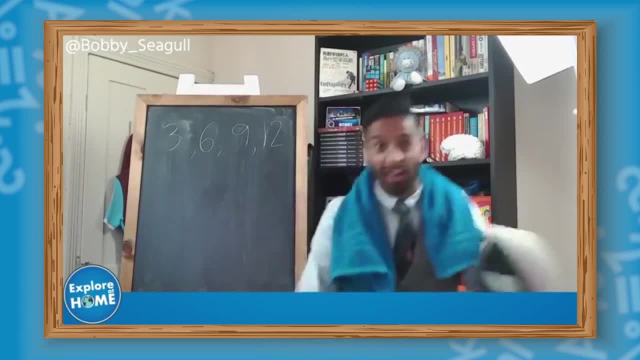 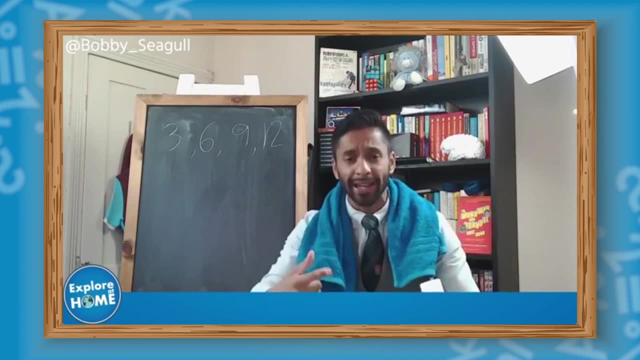 i've done three, i've done six, i've done nine, i've done twelve. come on, i need to know the next thing, my sequence for my training session. what do you reckon? so we've done three, then six, then nine, then twelve. i can hear you shouting through the 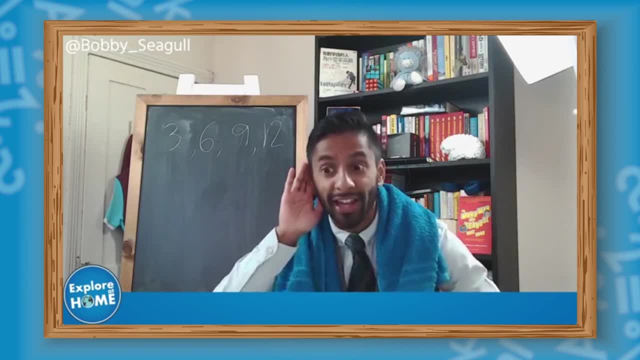 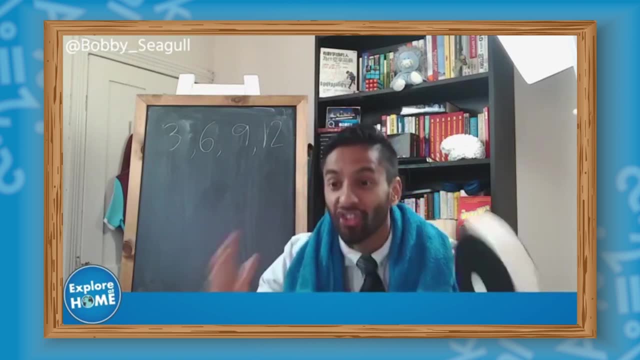 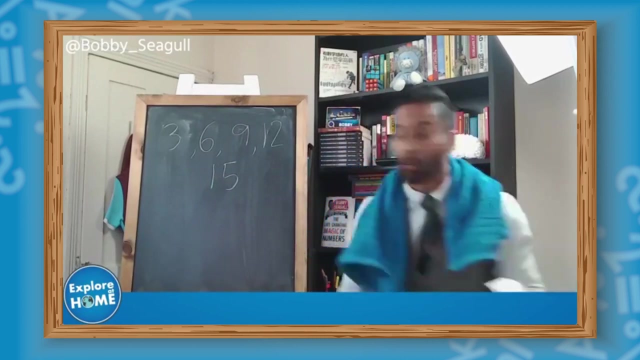 screens. come on, callum, tell me what it is. it is fifteen. yes, i think i heard shivan kia and misha shout it through the screen: it's fifteen, fifteen, well done so. the reason why that was fifteen was because they're going up in threes. 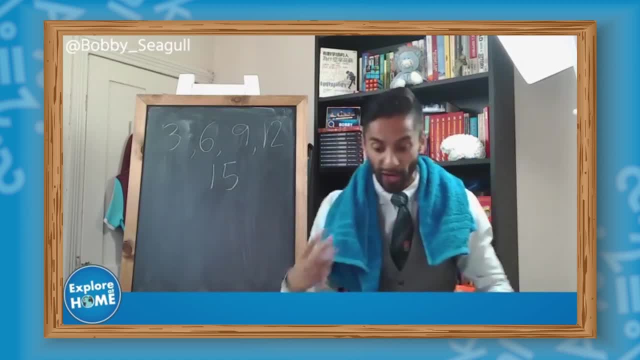 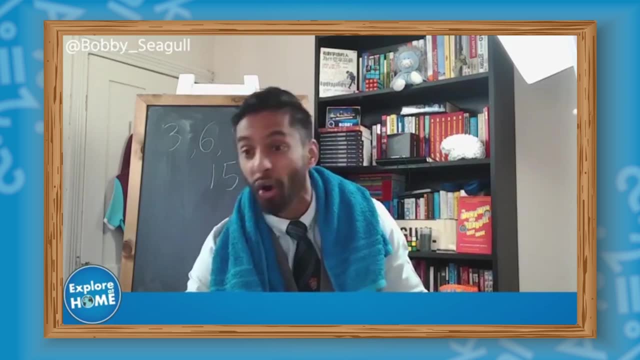 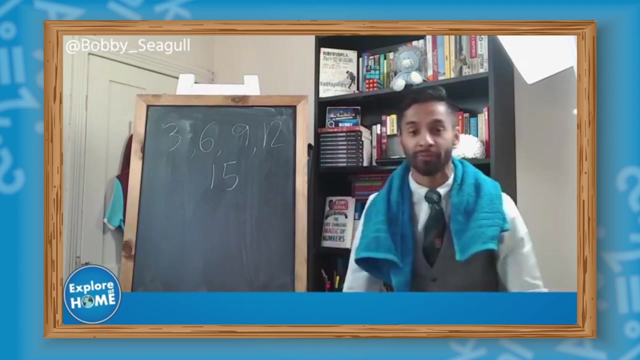 three, six, nine, twelve. we're going up in threes. let's try another one. let's try another one. toady says: do i do boxing? yes, i do. uh, box fit, box fit, i do like my boxing. so well done. lots of great answers, ooma ellie all got it spot on, so let's do the next one. so we're gonna. 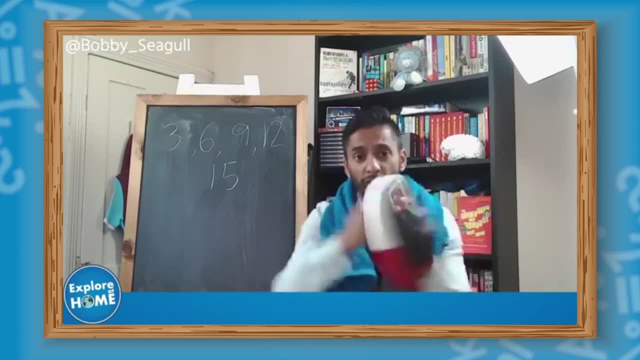 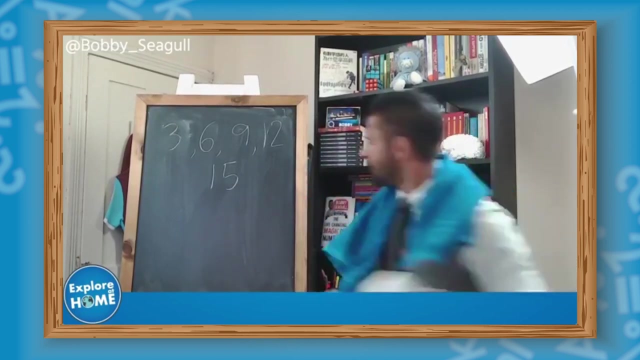 do another one, so we're gonna go down this time: one, two, three, four, five, six, seven, eight, nine, ten, ten punches. then one, two, three, four, five, six, seven, eight. now one, two, three, four, five, six, and the next one is one, two, three, four. so what is the mathematical? 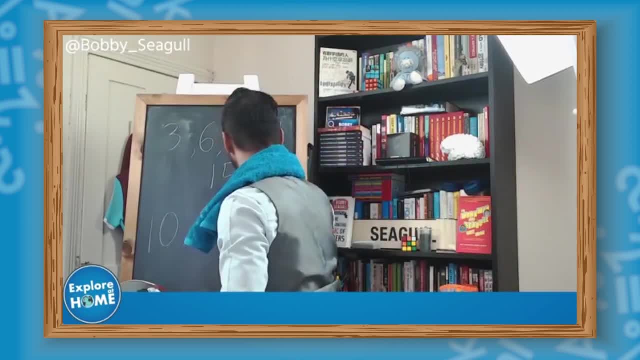 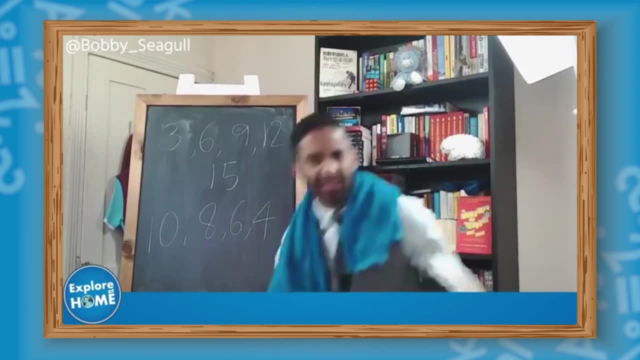 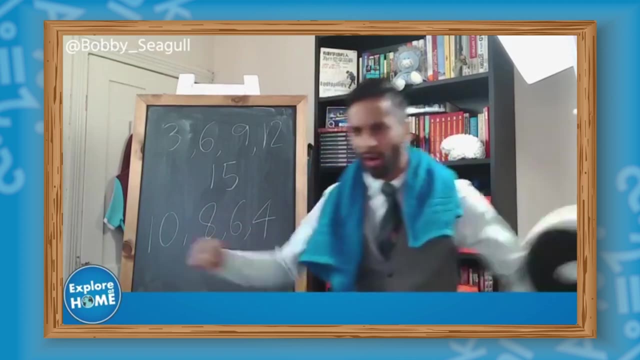 pattern as we go from ten eight, six four, so ten eight, six four. what's next now? so we've done, we've done some uh sequences in boxing. we've done ten eight, six four. so where are we going next? come on, what's my last bit? i need to know. come on, you have to let me know. 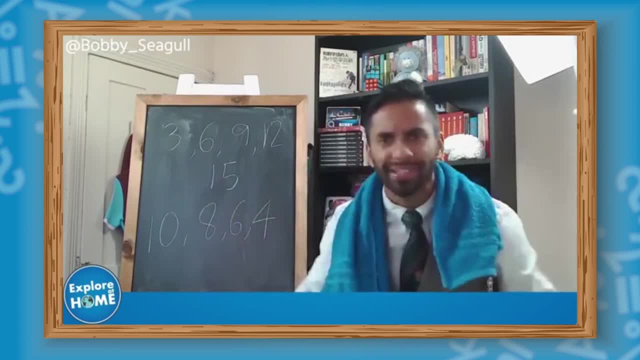 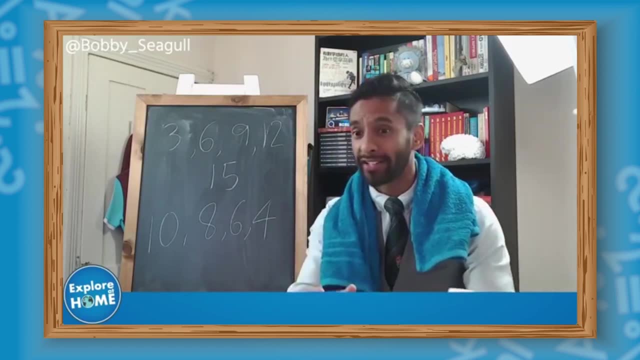 you have to let me know. come on, i'm ready, i'm ready, i'm ready for this session, but you need to tell me how many more punches Has it gone? 10,, 8,, 6,, 4, Zack. what do you reckon it is, Zack? 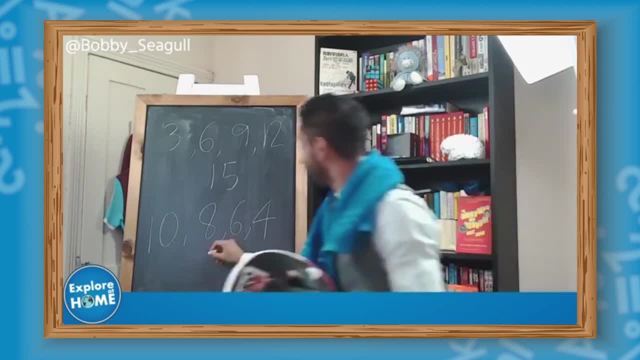 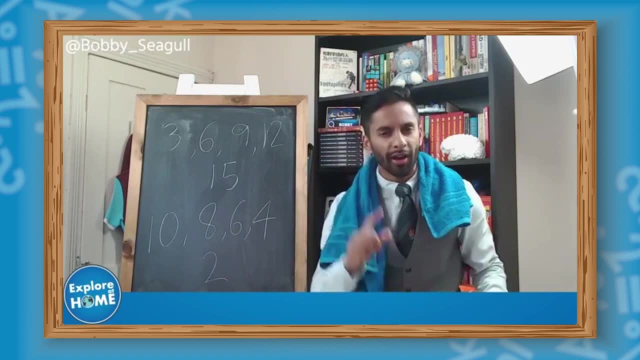 Rinky's got it. it's going down in twos. So this is 10, 8, 6, 4, 2.. Well done, So that's an easy one. that's an easy one. But now I'm gonna, I'm gonna test you. I think you're, you're saying, Mr Segar. 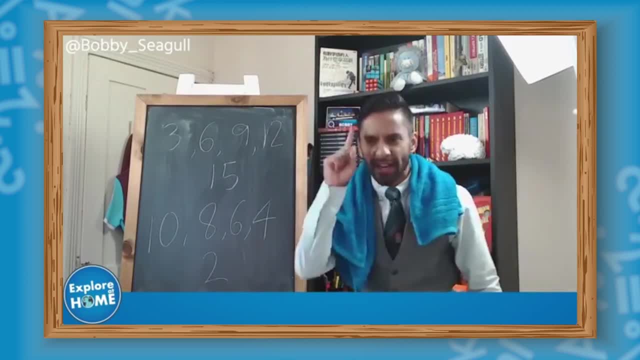 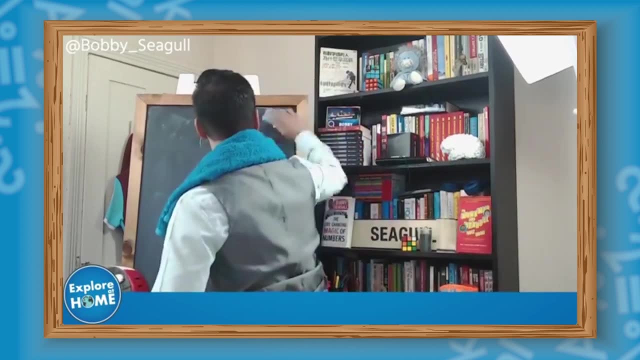 I know these boxing, these routines, these sequences are easy. Let's, let's try another one, Let's try another one. Who would have thought, Mr Segar, you've got, you've got the boxing, boxing training this morning, going on Boxing training. Okay, so this time, what we're gonna 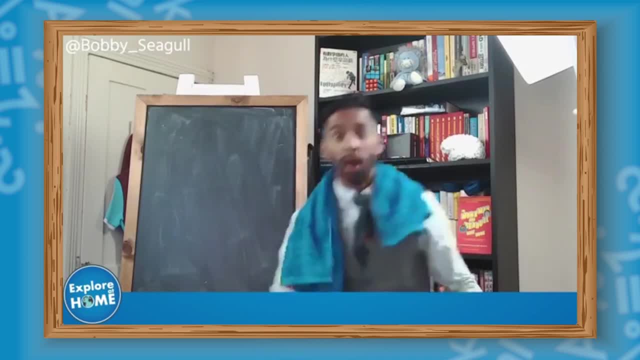 do is a new one, a new sequence, a bit more difficult. We're gonna go one, then we're gonna go one, two, Okay, then we're doing one, two, three, four, Then one, two, three, four, five, six, seven. 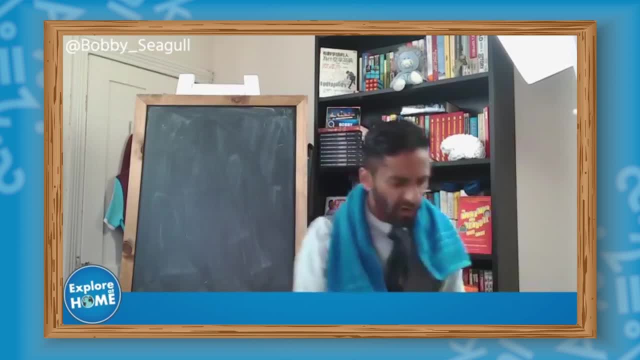 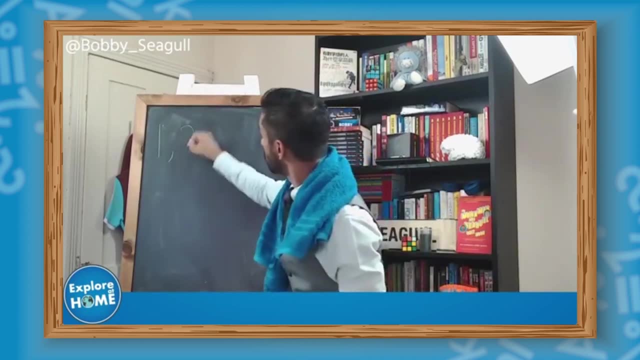 Then one, two, three, four, five, six, seven, eight, nine, ten, eleven. Whoa, what is this? This is gonna be? so it goes one, then it goes two, then it goes four, then it goes seven. 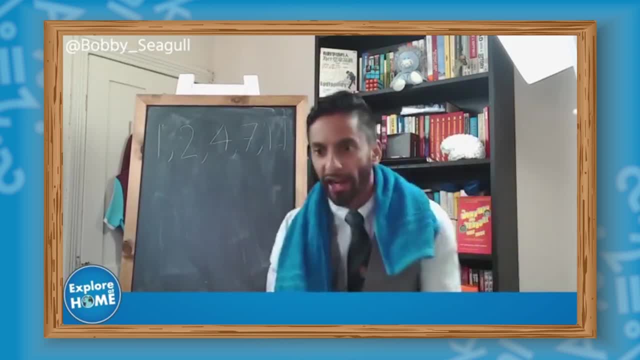 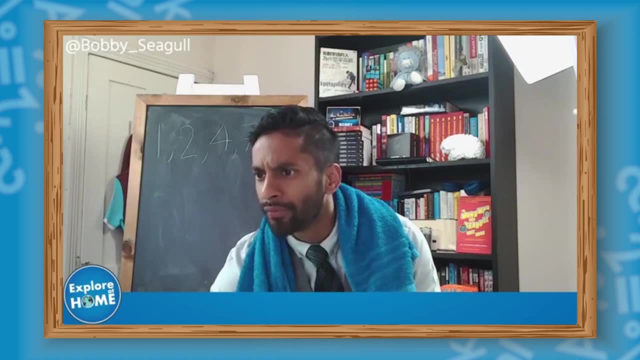 and eleven, So this one is a bit bit trickier. I'm gonna actually put this up for you, boys and girls, as a poll. I want to see if you've got this one, So have a look. Let me see if I've got it correct before I publish it. Yes, 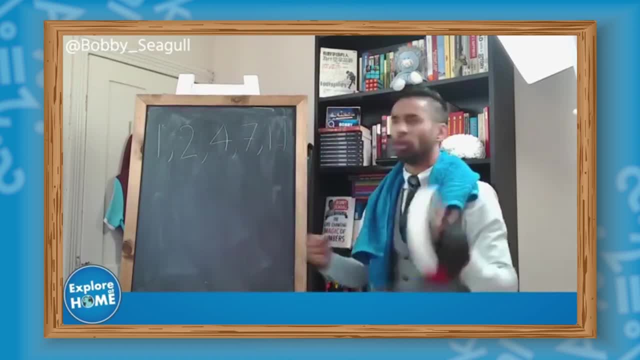 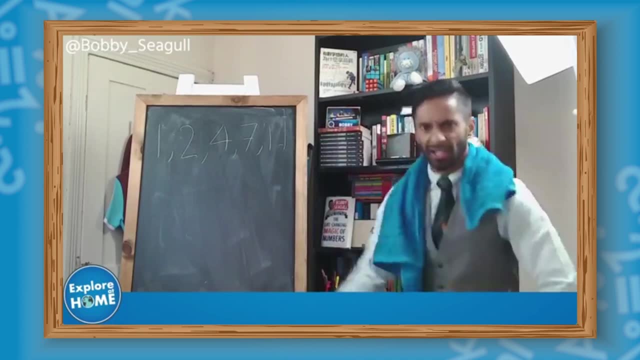 So have a look at this. It's coming up on your screen. It goes: one, two, four, seven, eleven. What is next? What is next? Come on, The boxer needs to. the boxer needs to get involved. I'm ready, I'm ready for this, but I need you to tell me what's next. 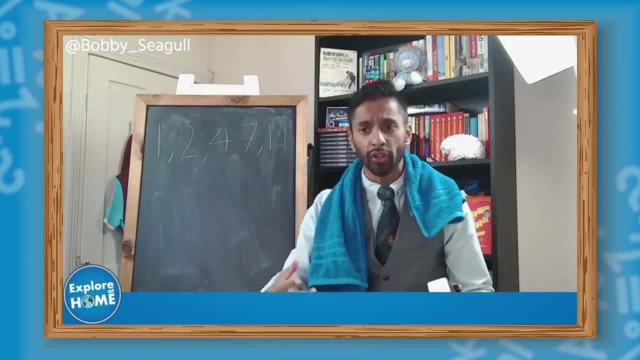 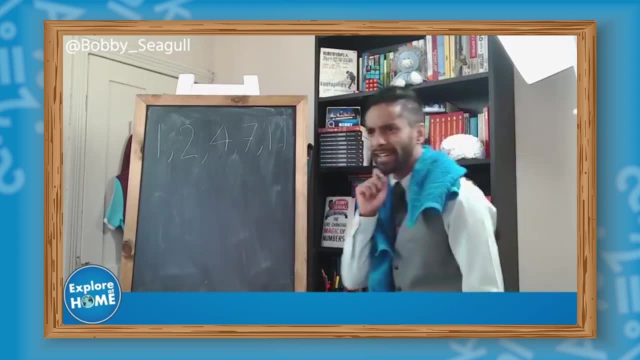 What's next, Come on. So you've got one, then two, then four, then seven, then eleven. So this is slightly slightly different. So, Amisha, this is slightly different this time. So I'm gonna poll up on the screen. You've got option 13,, 14,, 15, or 16.. 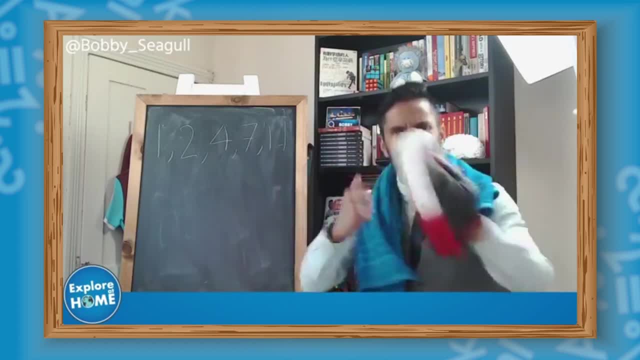 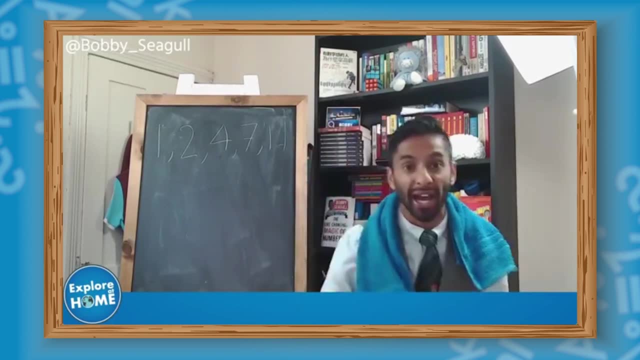 So we are doing patterns and sequences. if you just joined us And the reason that I'm I'm getting all boxing, is that boxers they involve sequences and patterns because sometimes they'll stay up, Some they'll stay down, Sometimes they'll go sideways and 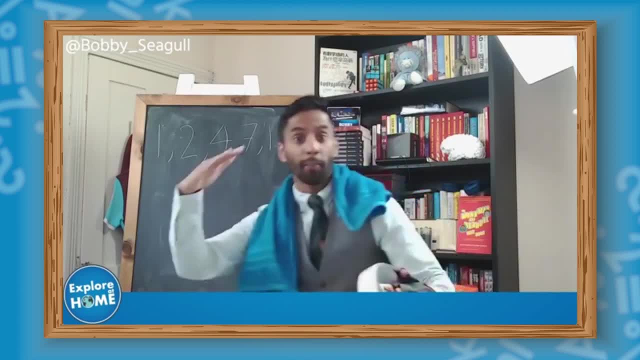 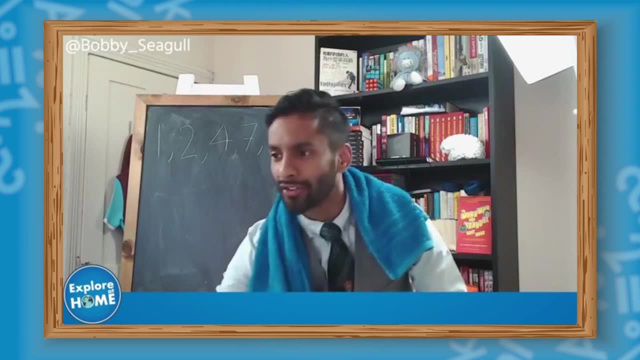 patterns and mathematics and sequences are similar. Things go up, down or stall. Okay, Laura says she's not quite sure what's going on, So let's look at the answer. Let's look at the answers. I'm gonna show you the results. So this is the closest poll we've. 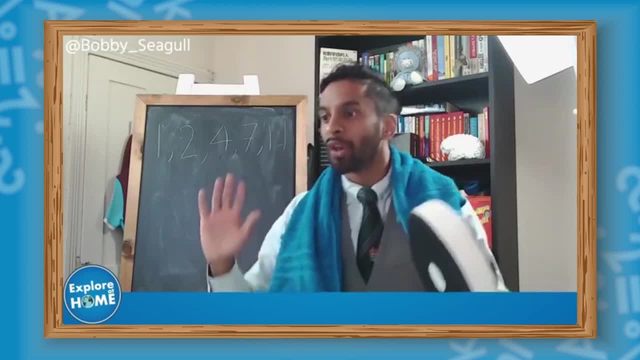 ever had. It shows, it's, it's. it's not an easy question. We've got half the people saying its 13,, 14 or 15, but we've got a great answer, Okay. so there we go. Let me double check this heredsfngs. 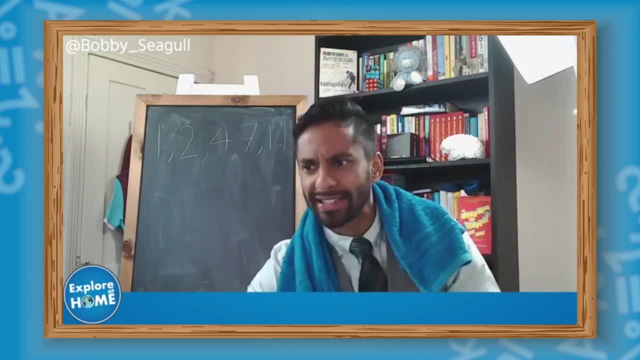 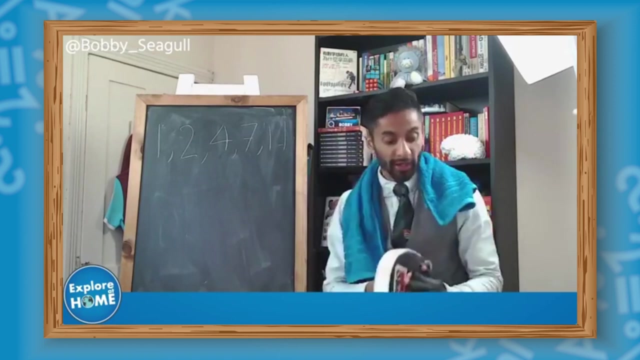 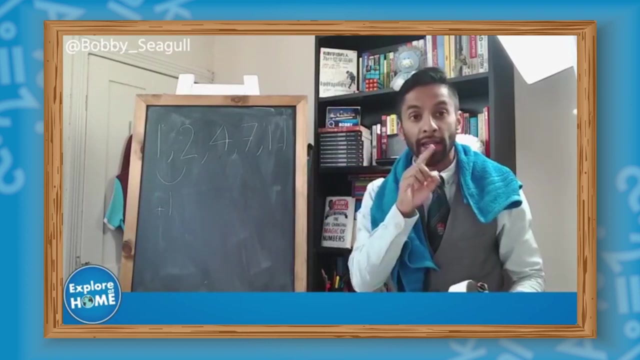 or 15, but we got a good, just about a marginal leader at 16. so let's have a look. so the answer was actually- I'm going to show you the poll- it was 16. it was 16. I'm going to show you why. so 1 to 2, it goes up by. you add 1, we add 1, then 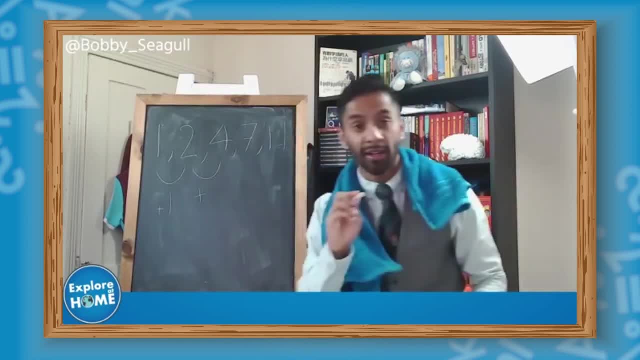 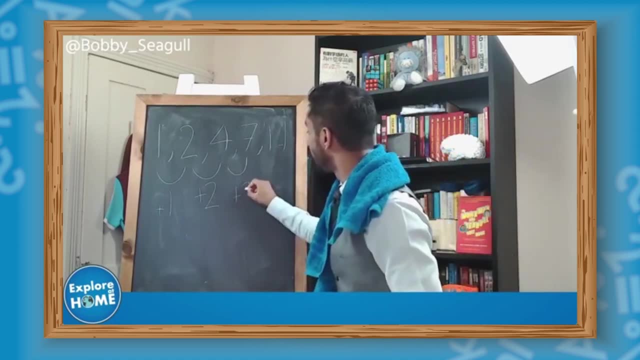 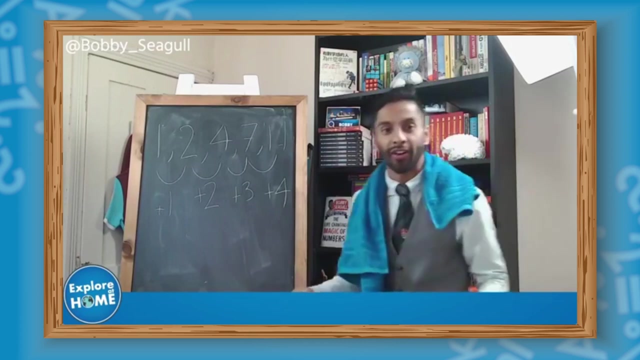 2 to 4, we add 2, then 4 to 7, we add 3. it's time to spot a pattern here. then 7 to 11, we add 4. so each time we're going up a bit further, we're adding 1, then. 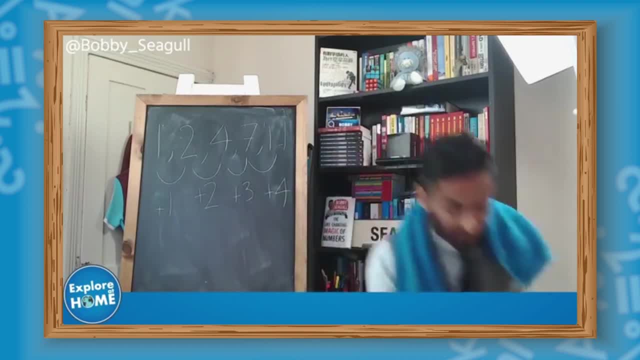 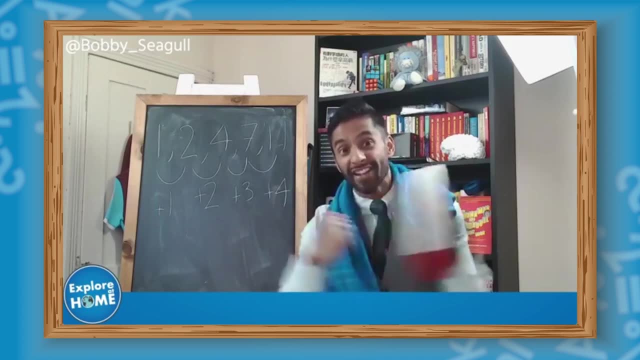 we're adding 2, then we're adding 3, then we're adding 4, so the last one we add 5 is 16. so 1, 2, 3, 4, 5, 6, 7, 8, 9, 10, 11, 12, 13, 14, 15, 16, there we go, there we go, so. 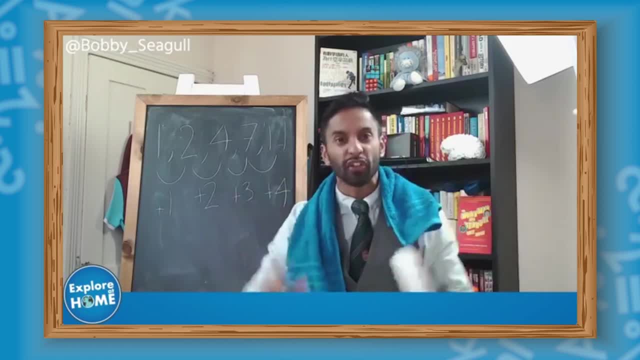 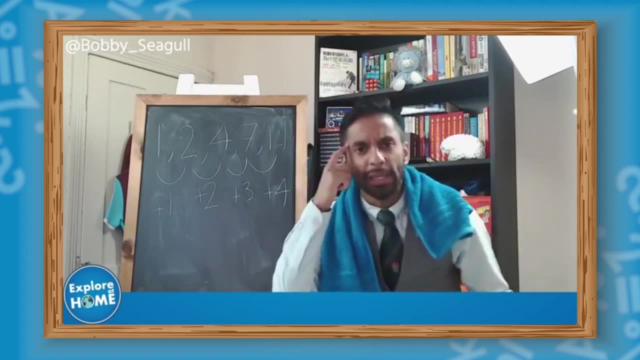 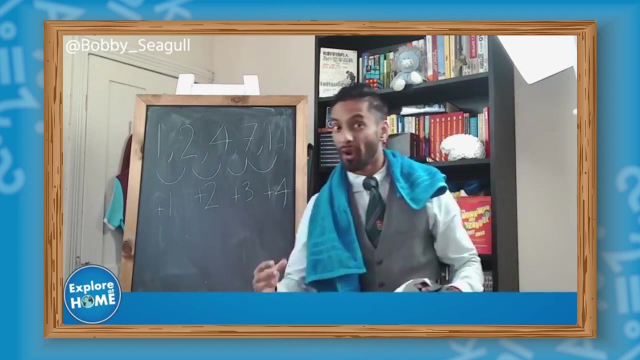 that was so the poll should be in your Facebook screen if you look up. so that is a mathematical sequence. and again these sequences. you got to keep your wits about you, because sometimes they go up in a certain number, sometimes they go down, sometimes they get smaller, sometimes actually, you'll find 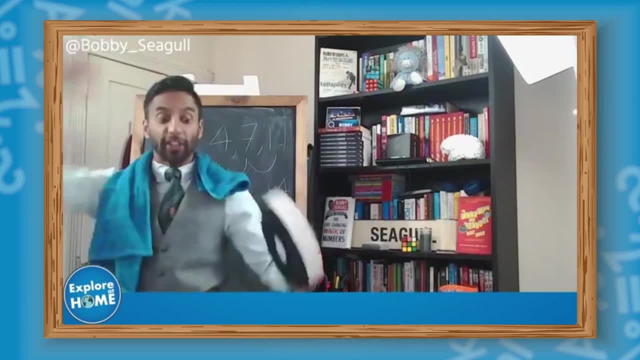 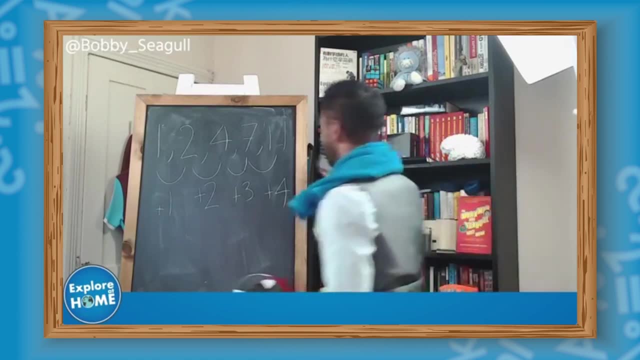 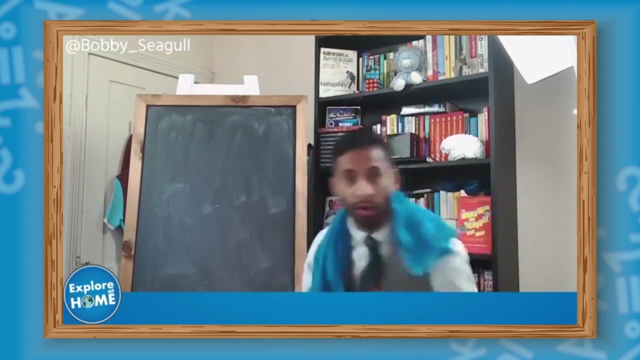 that they get larger and larger and larger and larger the gaps get bigger. so you got to really keep your brain thinking. so we'll do a couple more, we'll do a couple more and I've got a really exciting part of the lesson, even more exciting than boxing and mathematics. think I need to. I'm tired. 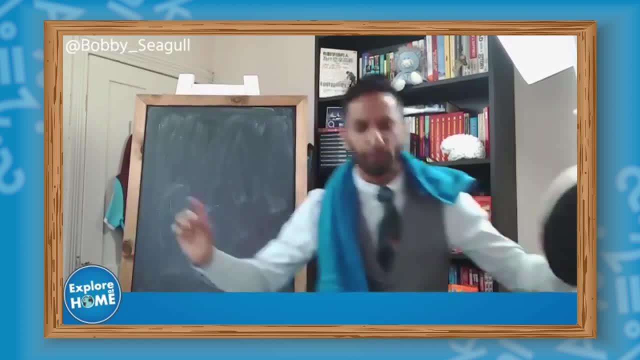 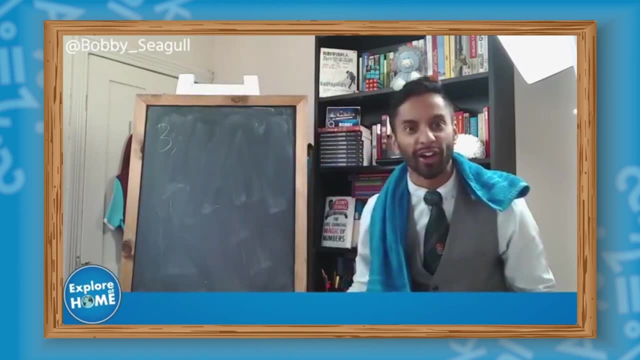 let's get in, okay. so imagine, now I'm not going to do these boxes because I'm going to be here a long while. so imagine we have. so I did. I started doing some boxing when I went to university. it's more box fit now I don't want to get my head. 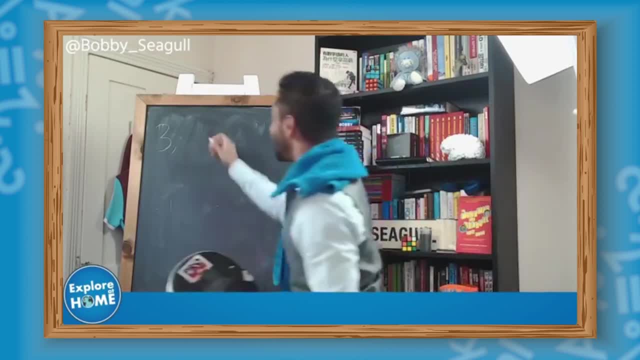 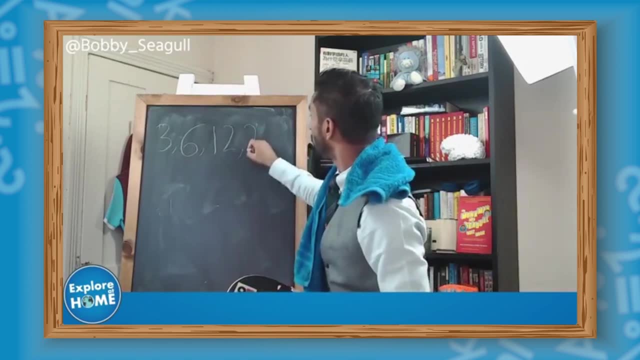 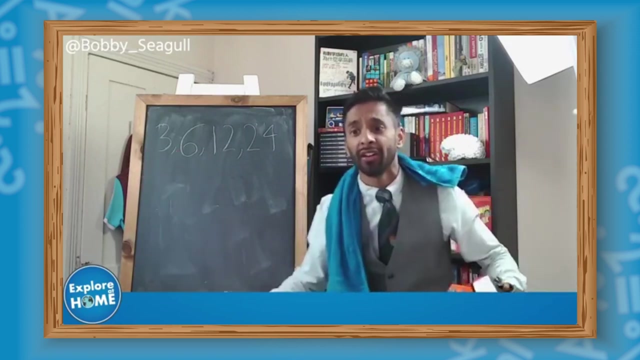 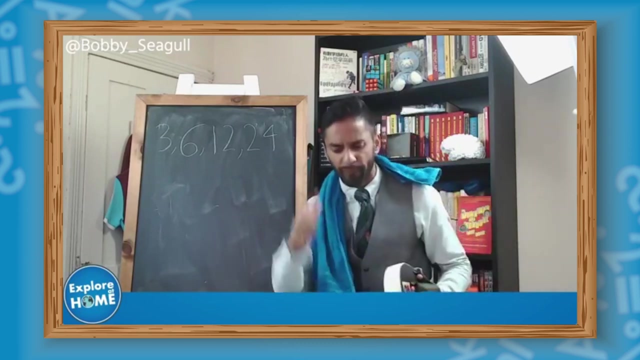 damaged because it's non contact boxing. there you go. so imagine we've got 3, then 6, then 12, then 24, 3- and I'm not going to do 24 punches because I will be exhausted. so 3, then 6, then 12, then 24. what do you reckon is next so? 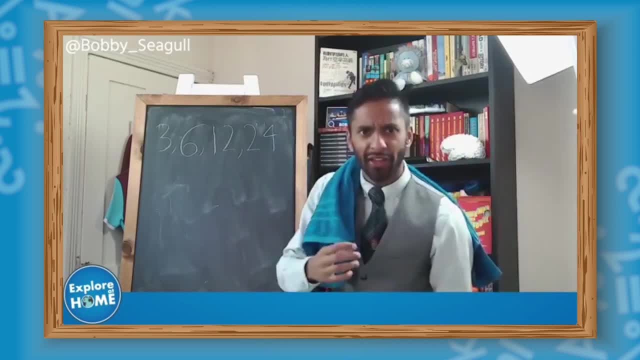 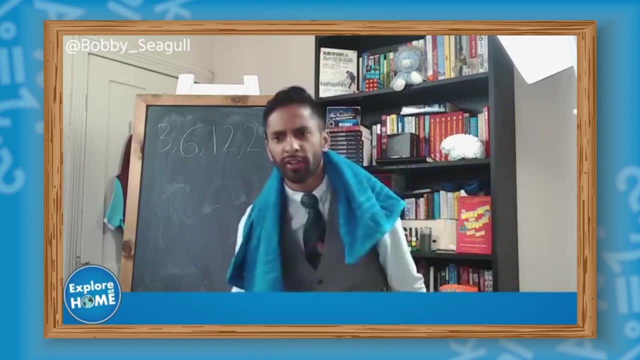 going to do 24, so 3 then 6, then 12, then 24. what do you reckon is next? so going three then six, then 12, then 24.. What do you reckon is next? So it's going to be, if you look. 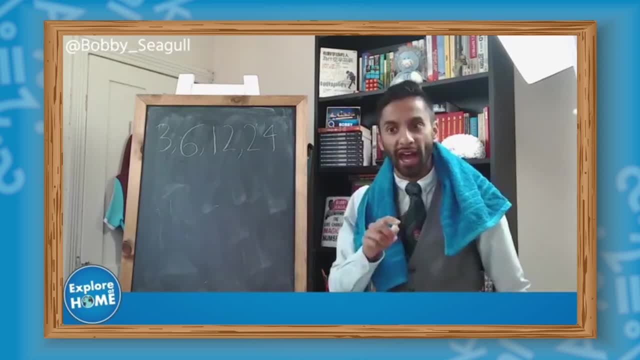 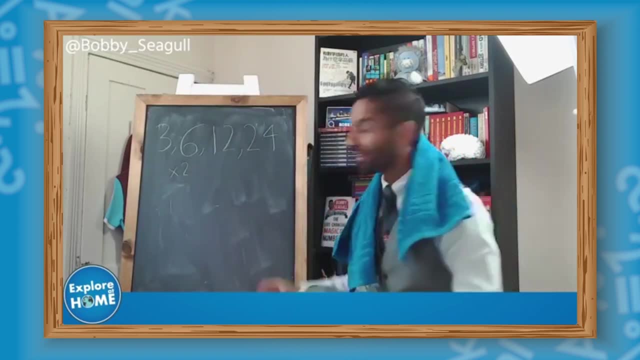 it's going up by three, by six, by 12.. You can look at that, but actually meters got it right. We're doubling Three to six, we're doubling yeah, And then six to 12, we're doubling again. 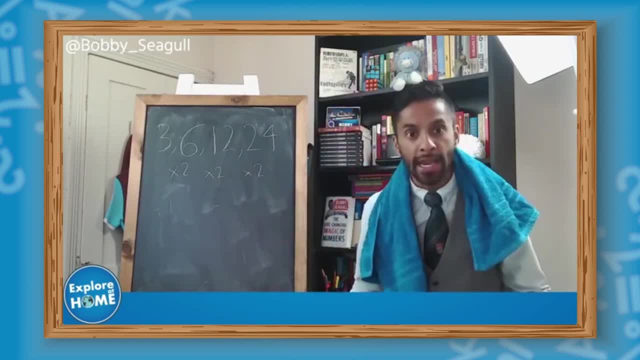 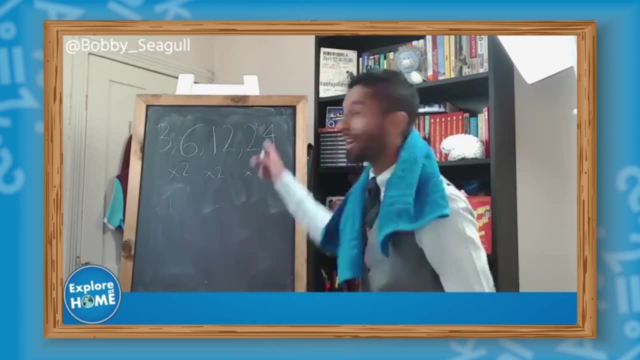 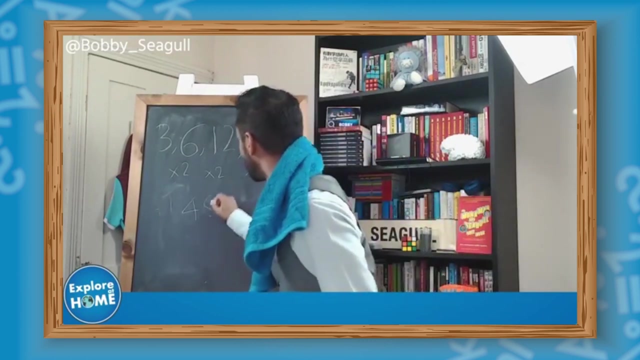 Then 12 to 24, we're doubling again. Okay, do you think I'm going to sit there and do double number of 24 boxing punches? Not today, but I can tell you the answer. The answer, Ritesh, is correct. She says it's 48. And if we double that the next one, we get 48 times two. 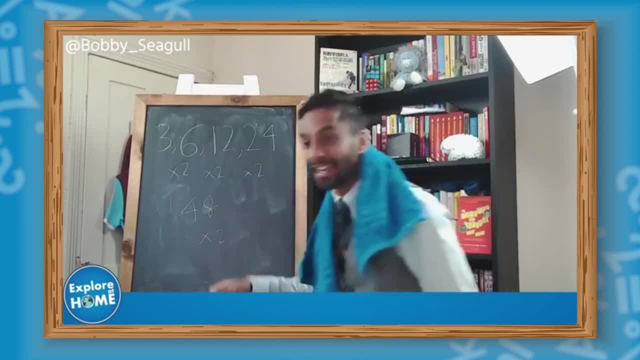 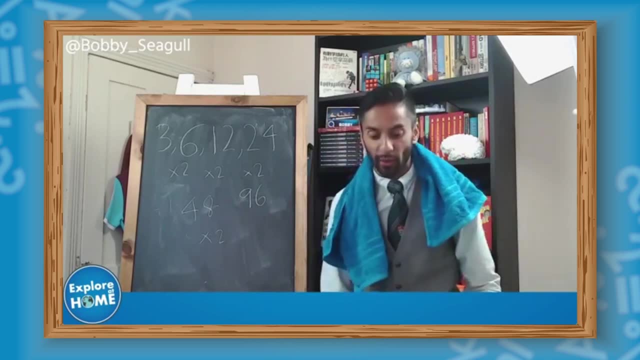 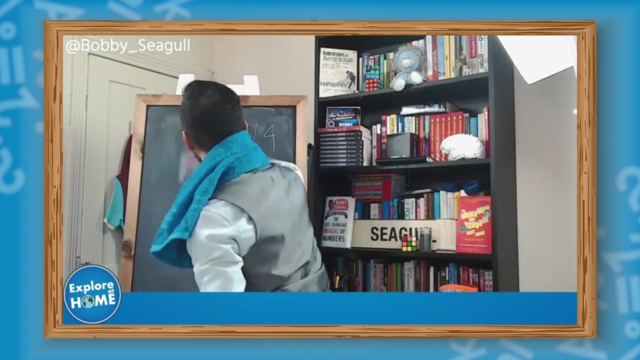 which is 96.. Yes, it's good, I've got a few people on the ball. Johnson Nathaniel also says we're doubling it. So we're doubling the sequence. We can double things. We'll look at another one. I want to do one more, one more with you. Let's have a look at another sequence. another sequence. 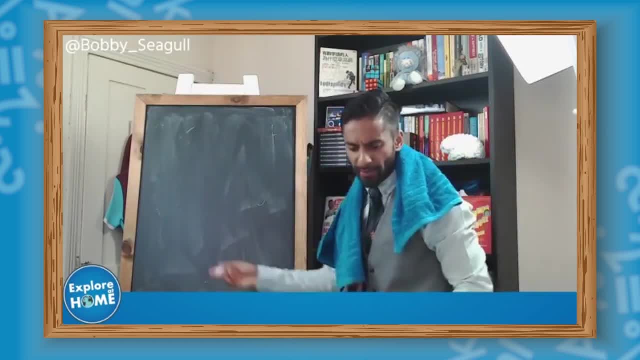 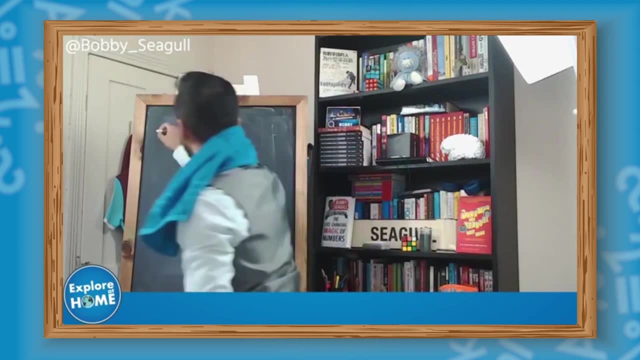 I want to see if I can test you on one. So imagine we have to this one here. This one is a bit trickier. okay, This one's a bit trickier, So 31.. Okay, this one I'm not going to be doing. 31. 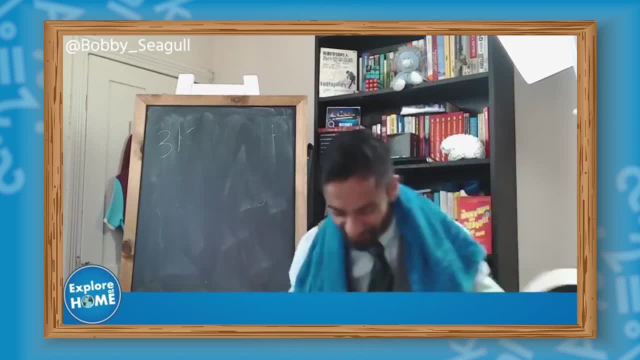 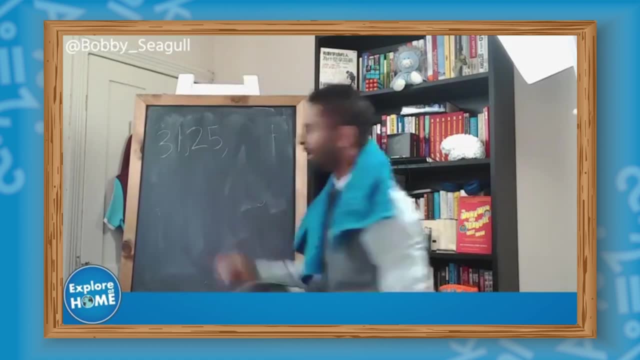 punches. okay, Even for you. as much as I love maths, I'm not going to do 31 punches. So 31,, then 25.. So 31, then 25.. This looks a bit strange. Then 35. Now you're thinking where's this going? 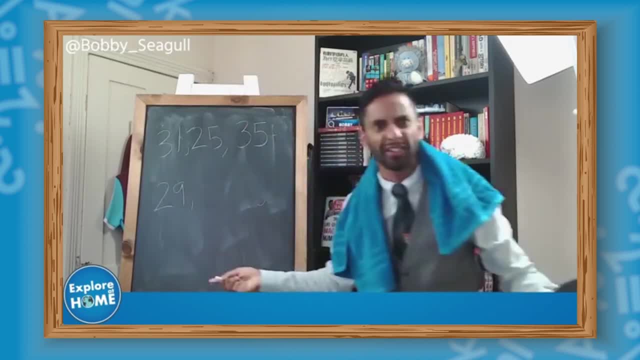 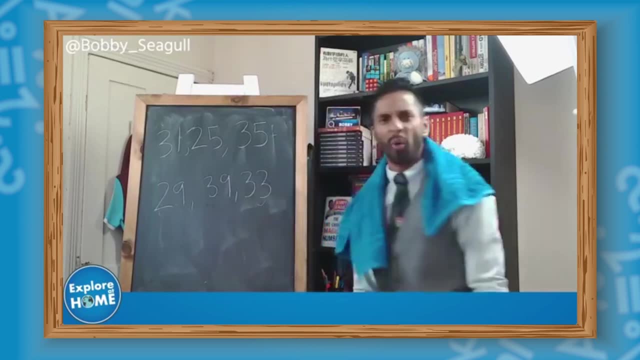 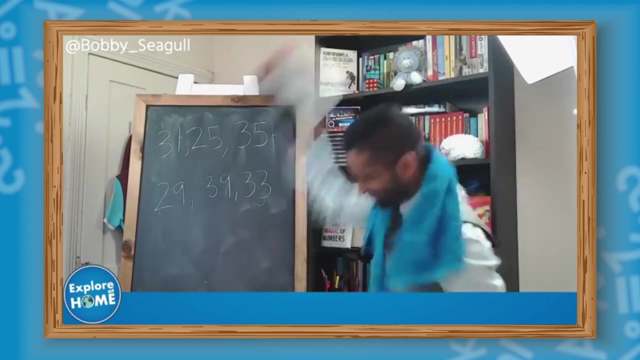 Then 29.. What on earth is this boxer doing? He's a mad boxer. Then 39,, then 33.. What is this boxer doing? What could he possibly do? He's crazy, this boxer. He's nuts. What is this boxer doing? I'm not happy with this sequence. What is he doing? He's doing 31,. 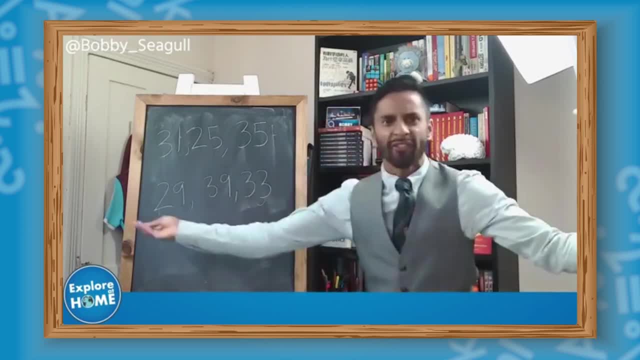 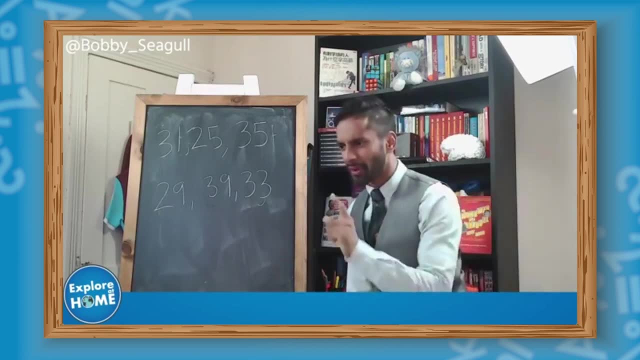 then 25,, then 35,, 29,, then 39, 33.. I have no idea what he's doing. It makes no sense. Makes no sense. Let's see if we can get what he's doing. Okay, so this one is a bit trickier. 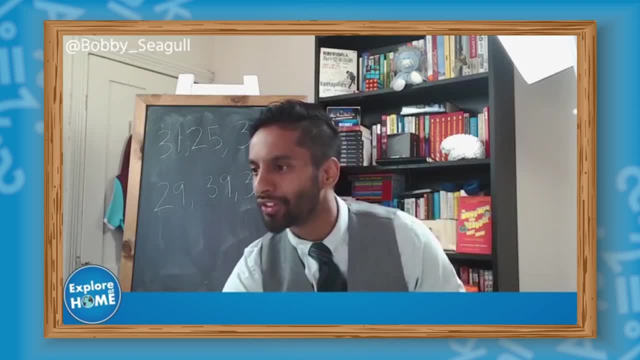 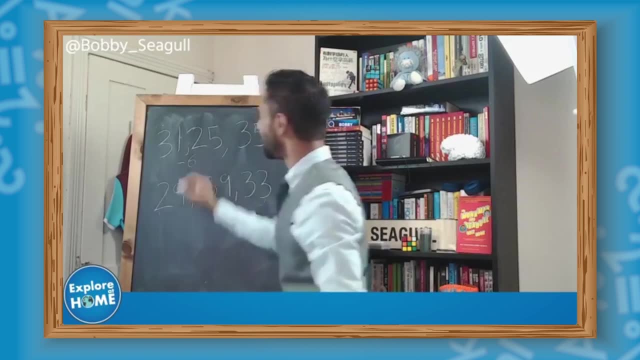 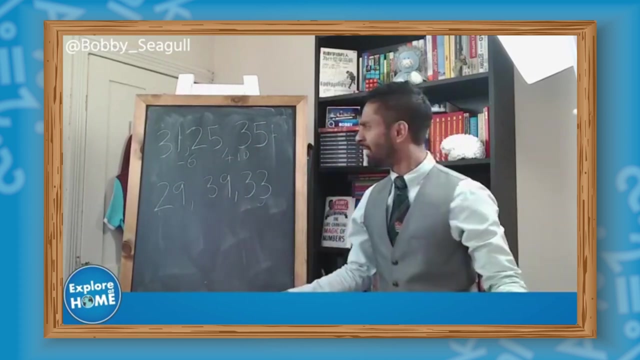 So in this particular one I'm going to see if I've got a pole on this as well. So this one here: firstly, he goes down by six. yeah, Down by six. Then he goes up by 10.. 25 to 35, okay. Then he goes down by six again, from 35 to 29.. 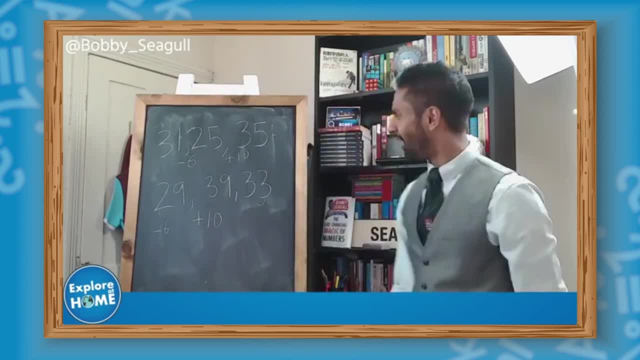 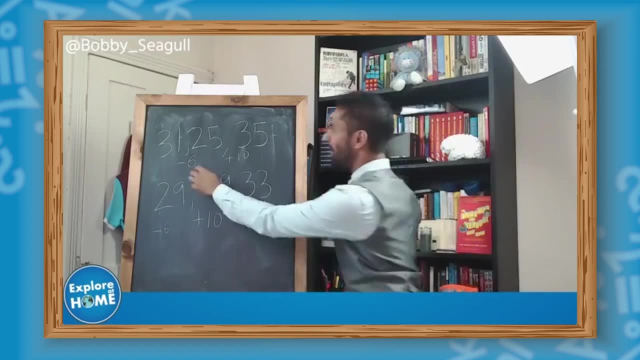 Then he goes up by 10 again. What is up with this boxer? Then he goes down by six again. So can you see, in this sequence it's strange, It's going down by six, up by 10.. Down by six. 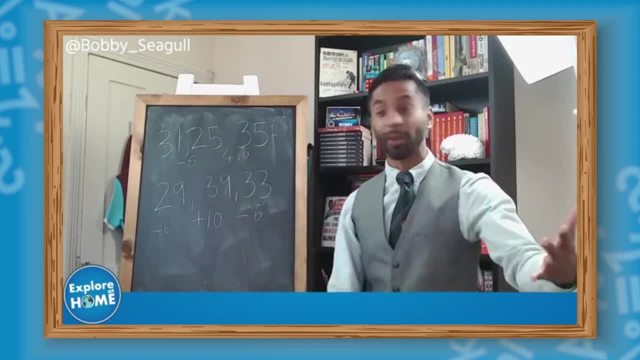 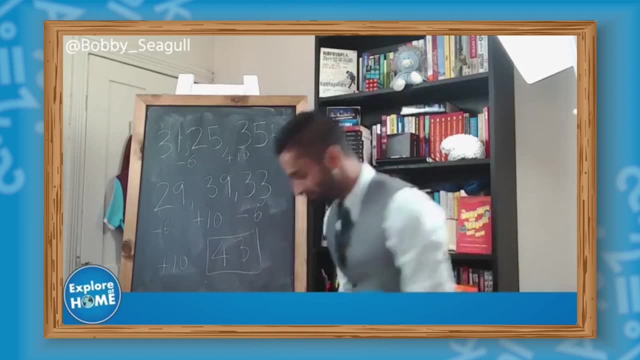 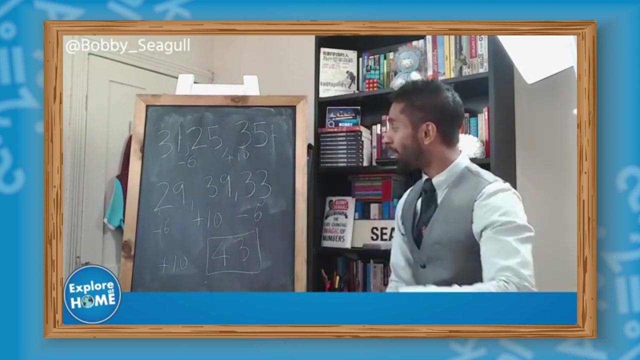 up by 10.. Down by six, Then the next one's going to be up by 10 again. It's going to be 43. That is a sneaky little boxer, Sneaky guy, Sneaky guy. So, Sam, you got it right. It goes down by six and up by 10.. So, with sequences, you've got to be very. 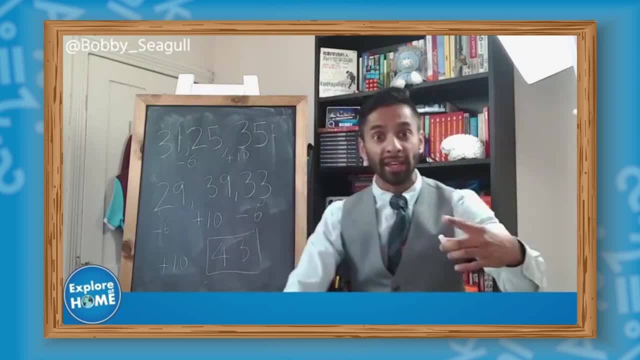 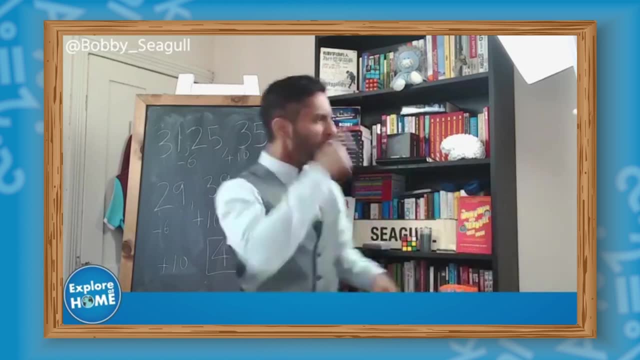 careful about thinking where it's going. Is it doubling, Is it adding a number? Is it getting smaller? Someone's saying I'm the boxer. That's true. That's true. I should tell myself off. You shouldn't trick them with boxing things. Okay, I'm really sorry. Don't trick them, because. 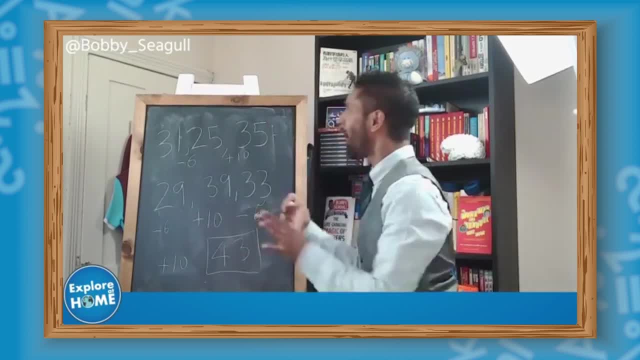 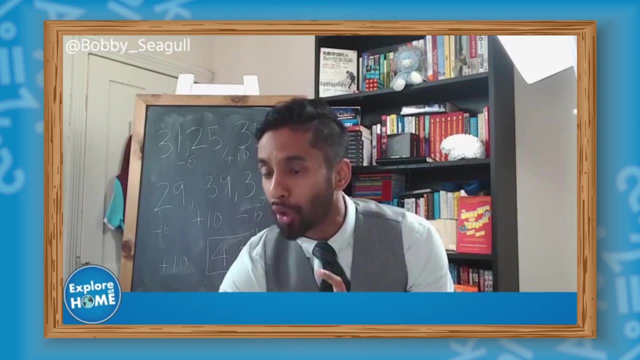 sequences are very important. You shouldn't trick them with boxing. You shouldn't trick them with important. I need to understand it. I'm sure. okay, I promise I'll be good. okay, I've told myself off, I'll be good, okay. so, uh, Allah, we're gonna do a problem on this, um, so we're gonna do a quick poll. 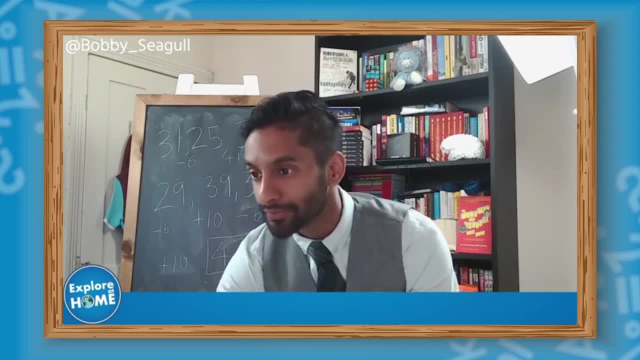 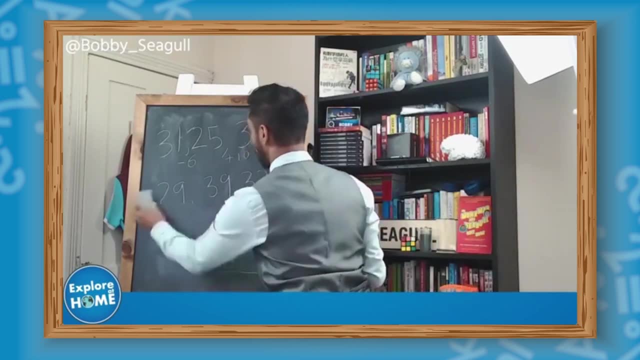 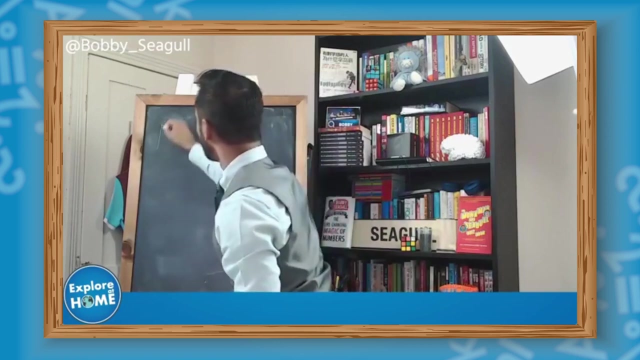 and it should be open. have a look at this. so it goes: 15 is the last one before we move on to a new topic. a new topic. I'm really excited about this topic today. so have a look at this topic. so, uh, it says 15. have a look, is it doubling, is it tripling? 15, 26. 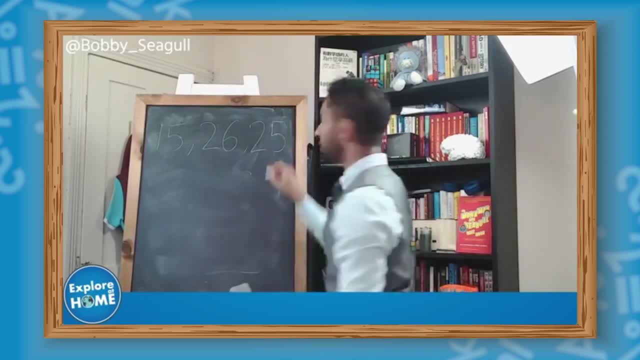 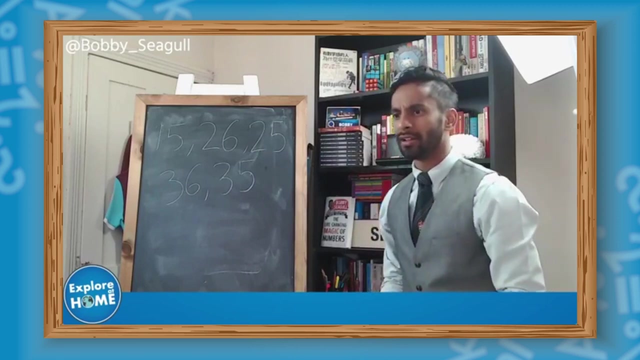 25 and I put up on the board- for those of you can't see the Facebook poll: 36, 35. so have a look at this. boys and girls, have a look at this poll. have a look at this. so Karen looks like she's on it. 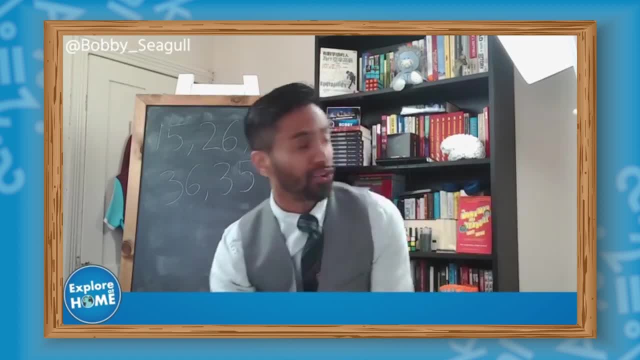 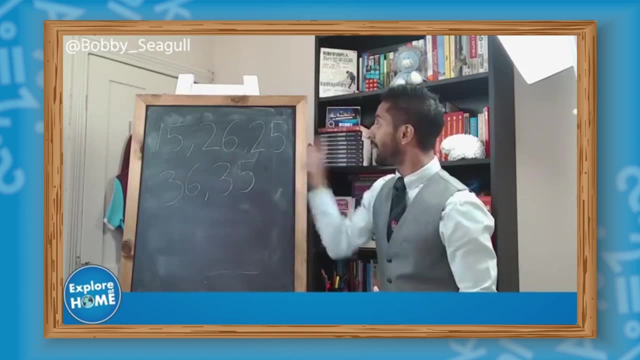 Karen looks like she's on it. let's see. is that we've got um? Shivan Gabriel Alexander, do you know what's going on? so if you can't see the poll, it's on the board here. it says 15, 26, 25, 36, 35. 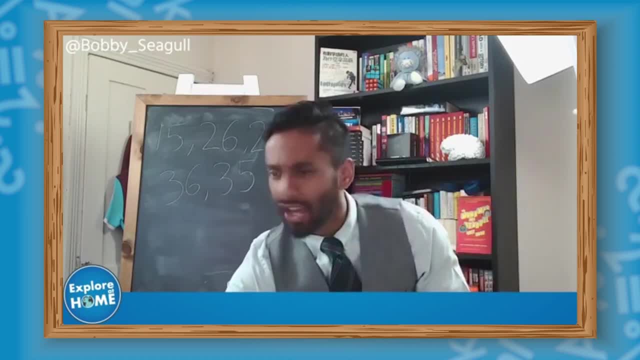 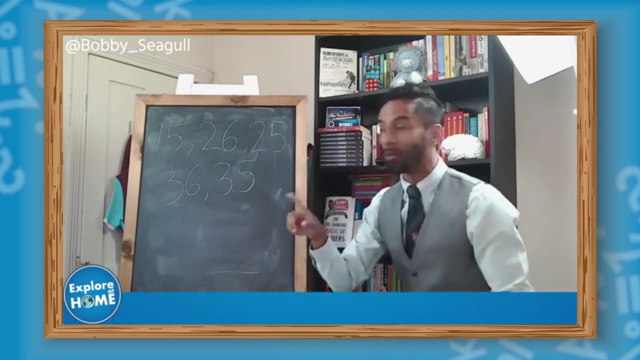 what's happening here? um, Kia and Misha, any ideas? uh, who else do we have? Hannah, welcome today. Hannah, do you have an idea? let's have a look. so I think a lot of you are on the ball here. so, Jane Black and Tony, they say what. 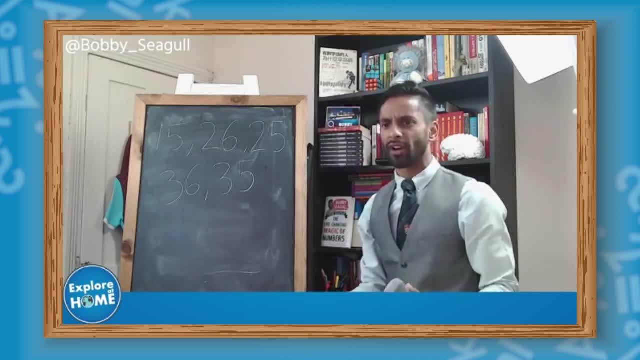 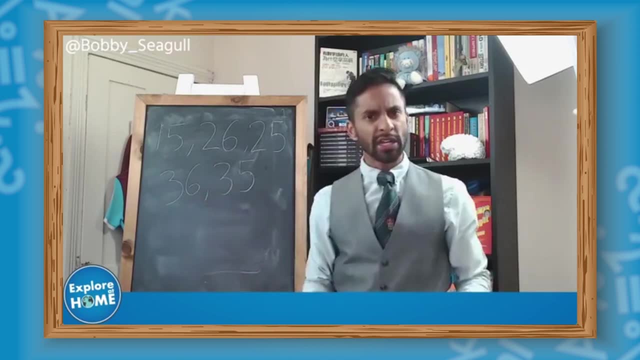 we do is you add 11 minus one. let's have a look. let's have a look, Karen Jacob's right. so you add 11, 15 to 26, then you minus one, then we add 11, then you minus one, then we add 11 again and we get 46. 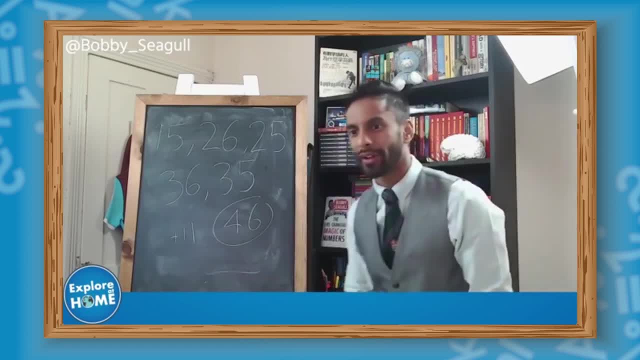 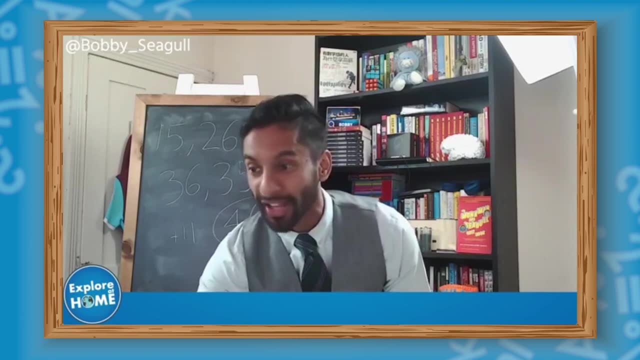 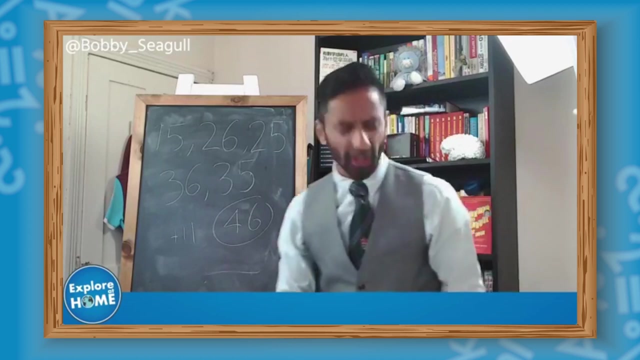 so that is the sequence for this particular one, Leah. well, well done, congratulations, that's good. I'm going to close the poll now. thank you for your contributions, everyone. Casper, well done as well. so we're adding 11.. so again with sequences. remember, we've got the boxer. the box, it's me. 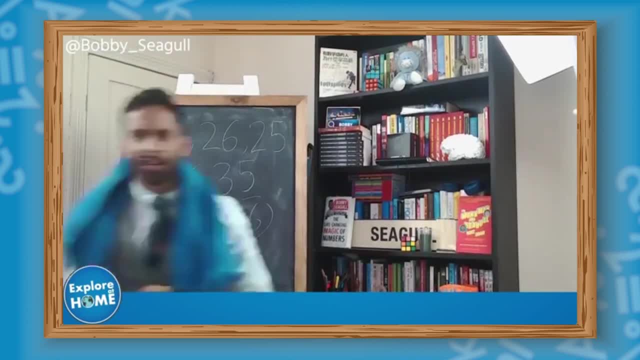 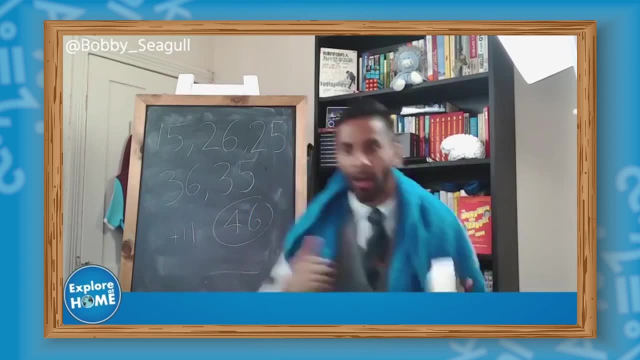 let me get my boxing pads. the key thing is be nimble, be ready to move, because the sequences could go up, could go down, could stall a bit up and down. so you've just got to be ready, Eva. you've got to be ready for all of these things, okay, okay. so now we're going to move on to the next. 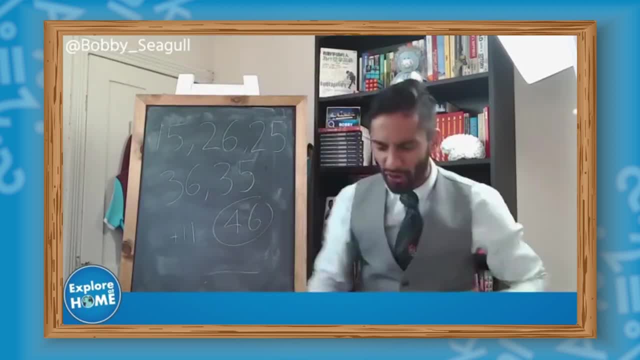 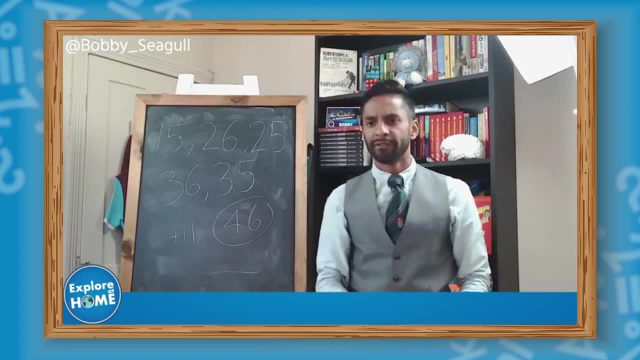 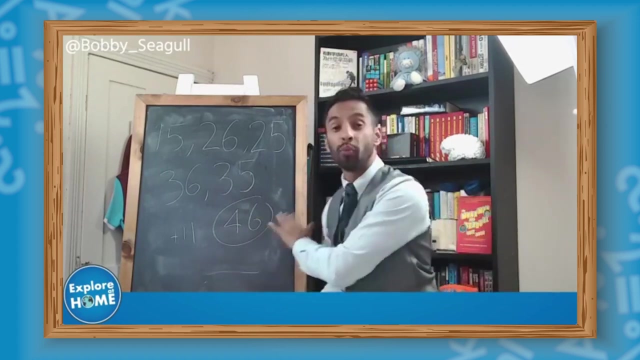 topic. I'm done with boxing for today. I'm done. it's time to now focus on something else. okay, it's half. we're about halfway, more than halfway through. so so someone said: they're not sure if you get it. if you're not sure about this, go back later on to Facebook or YouTube and watch the video. 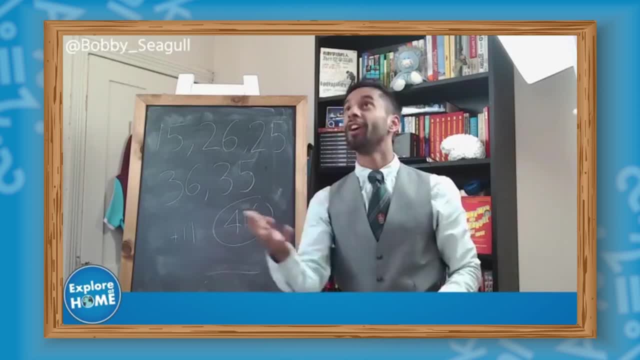 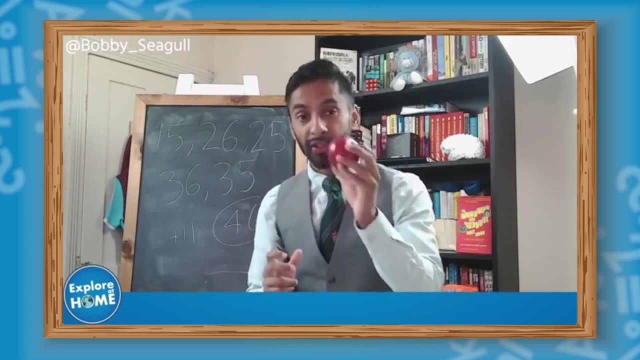 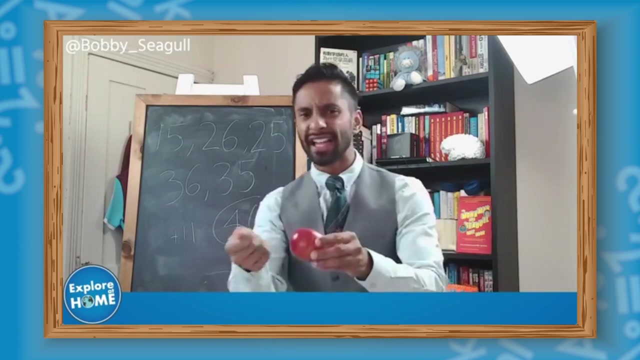 again, and that'll give you more time to catch up. so do that. so here we are, an apple. you got an apple here. am I going to eat it? yes, but not right now. so what I want you to do is: can you ever think? imagine this apple here, and I sliced. 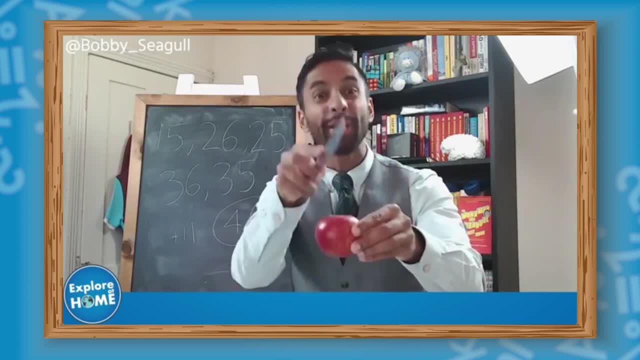 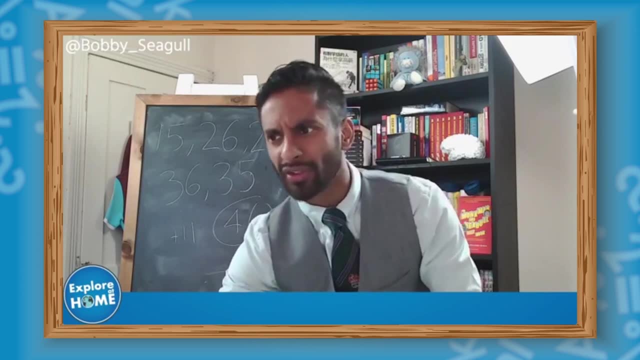 it in half, along the middle, not down. normally we cut it down vertically. imagine we cut it along the middle. what happens? so I'm going to leave this as a question for you. what do you think might happen if you cut it? what does it look like? what would the pattern be? let's have a look. 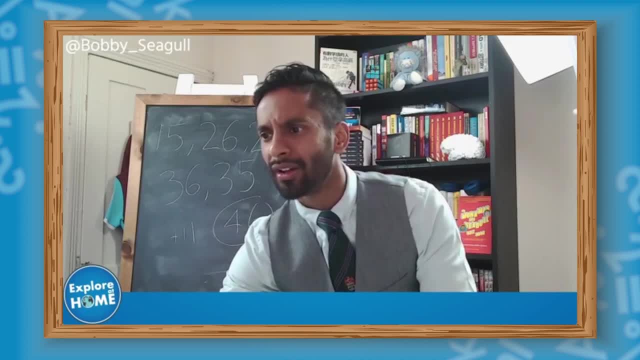 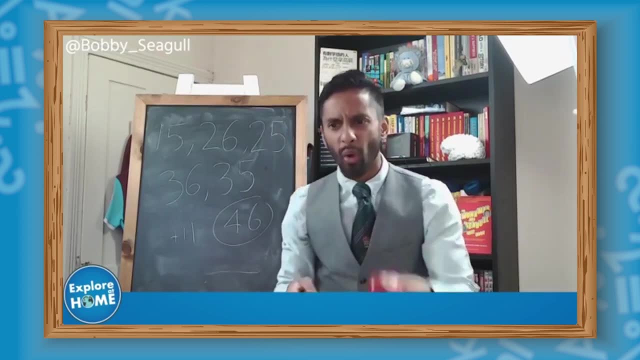 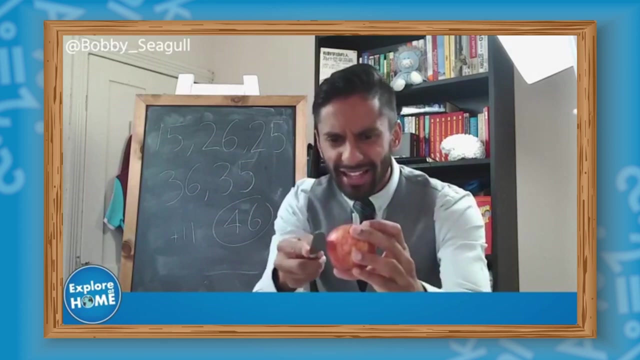 so we have- let's have a look. so we have an apple and we slice it along the middle. what do you think might happen? and the box that we lost, the box, the box are now needs to nutrition, what you're going to happen? so get the apple, slice it in half down the middle. what do you reckon normally I'd get you to draw? 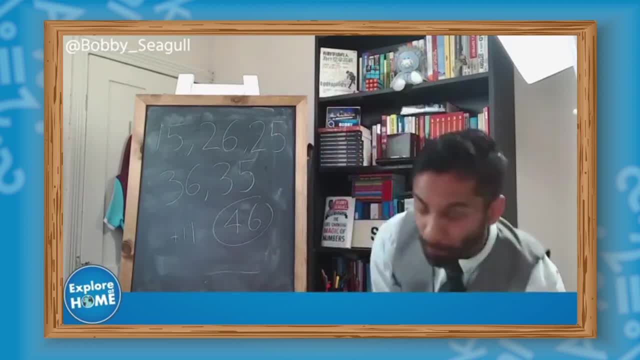 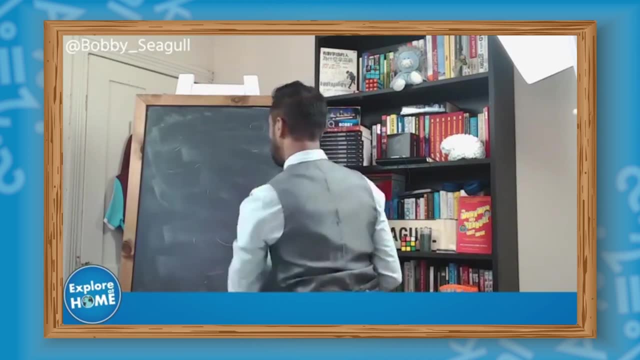 this and show me in the class. but what do you like can describe it? there's some sort of pattern going on. what do you reckon I'm going to show you now? I'm going to cut this Apple. I'm going to cut this really tasty, delicious apple. we've got this apple here. what jacket it will cut my hand. I hope not. 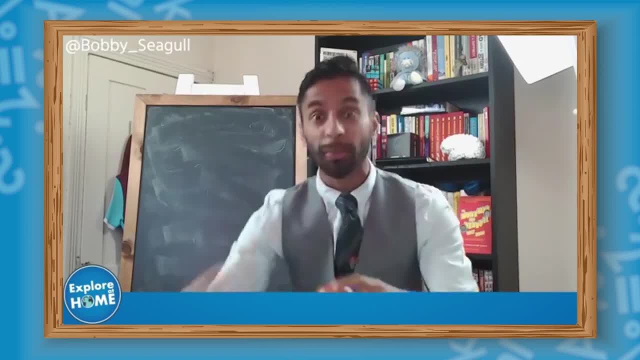 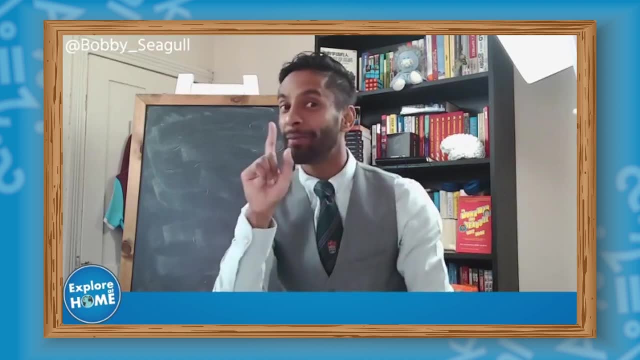 someone says two halvesmi the middle and make two halves. Leah thinks: oh, Leah's got a very smart idea. Leah says it looks like a flower. Leah might be quite close to the truth. We says a seed in each side, says Joshua. 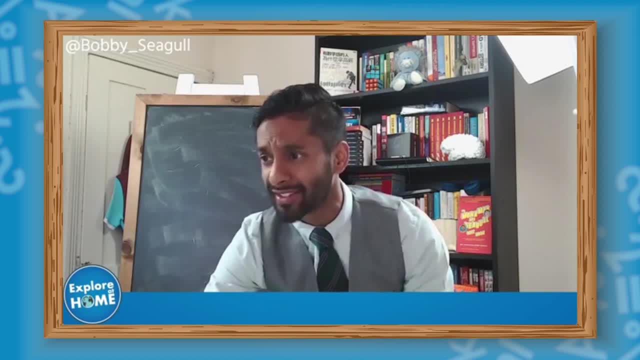 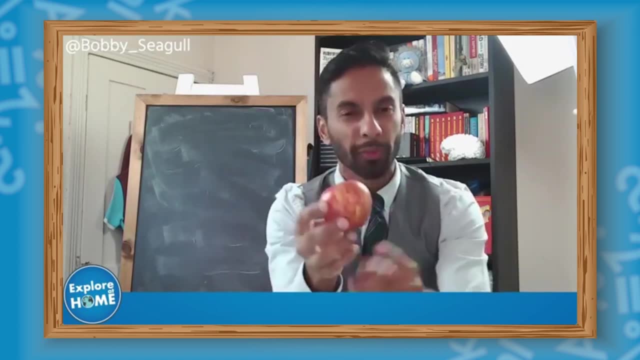 Let's see what else we have. Someone says- I think it's Samantha- says- there's a circle- Two halves. A lot of people say it's two halves, but if you split it down the middle they're two halves If you split it along the horizontal. I think Leah's idea was quite smart. So let's have 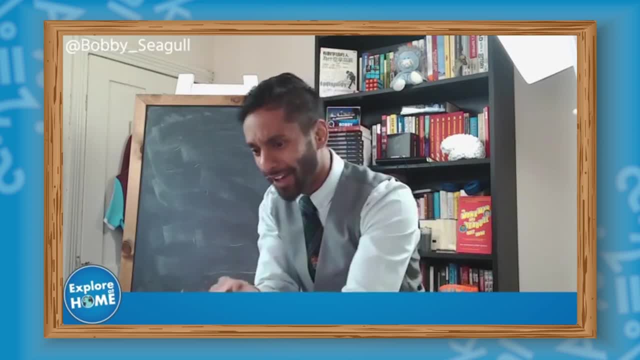 a go and let's have a look. So I'm going to slice it. I'm going to slice it and I hope this works. I haven't tried it. I haven't tried it today. I'm going to slice this apple. I am actually cutting. 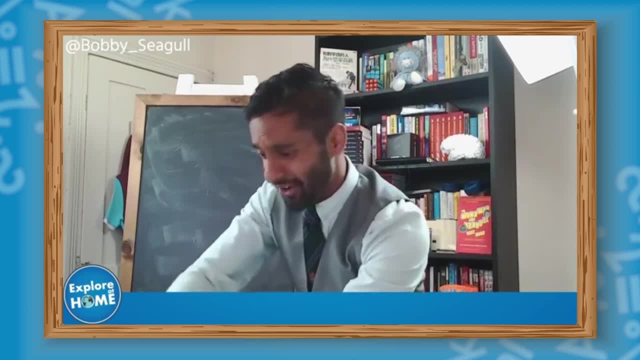 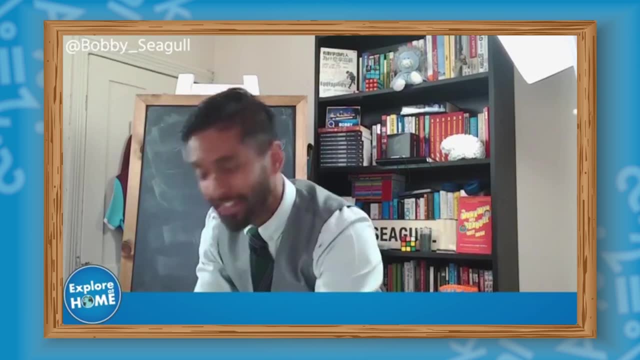 it. Hold on. I need to do more boxing training because I'm finding it difficult to slice this apple. Oh my gosh, This is really difficult And I don't want to cut my hand live on Facebook. So again I'm on Facebook, It's facebookcom: forward slash, Bobby Seagull. So if you want, 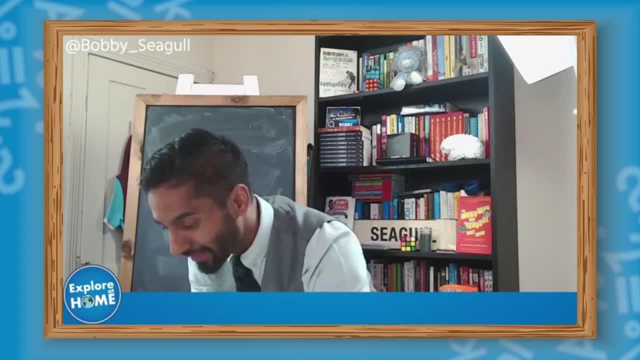 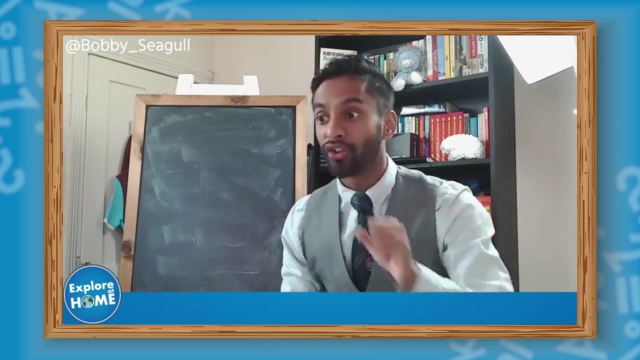 to follow me. Oh yes, I think we've got it. I think we've got it. Oh God, my hands are going to get sticky now. Okay, So I'm going to get my towel. If you look here, boys and girls- So some of you said it looks like a flower. Oh wow, Justin says a hexagon. So 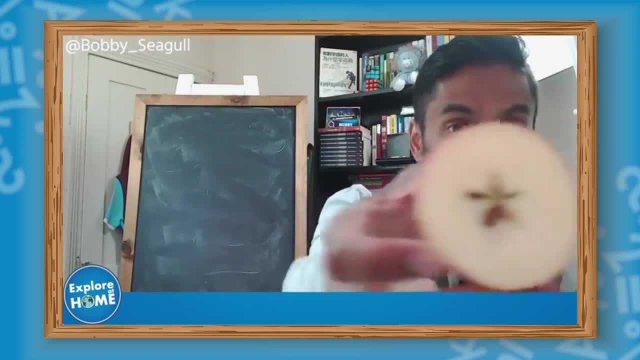 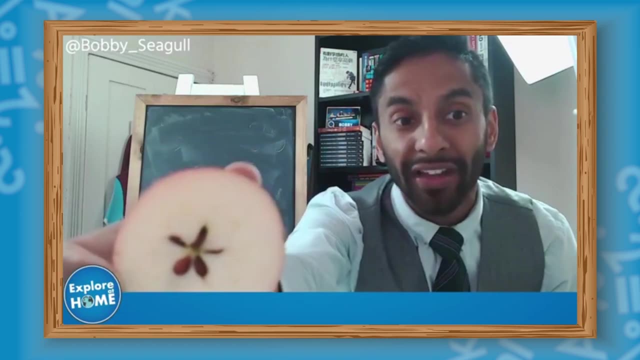 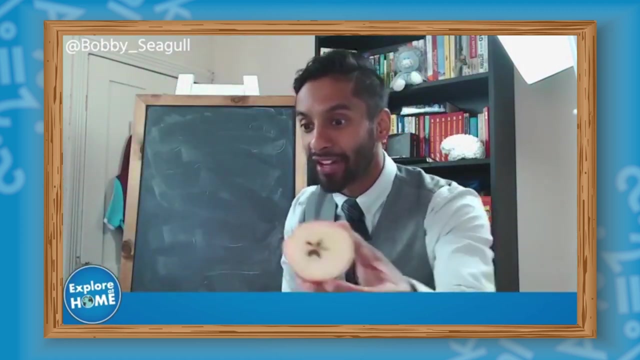 if you look here closely, can you see: there's five bits. There's five bits. Can you see one, two, three, four, five seeds. So an apple is split into five parts. That's amazing. Five parts, Five parts. Bo, did you get that? And Ismail says it looks like a star. 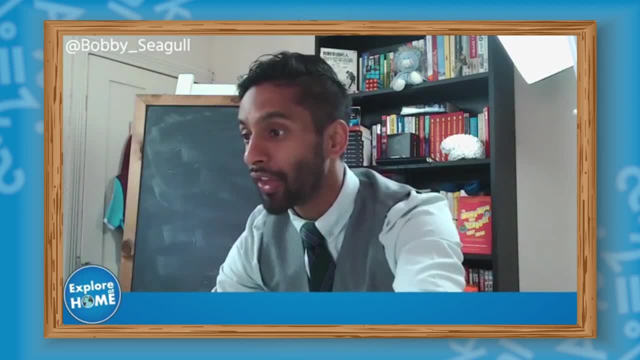 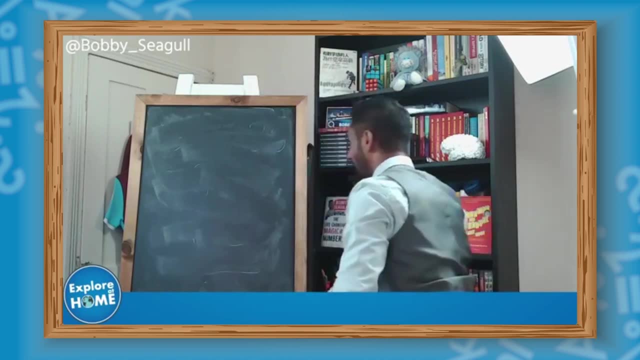 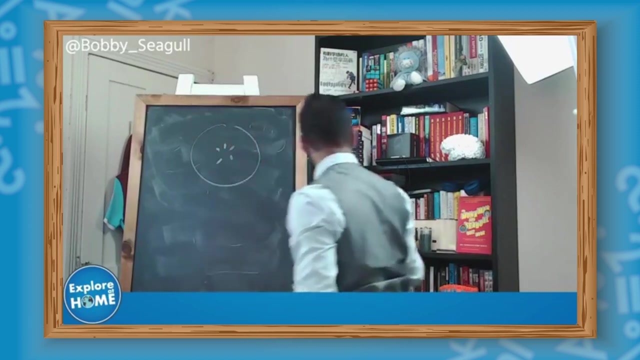 It does a little bit, doesn't it? I'm going to tell you why. So thank you so much for your contributions to the answer. So it has five seeds. Have a look at this. So the apple's there- One, two, three, four, five, Five seeds- And what you find is this five has a reason behind it. 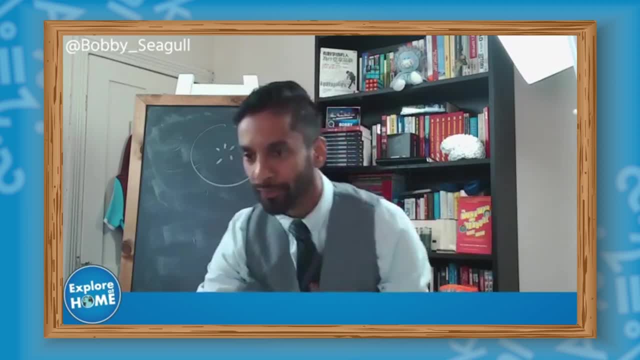 And we're going to look into why. So I'm going to get a video clip up for you. Hopefully it'll work. We're going to get a video clip up for you. Hold on, Give me a second. So the question that I want: 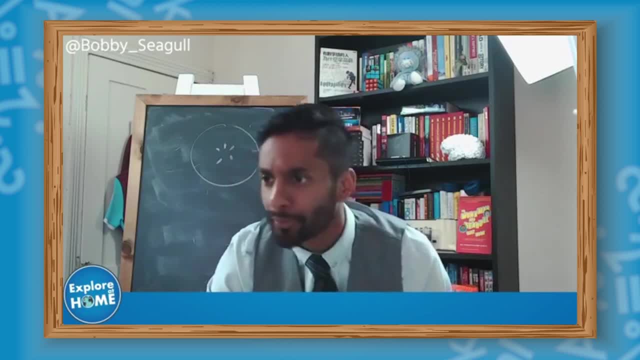 you to think about is: why is it five seeds? Why is it five seeds Like what? why? you know what's the relevance of five seeds. So let us play the clip, Hold on, Let me get it for you. So five like: why is it not four? Why is it not one? Why is it not 10?? Why is it not an even number? 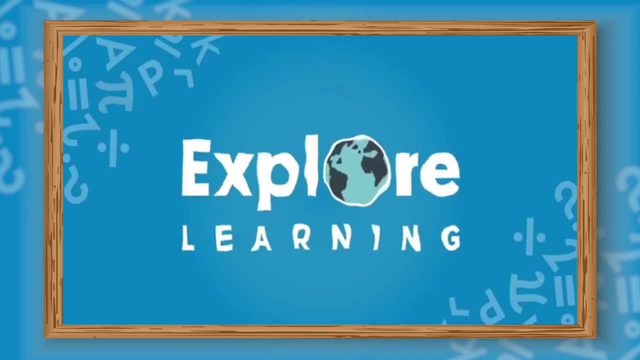 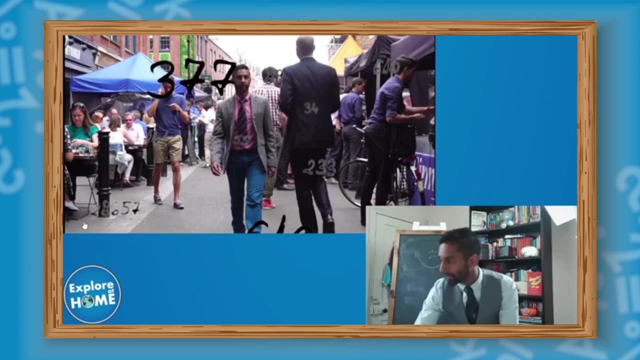 Let me get this. Here we are, So have a watch of this. That's me, Mr Seagull, And you're going to see a clip on this. Let's have a watch, So pay attention. Hopefully the sound will work. 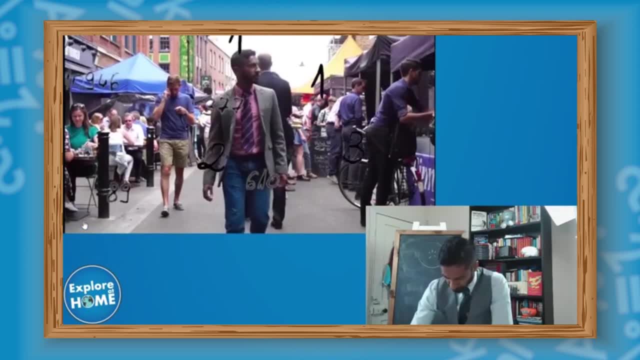 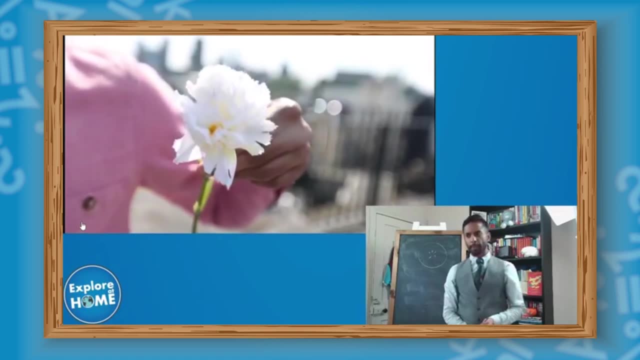 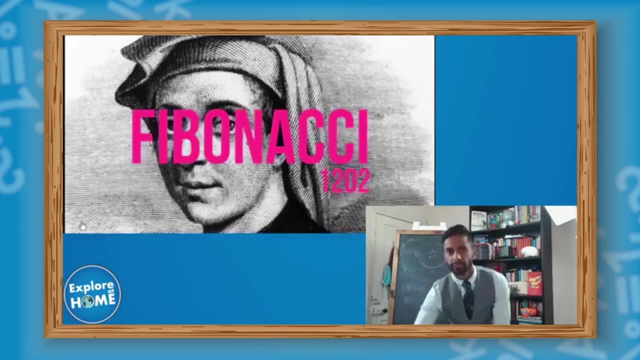 And myself. I've always searched for patterns in the world in an attempt to find logic and order within randomness and chaos. Take this flower. The number of petals in each row is the sum of the preceding two. It's called a Fibonacci sequence, Discovered in 1202 by a. 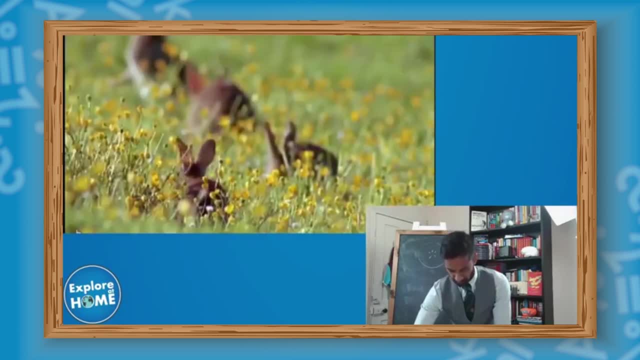 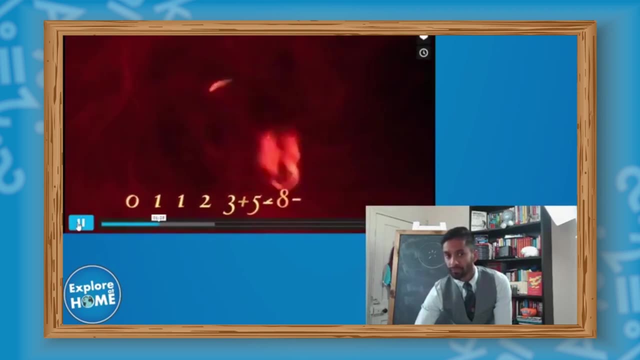 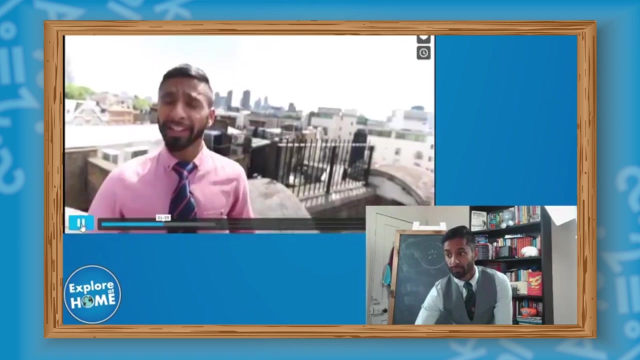 historian Leonardo Fibonacci. whilst contemplating mathematics of breeding rabbits, He noted a sequence formed through constantly adding together the previous two numbers. As the numbers get bigger and bigger, the ratio between each of the values trends to 1.618.. It's a special So. 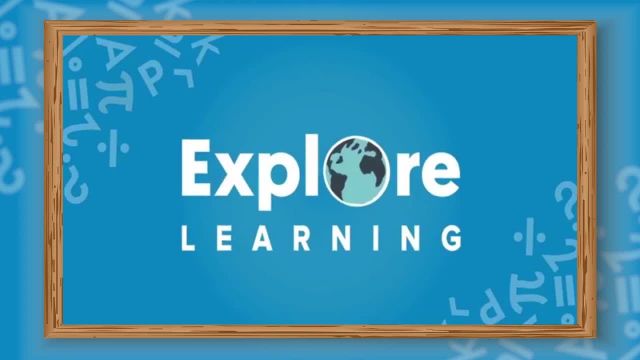 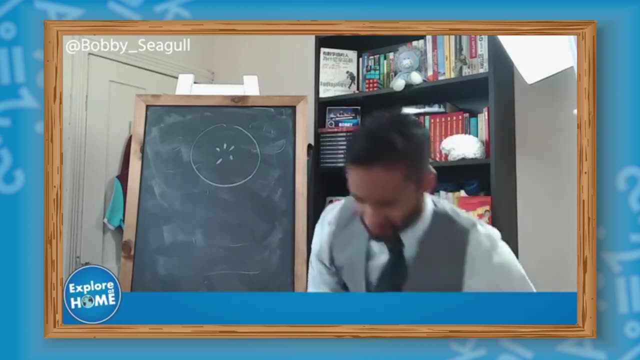 we'll go back. So you're seeing the number five crop up. So let's have a look at that sequence here. So it started off at zero. You don't have to add the zero, but it's there. Then it went one. 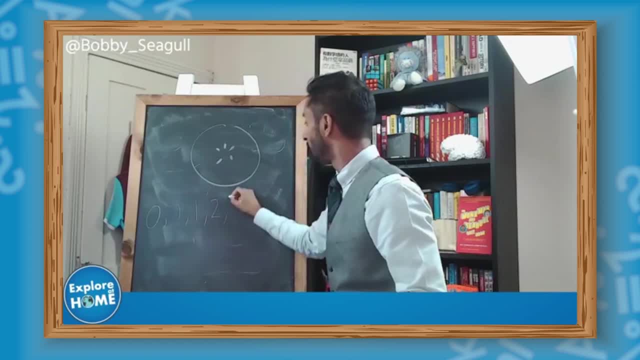 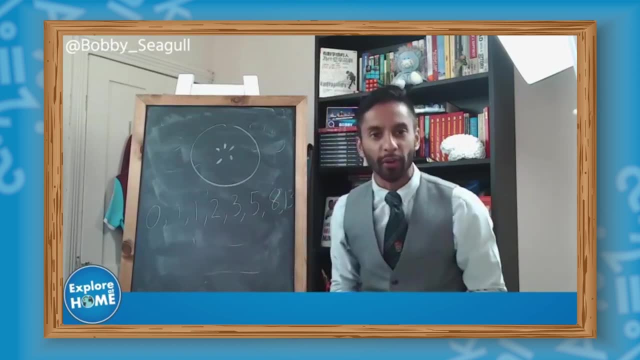 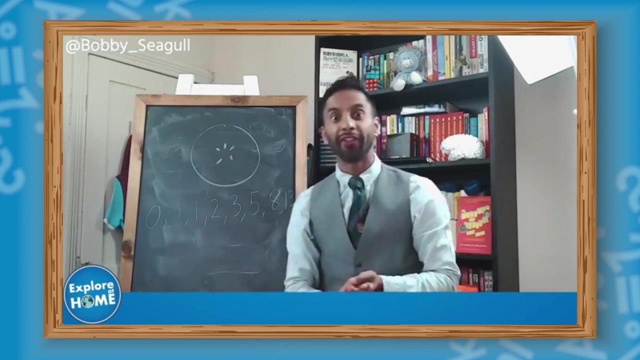 one, two, three, five and then eight and then 13.. So I can get 13 there. So can you see that sequence: Zero, one, one, two, three, five, eight, 13.. And this is called a Fibonacci sequence. 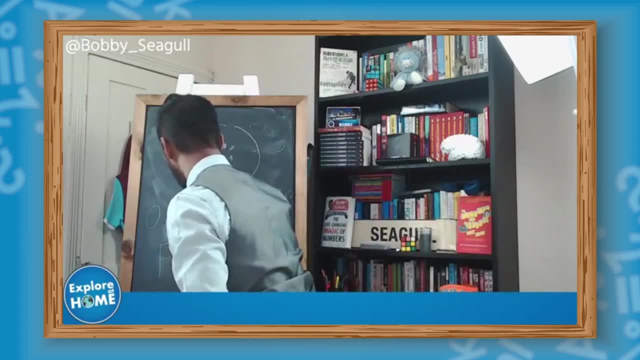 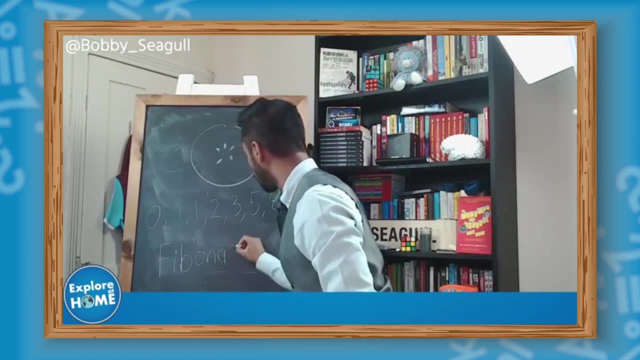 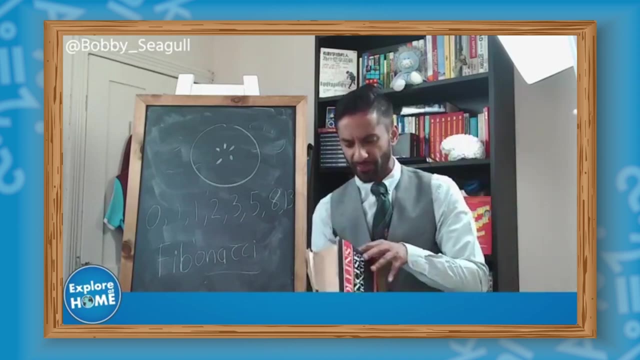 I'm going to write that for you: Fib, F-I-D, When you get the spelling correct. maths is always good in Fibonacci. Fibonacci, And this is something new, And let me consult my dictionary: Fibonacci, Let's have a look at the dictionary. What does it say in the dictionary? So, Fibonacci, if I go to F, 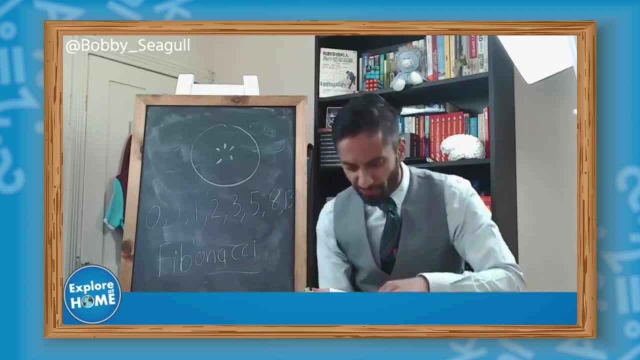 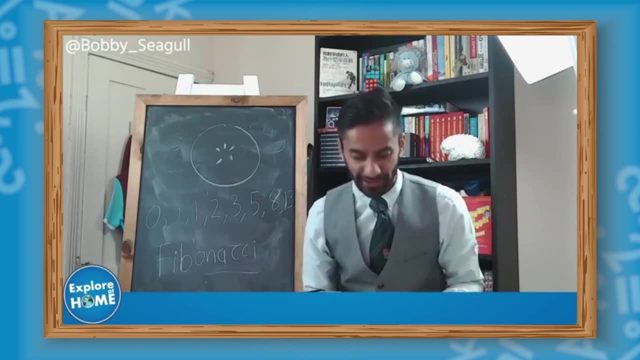 the mathematical dictionary. let me get it out. So it says here for Fibonacci. the Fibonacci sequence is one of the most famous formulas in mathematics. Each number in the sequence is the sum of the previous two That are before it. So each number in the sequence is the sum of the previous two before it. 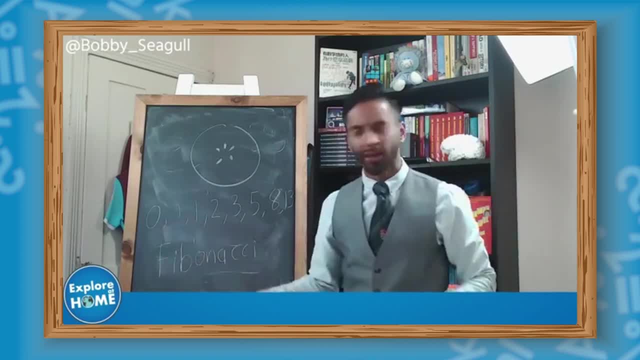 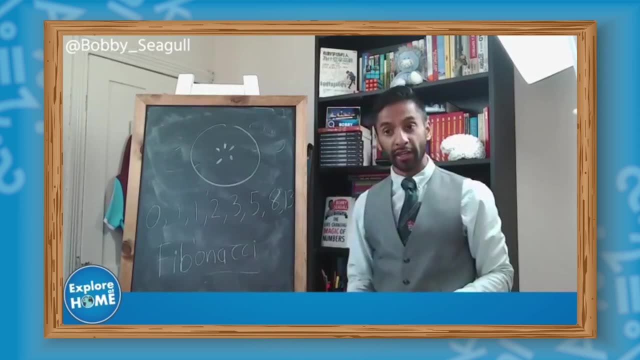 So, if you look at it, if you add zero and one, you get one. If you add one and one, you get two. If you add one and two, you get three. If you add three and five, you get eight. 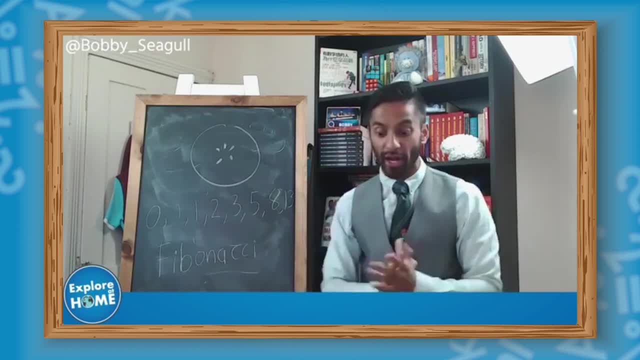 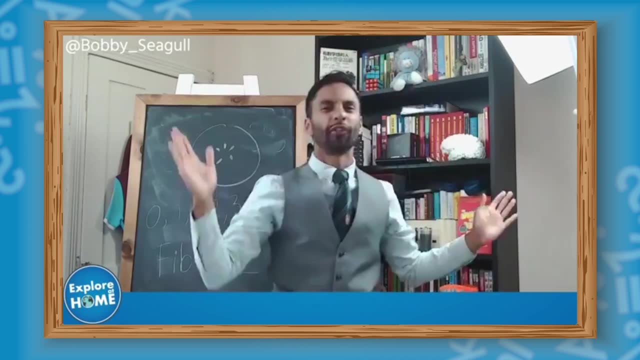 So this sequence here is called a Fibonacci And it's named after a man called Leonardo of Pisa. You know, the Leaning Tower of Pisa. It's not going to fall, hopefully, but I hope it doesn't. The Leaning Tower of Pisa, he's from there in Italy about 1200 years. 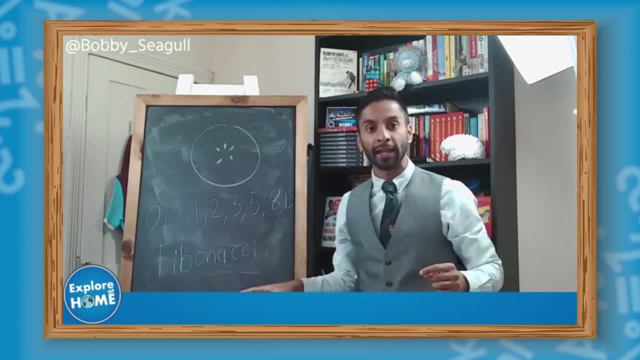 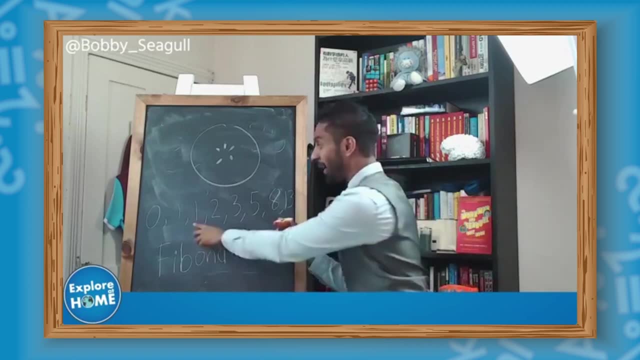 so about 820 years ago, And he came up with this pattern And he noticed that this pattern was everywhere in nature And the way nature grows is actually grows in this particular pattern. Things will have one leaf, then another leaf, then two, then three, then five. 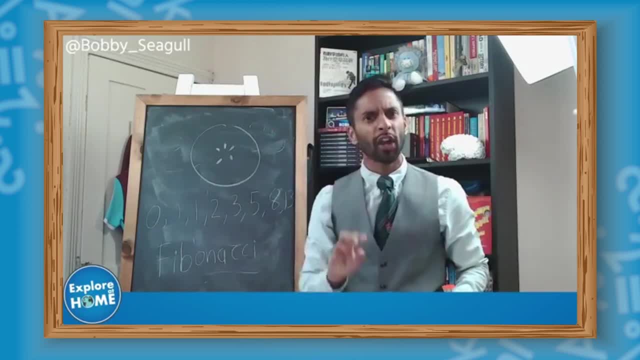 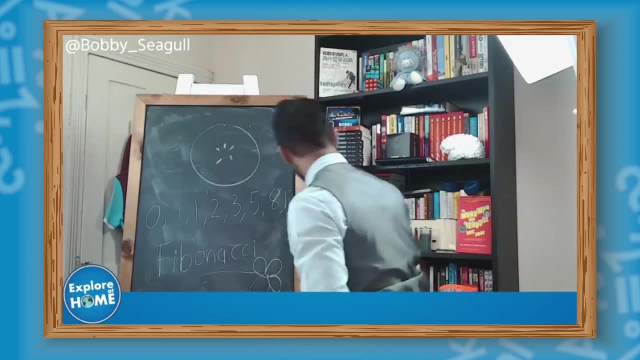 And if you think about it, have you ever seen a four-leafed clover? A four-leafed clover, They do exist, but they're rare, A four-leafed clover, And the reason is often things will go up in one, one, two, three, five. 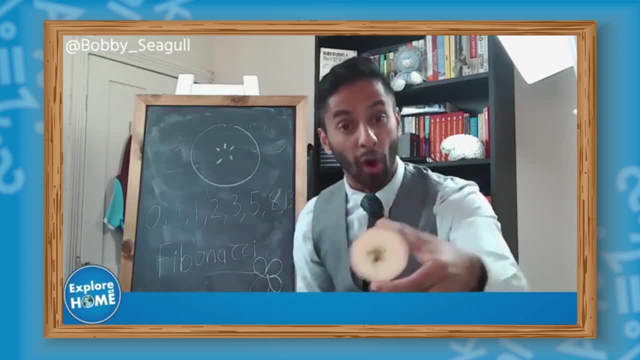 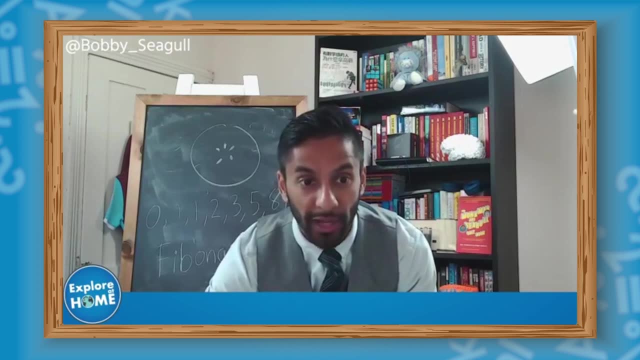 And we had the apple here and we saw the five. It exists because of the Fibonacci sequence And I'm going to show you. I'm going to carry on this clip for you. I'm going to carry on this clip for you. 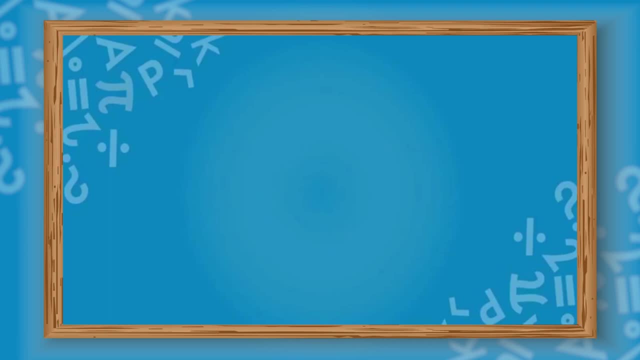 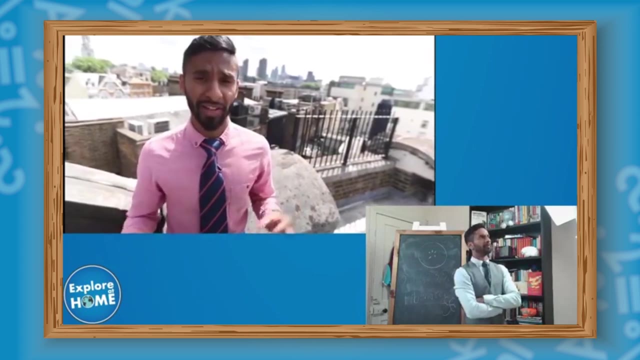 Let's have a look. I'm going to carry on, So I want to show you where this goes. And this is quite magical. This is a special number that, since the beginning of time, has been hidden in plain sight All around us, Embedded in nature and fundamental to life itself. 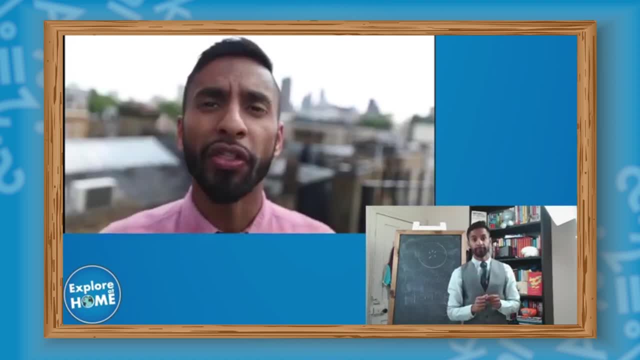 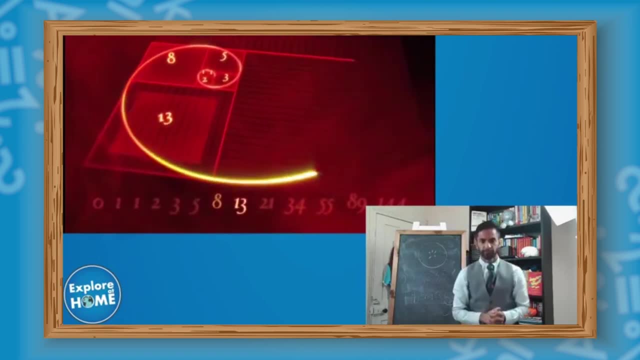 The Greeks knew of this number and had a name for it. They called it the golden ratio. Picturing a curve, a golden spiral, if you will, growing at a constant rate of 1.618 every turn, suddenly reveals a startling influence in the world around us. 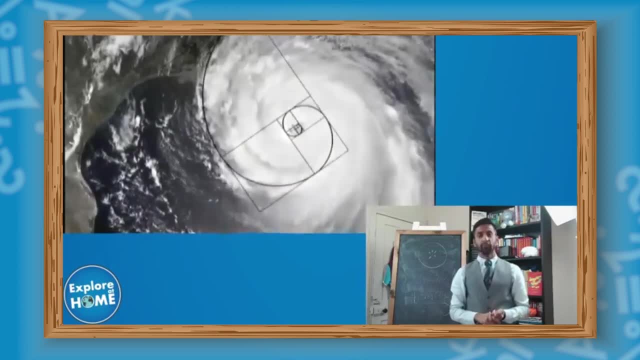 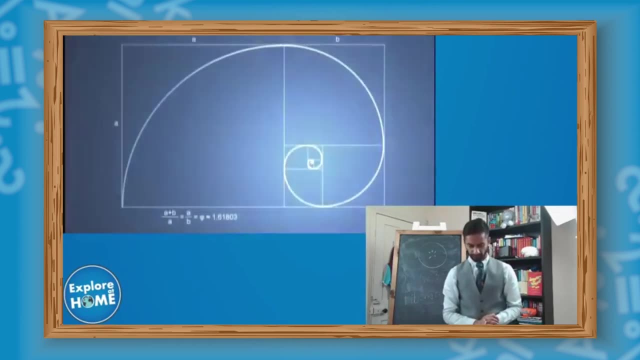 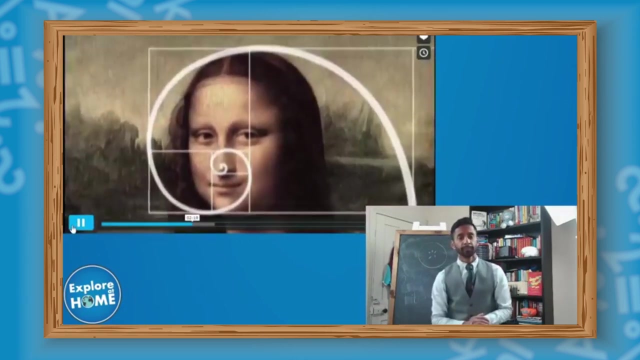 From how a nautilus shell grows to the destructive power of a hurricane or the movement. The golden ratio is even found in ancient structures, as humans harnessed its power for the purpose of beauty, From famous works of art to the corporate logos and symbols that dominate our lives. 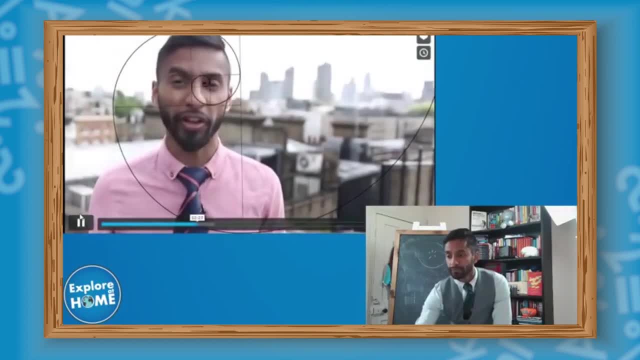 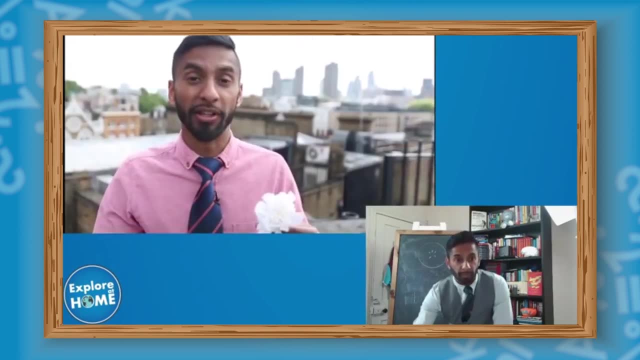 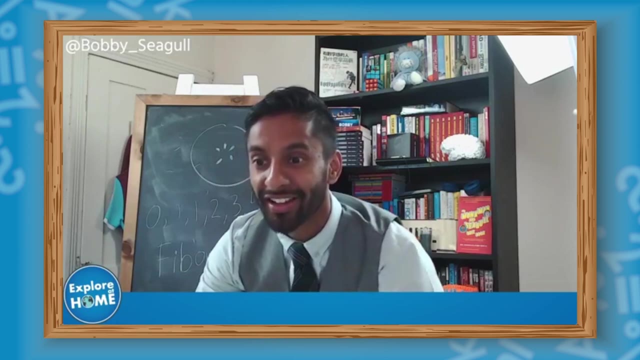 I'm even talking to you right now in the golden ratio, all based on a number you can find in a flower. Now, isn't that just incredible? So, boys and girls, I think that's remarkable, isn't it? I think that's remarkable. 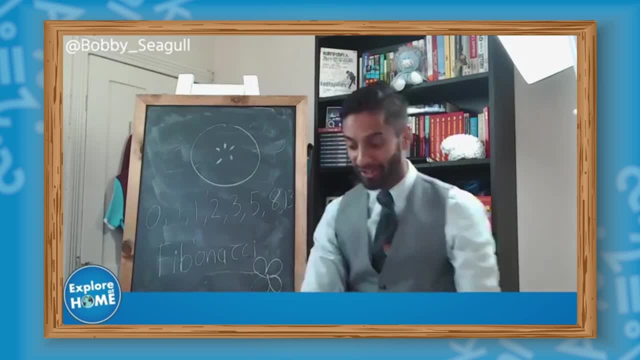 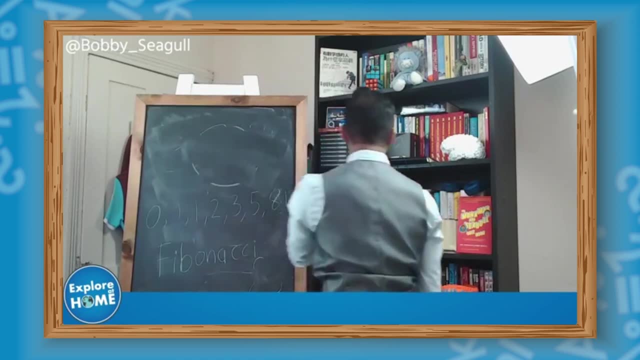 Can you see that? The golden ratio? And this is all to do with Fibonacci. So Fibonacci is a new thing. Again, when you look at an apple, you would think it might have four or two in an even number of pips. 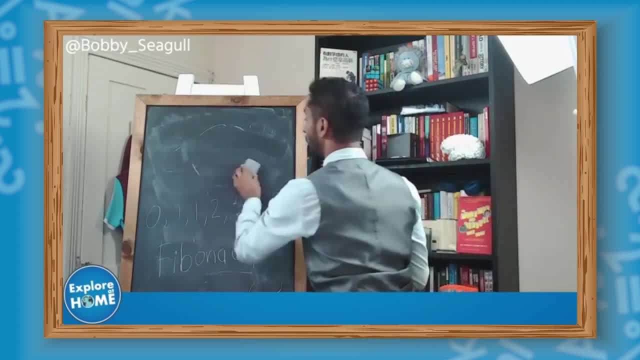 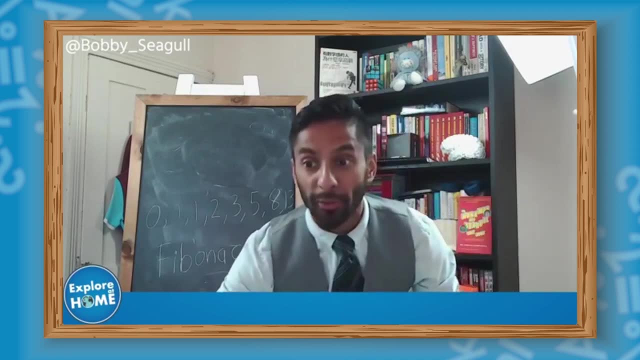 But it has five. because of Fibonacci And that Fibonacci sequence, we can see it throughout the world. Again, remember in that clip it talked about a few things. Let's see if it's here. So we can see it in sunflower seeds. 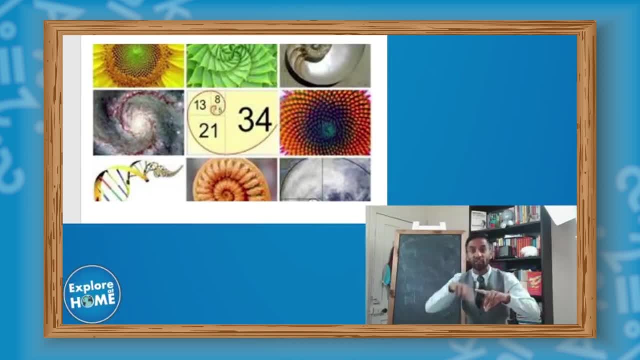 You can see it in cauliflowers, You can see it in shells, You can see it in the spiral of the universe, You can see it in DNA. And someone's asking me, Raj, what is the golden ratio? And that's a really great question. 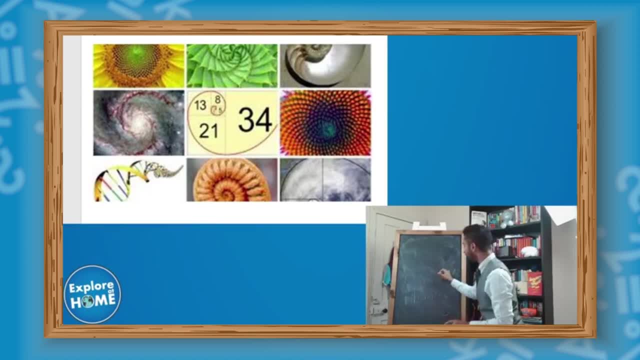 So you know what the golden ratio is. If you divide the number, let's say 3 divided by 2.. So do 3 divided by 2., You get 1.5.. If you do 5 divided by 3,. 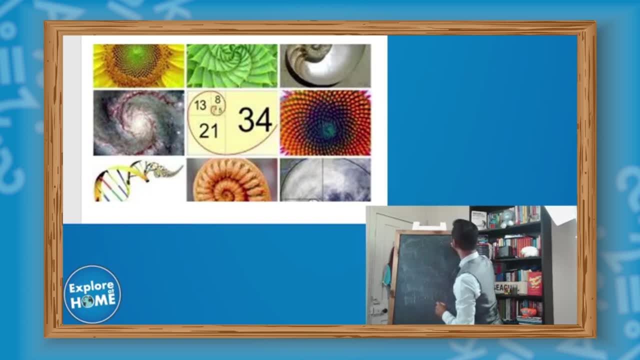 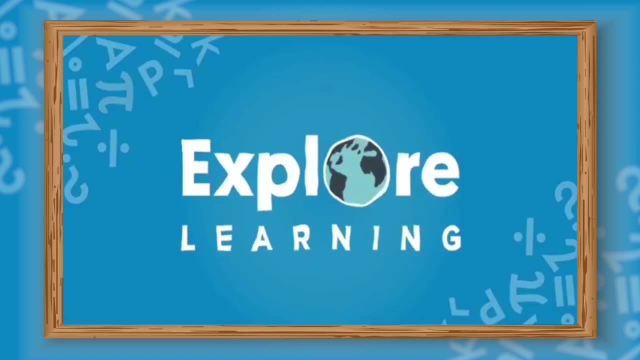 you get 1.67.. If you do 8 divided by 5, you get 1.6.. What happens is: what happens is as we get. so what happens is as we get larger with the sequence here. so you have the Fibonacci sequence. 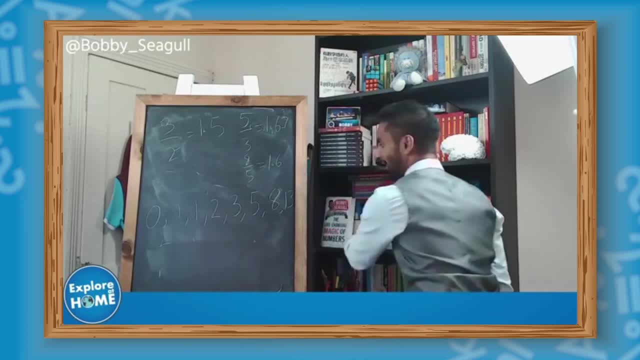 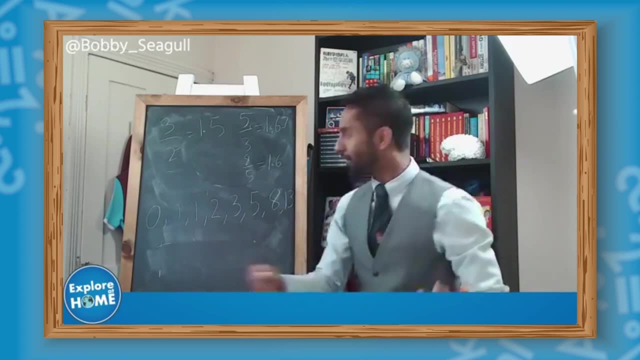 Again, this is amazing, boys and girls. This is the power of mathematics. So we have 5, then 8,, then 13.. What's the next number After 13,? it's 13 plus 8 is 21.. 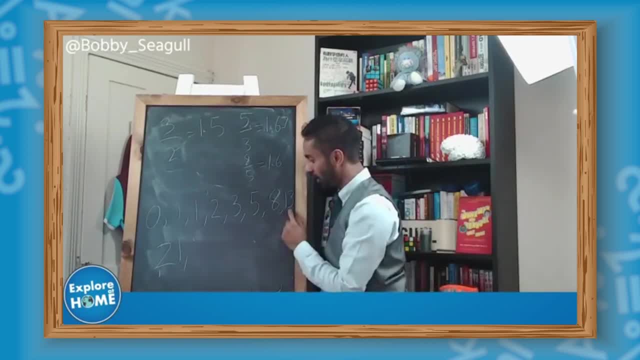 Then, after 21,. again, you add the two numbers next to it. 13 plus 21 is 34.. If we keep dividing the numbers next to each other, we get a number that's called the golden ratio, And Edward says he knows this. It's amazing, isn't it, though? 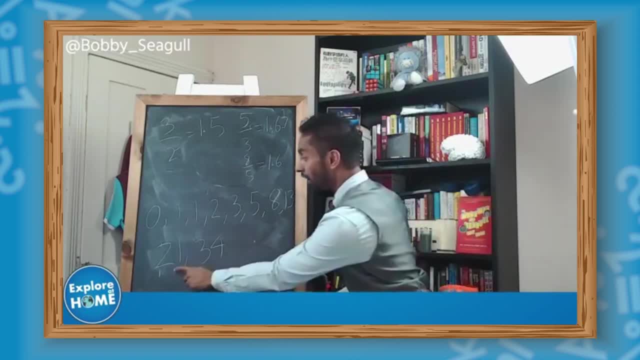 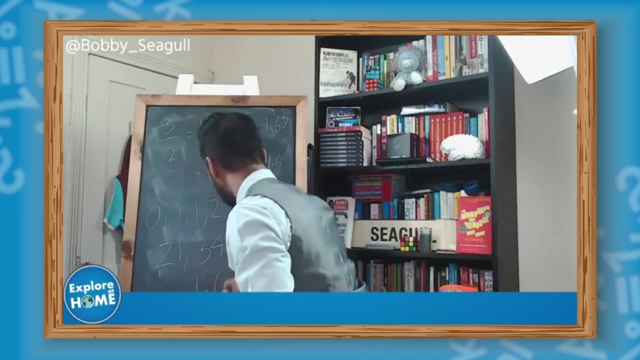 The golden ratio. Even in our DNA, we see there are 21 and 34 strands of a particular DNA, And Sarah Ling says it's about 1.618.. 1.618.. So this golden ratio exists everywhere in nature And it's amazing. 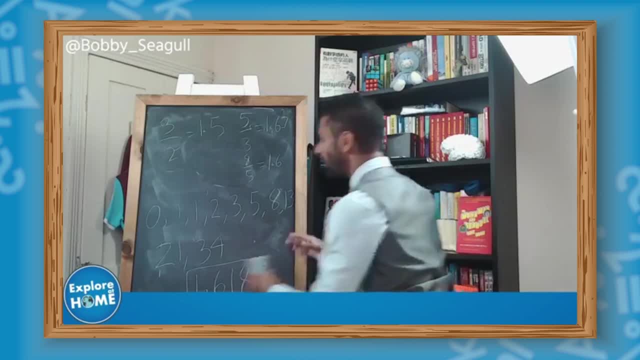 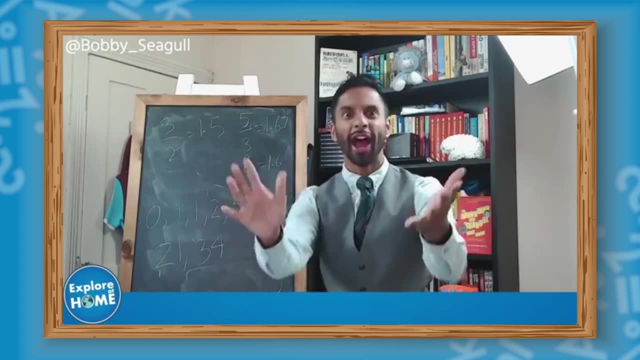 And there are some mathematicians that say, oh, but you know, we're just finding a pattern that doesn't really exist, But it's amazing. For example, we have two knuckles, or two hands, five fingers. These numbers here, 1, 1,, 2,, 3,, 5,, 8,, 13,. 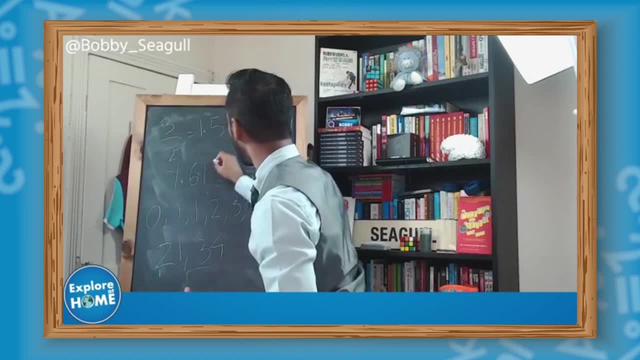 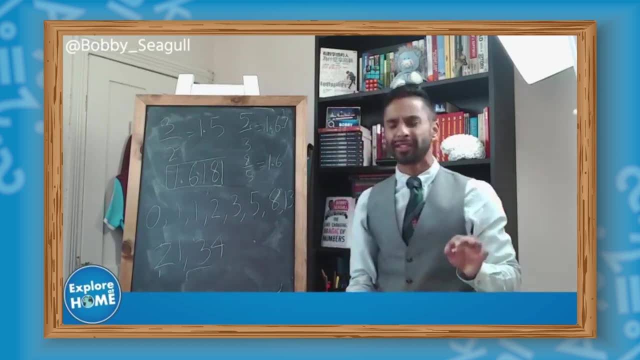 exist everywhere. So it's at 1.618.. And that is called the golden ratio. And this is a beautiful sequence, Beautiful sequence. So Phoebe says she doesn't get it. So let's just recap. Let's recap where we are. 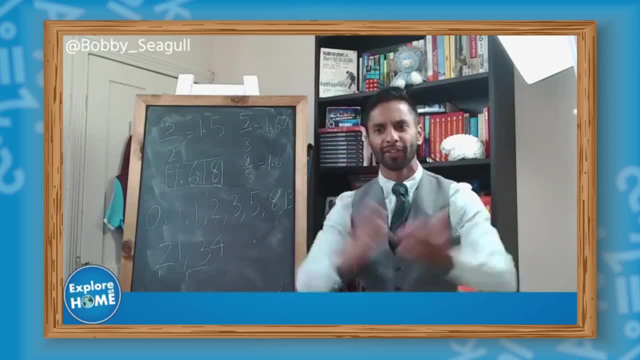 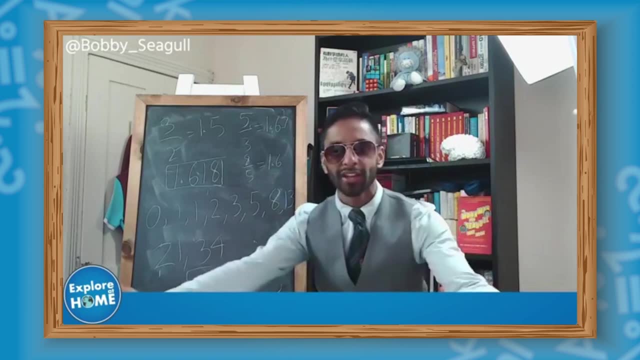 I'm going to do a quick rap about this, Of course. A quick rap, So a quick rap, So quick. glasses, Glasses, glasses, glasses, glasses. Time for the rap. Okay, The rap is 1, 1,, 2,, 3.. 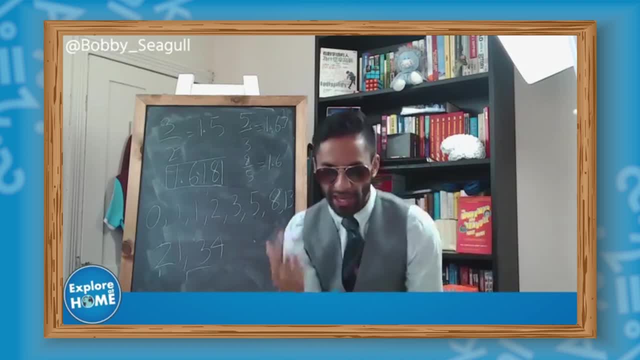 That starts Fibonacci 5,, 8,, 13.. Sequences to be seen. Let's do that again: 1, 1,, 2, 3.. That starts Fibonacci 5,, 8,, 13.. Sequences to be seen. 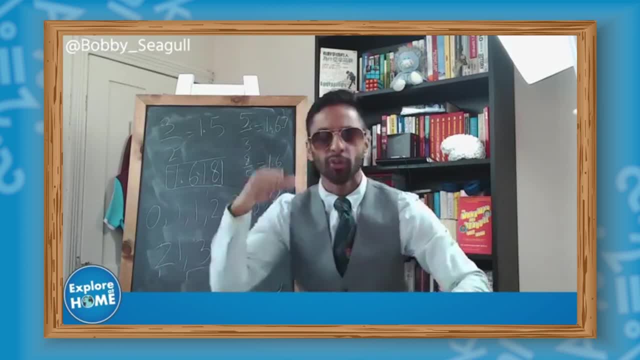 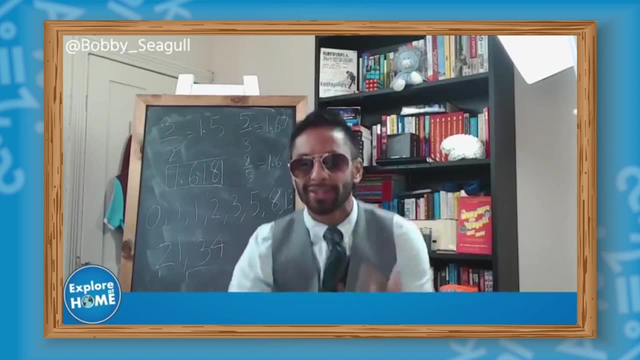 Let's do that one more time. And then Irene is going to explain the sequence again. It goes 1, 1,, 2, 3.. That starts Fibonacci 5, 8, 13.. Sequences to be seen. 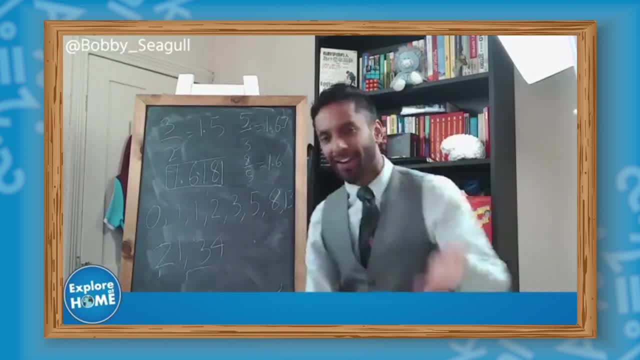 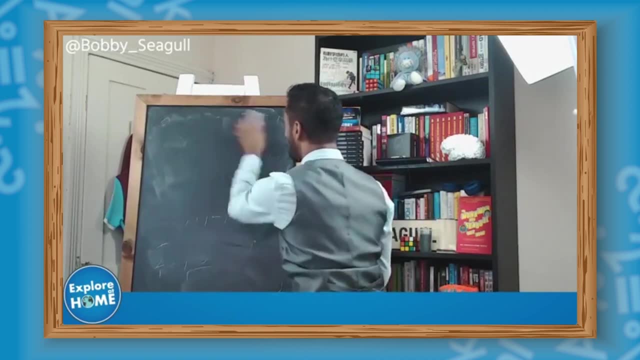 So let's get Bobby back. Let's get Bobby back. The rap has to go. So if you look at the sequence, I'll look at it properly again, because this is totally new. We've done sequences this morning with a boxer going up down. 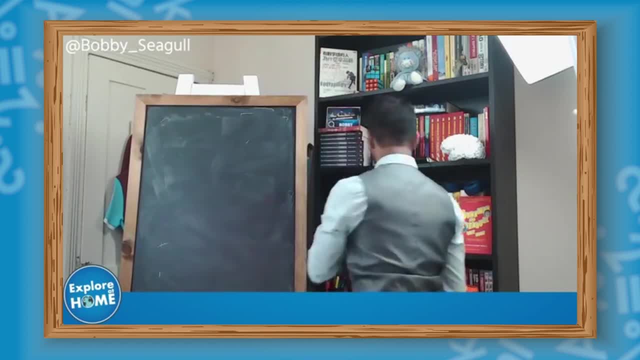 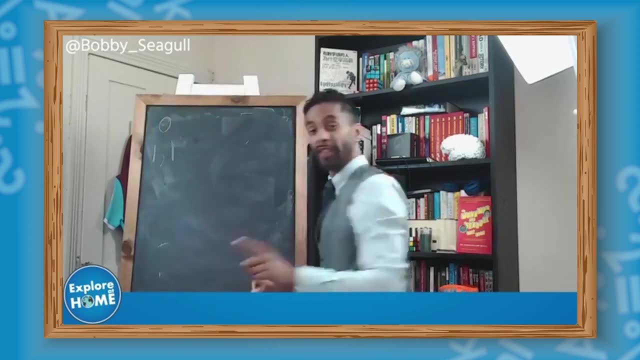 adding numbers, multiplying. But now let's look at this sequence Again. you often start with 0.. We'll put 1 there, So you get 1, then 1.. And then what we do, Irene, is. 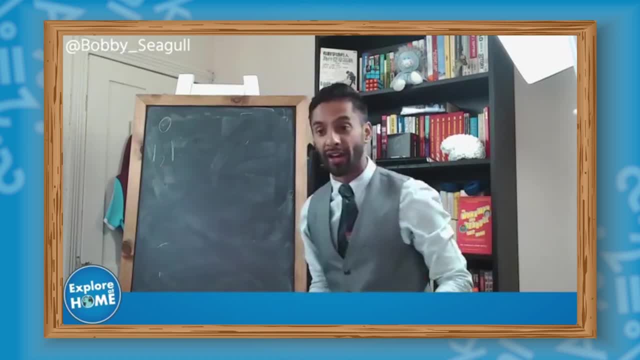 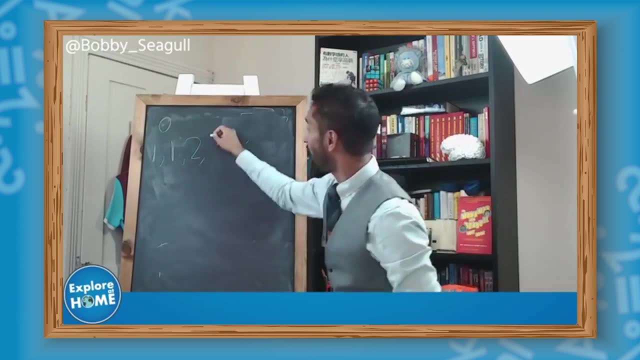 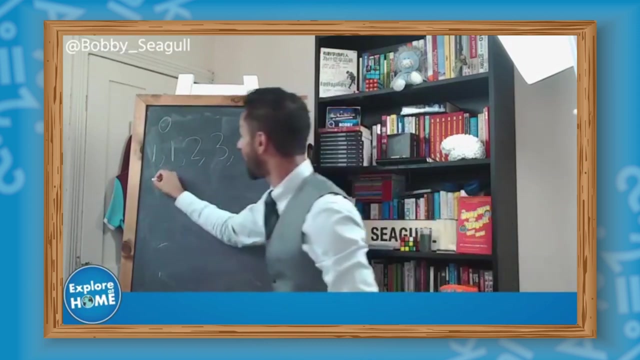 as you can see, that we add the two numbers together and we get 2.. Then we add those two numbers, Irene, Then you get 3.. Then we add those two together, 2 and 3,, you get 5.. 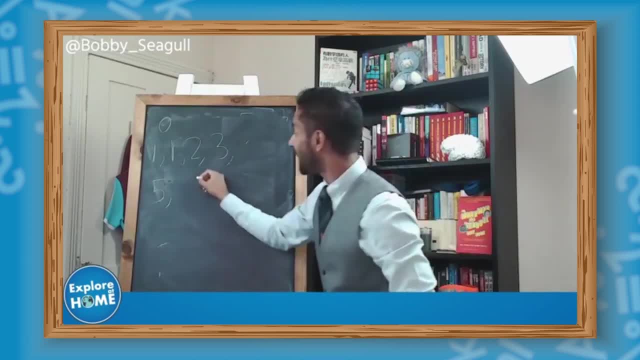 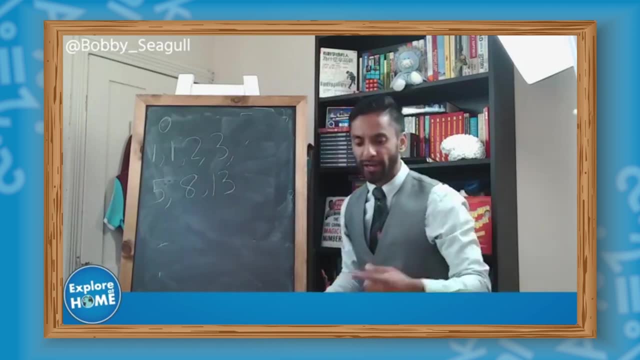 Then we add 3 and 5 together and we get 8.. And then we add 5 and 8, we get 13,. Zap, So when I think someone was asking me what happens. So again my rap was: 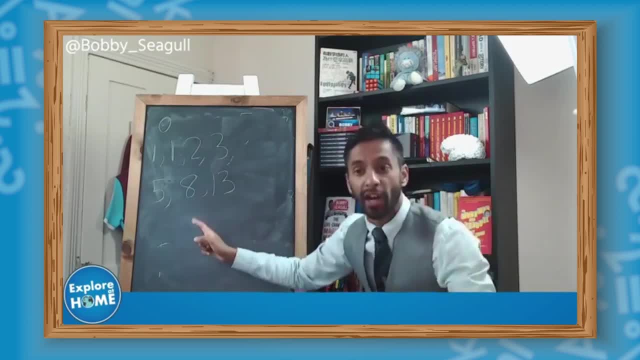 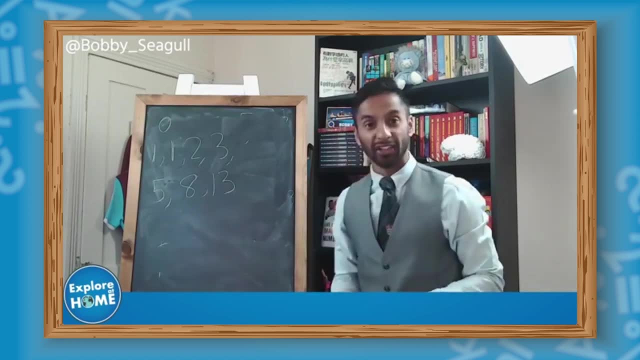 1,, 1,, 2,, 3.. That starts Fibonacci. 5,, 8,, 13.. Sequences to be seen. So you keep adding up the numbers next to each other. And the beautiful thing mathematically. 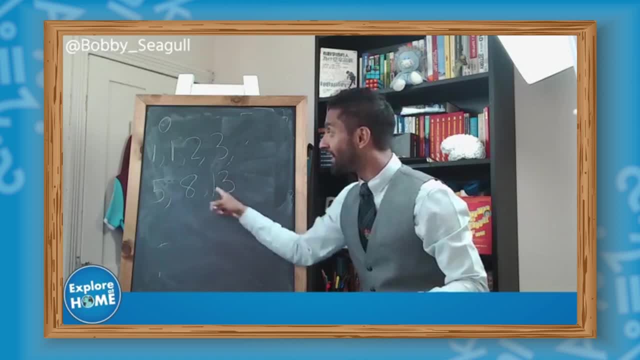 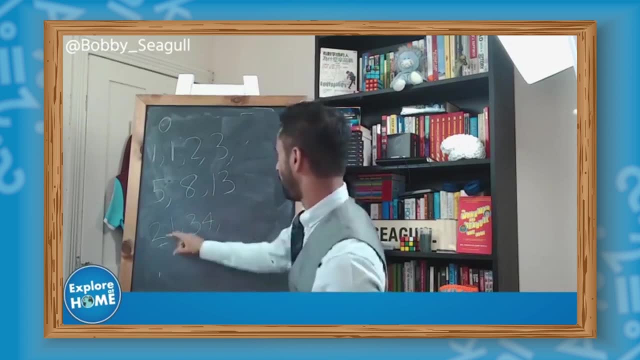 was that when you divide the numbers next to each other as the numbers get bigger and bigger- for example, you go 21,, 34.. And you can do this for me: 55, it keeps. Is that correct? Yeah? 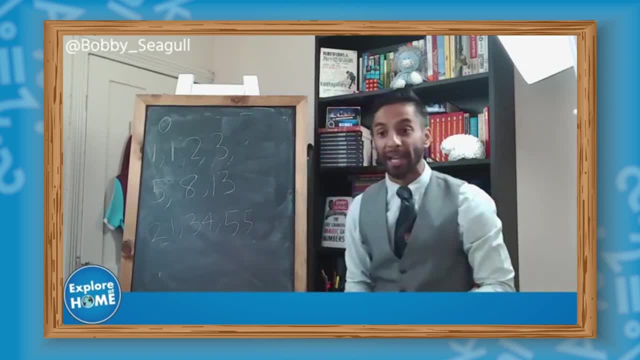 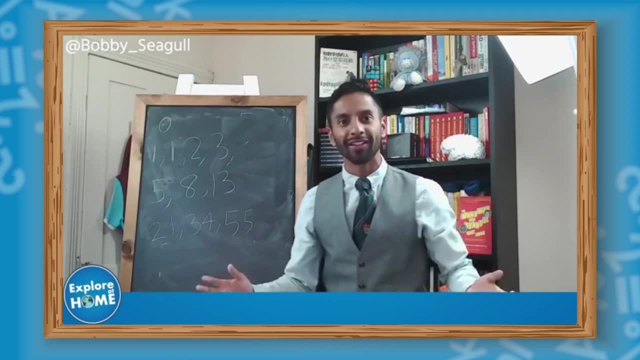 34,, 55,, yeah, It keeps adding up And this turns into 1.618.. And that is sequences for today. Sequences, So you can see, sequences can help us work out when things go up, when things go down. 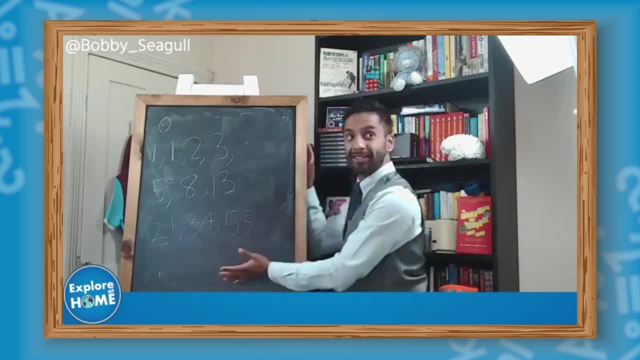 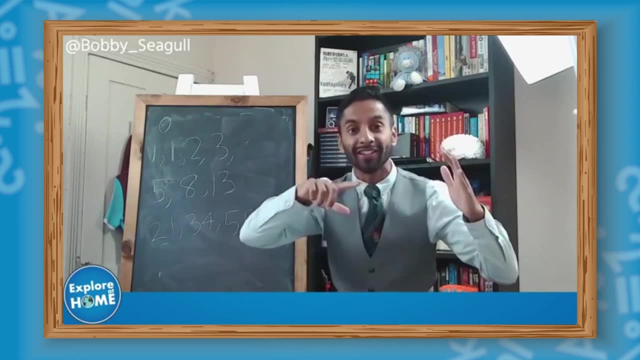 when things stay the same. Or you can look at things like this: Siobhan and Sean, the golden ratio About 1.618.. And you see it everywhere, In universes, In famous paintings. A wonderful structure, So. 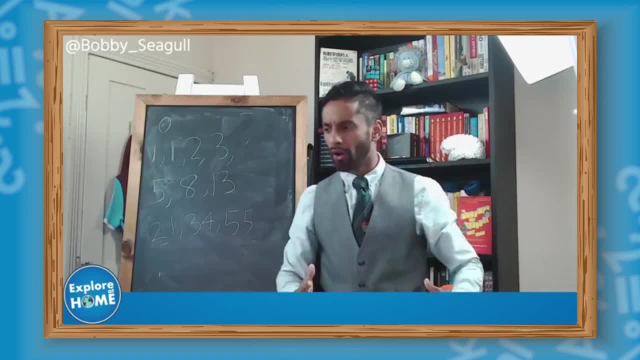 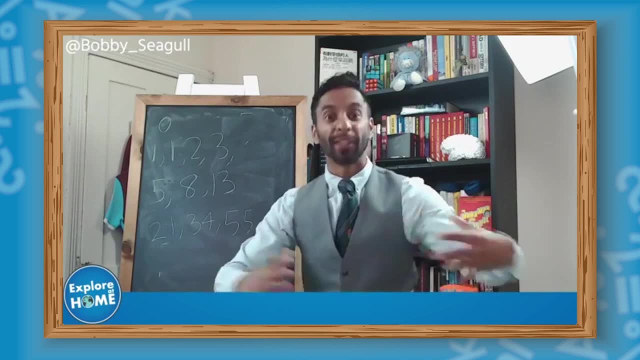 So Where are we now? It's time for Thoughts of Mr Seagull. Thoughts of Mr Seagull: So this is going to be related. So someone's saying I'm going a bit fast, There's a lot of content. 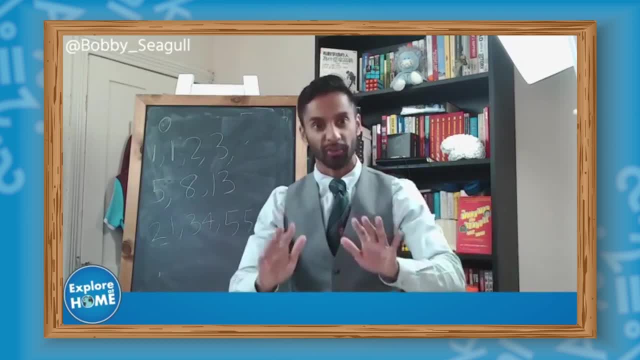 And what I would say is: you can always watch the video back, Always watch it back. So you've got your own time. You can watch it straight after. So Thoughts of Mr Seagull, So I want you to take a deep breath. 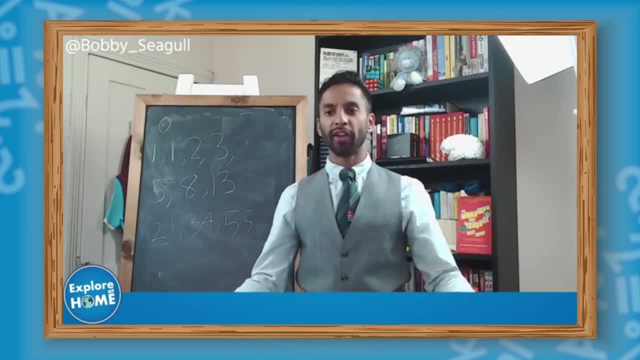 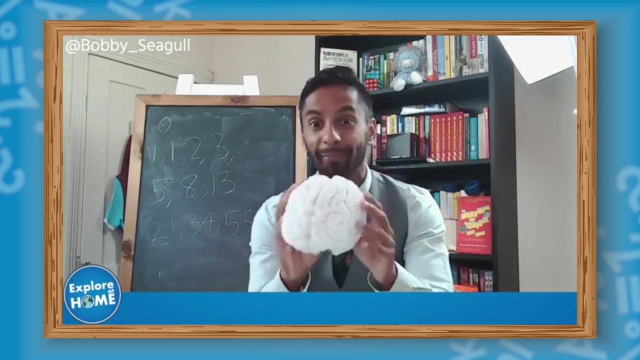 And then breathe out, Deep breath in And breathe out. Okay, So This is going to be related to a scene from the BBC programme on Monday. So on Monday my brain was scanned. My brain was scanned for a programme called The Great British Intelligence Test. 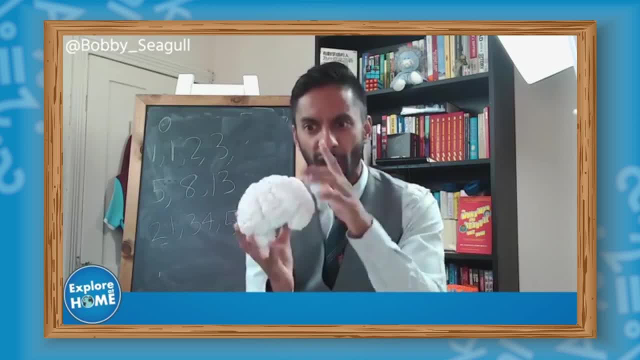 And they wanted to find out. is my brain any different to other people? And we're going to see it, Chris. we're going to see it. We're going to show you the scene here. Hold on, Let me get up in the scene. 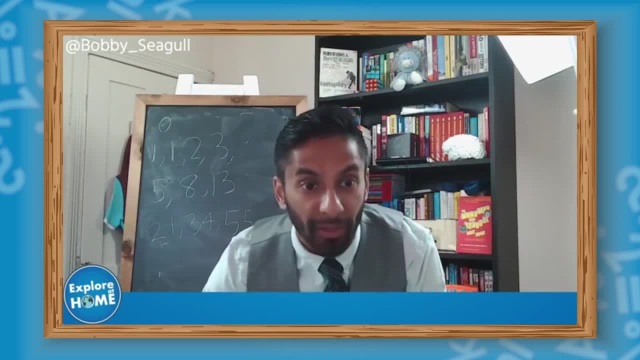 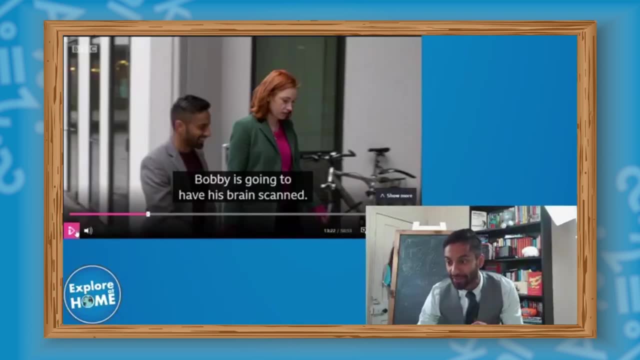 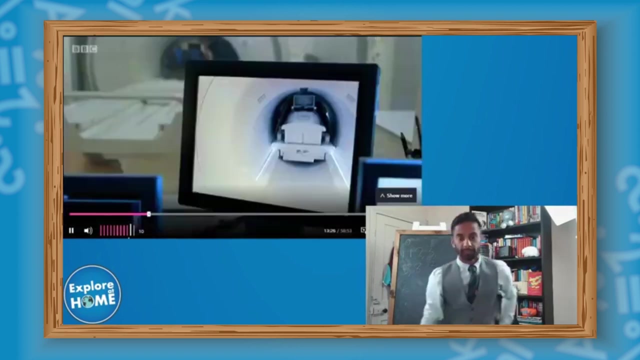 So this is on Monday And let me bring it up. Let me bring it up, Here we go, So have a go. And our lesson are Thoughts of Mr Seagulls related, So have a listen. Experts at the University of Edinburgh. 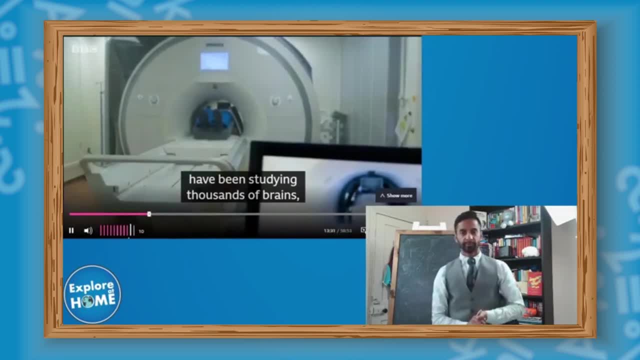 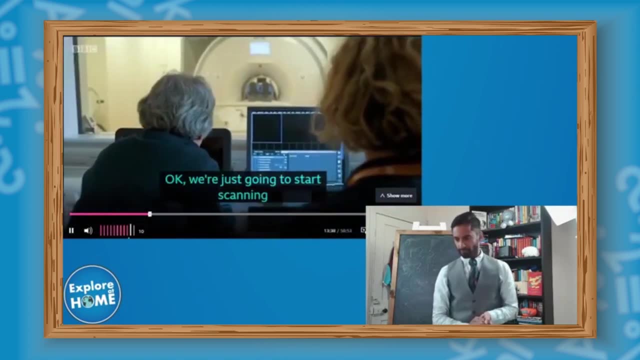 have been studying thousands of brains, searching for anything that might make some cleverer or faster than others. Okay, We're just going to start scanning and it's going to get very noisy. Are clever brains bigger? Are they wired differently? Are you all right there? 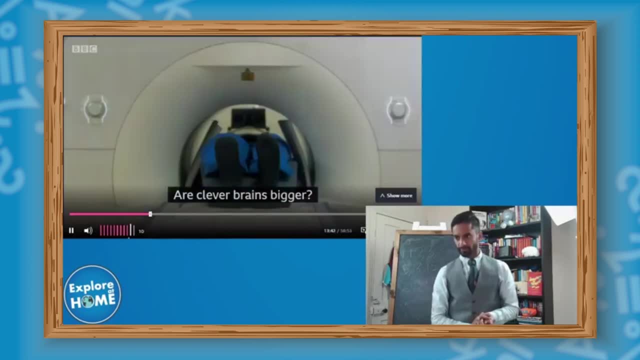 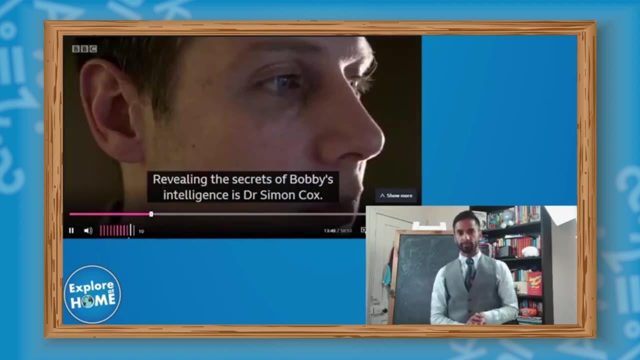 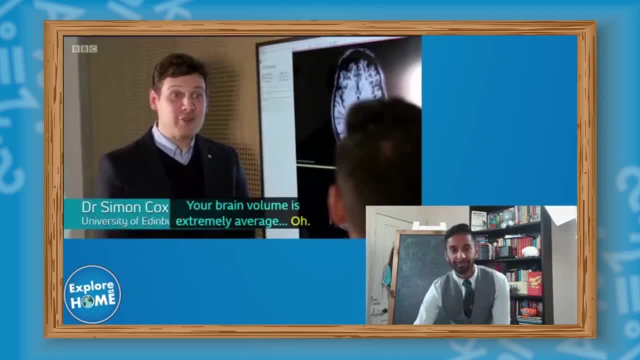 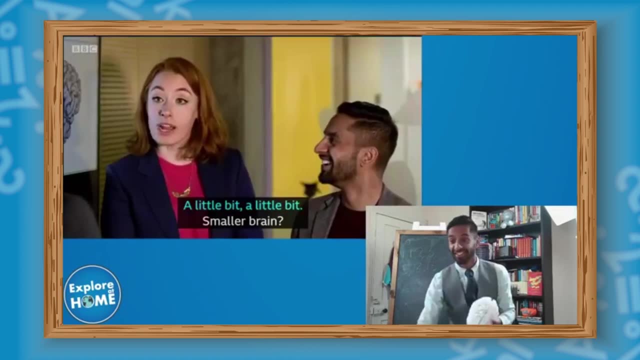 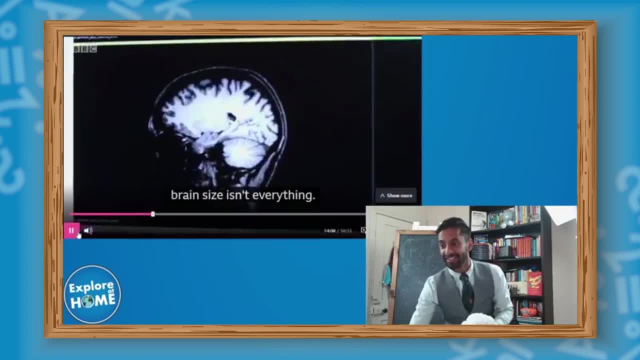 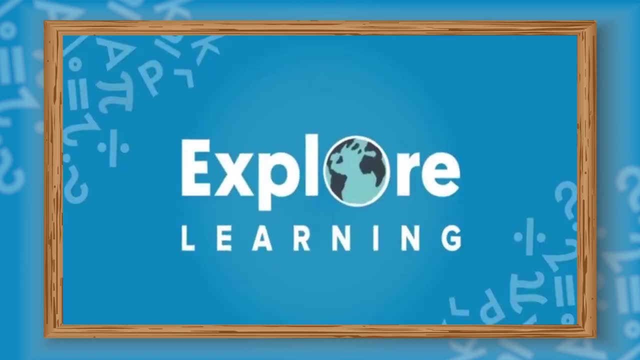 Oh, Bobbie, Clearly, when it comes to intelligence, brain size isn't everything. But is there something in Bobbie? So did you see my face? Did you see my face when they said your brain is smaller? I thought 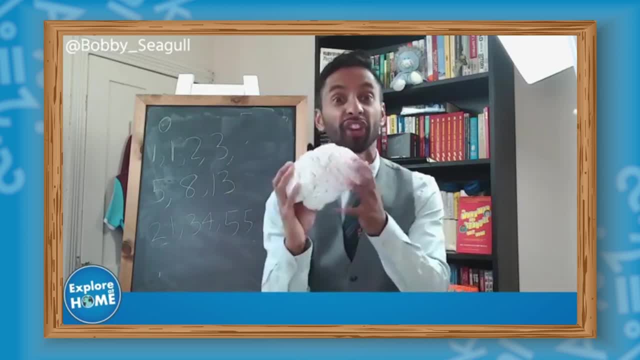 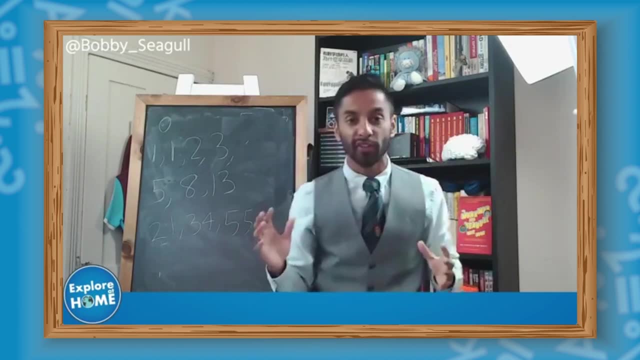 oh, is there something special? Actually, they said there's nothing special about my brain, And this is where the thought comes today. It's not about. it's not about the physical size of your brain. I think it's a lot what goes on here. 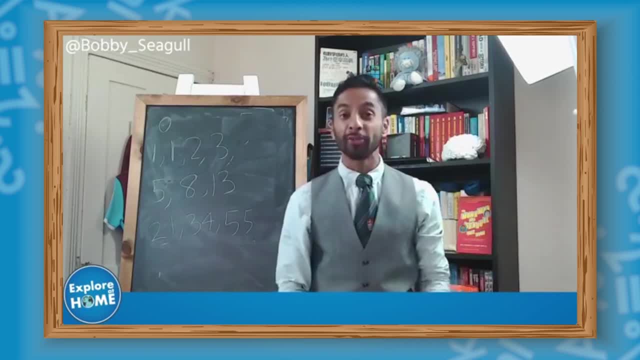 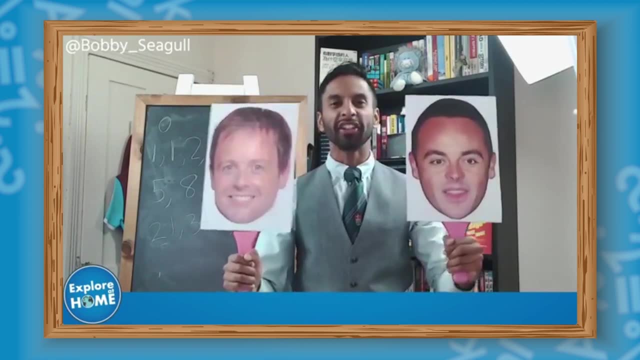 It's your attitude and mindset. Do you remember? a few weeks ago- you may have seen this before- I had these two guys here. We know these two guys, Ant and Dec. Ant and Dec. And imagine these were just two fictional characters. 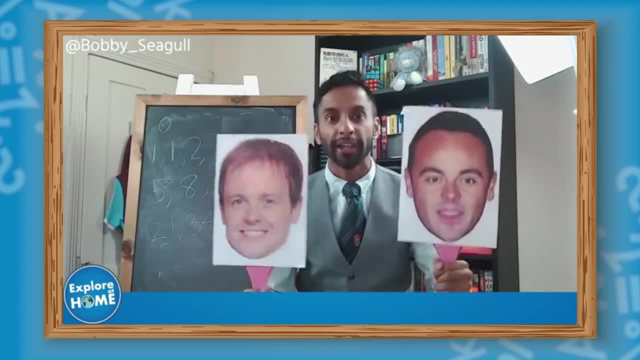 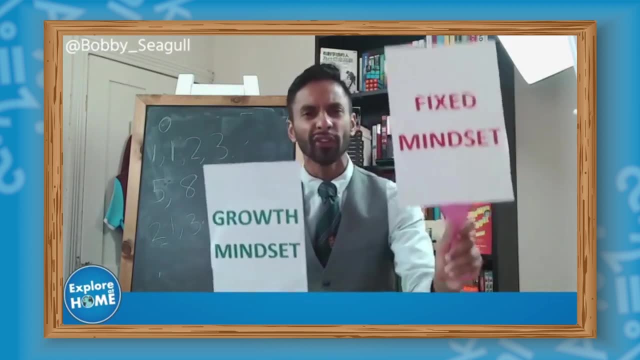 And one of them thinks that they can do maths and one thinks they can't. And there's one difference between the two people. It's their mindset. It's not about the brain, It's about your mindset If you're someone that says: 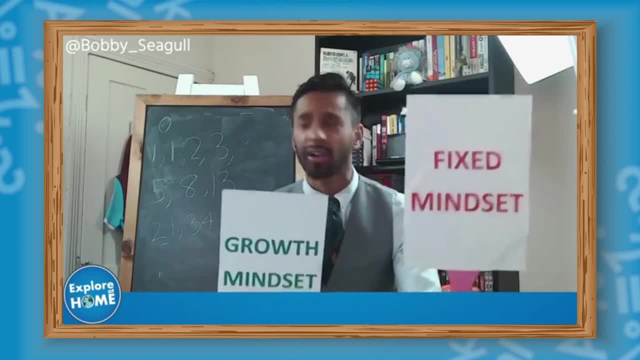 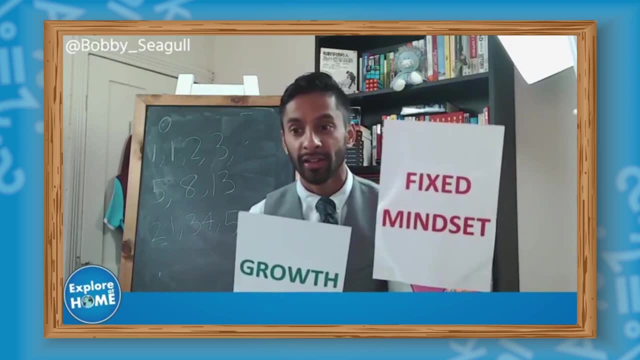 oh, maths is difficult, I haven't got a maths brain. Oh, I can't cook, Oh I can't dance, Oh I can't draw. Then you have a fixed mindset, Whereas if you're someone with a growth mindset, 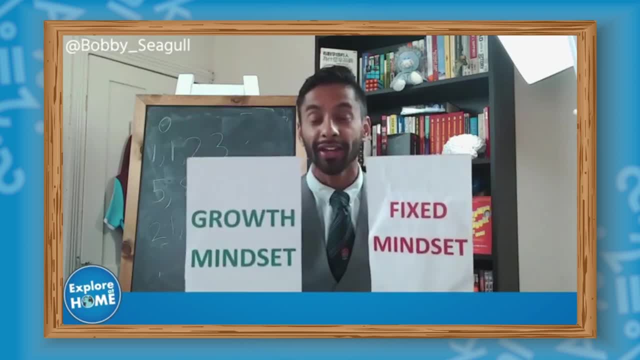 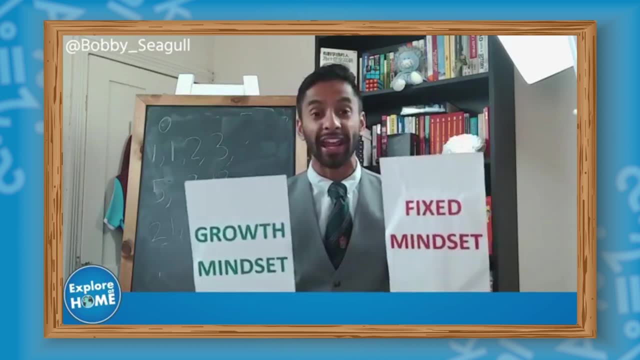 then you think, oh, actually, if I work hard at things, I can improve. I can improve. And that's the the thought of Mr Seagull today. It's your mindset. It's your mindset that makes a difference. 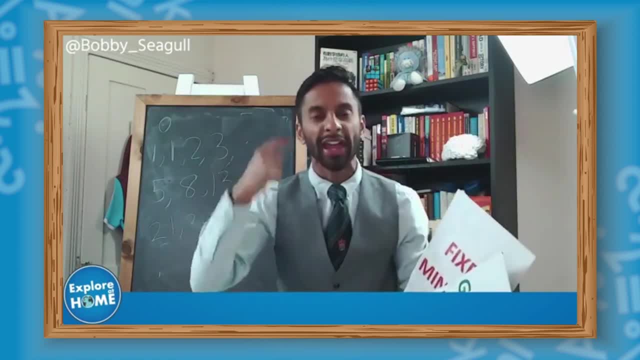 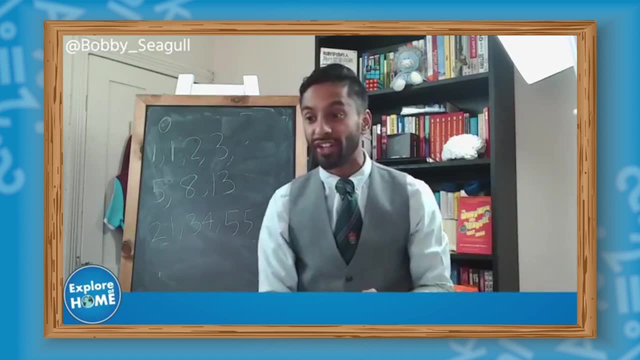 Not the size of your brain, Not what you got going on, It's your heart and what you think about that. And you can actually find this on BBC iPlayer. It's called The Great British Intelligence Test, So if you look at it there, 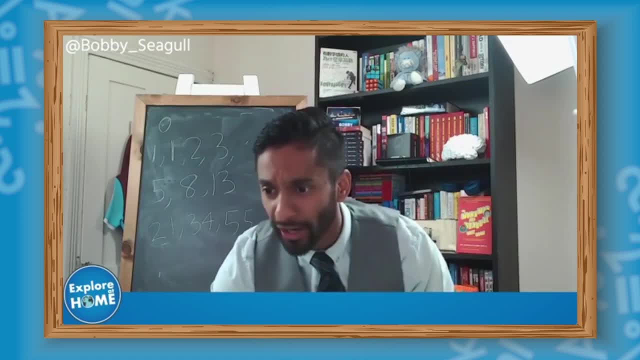 you can find it there. So let me try and find what other things are going on. So we've got a few messages. We've got a few messages coming up. Let's have a look. So this is the program on BBC iPlayer. 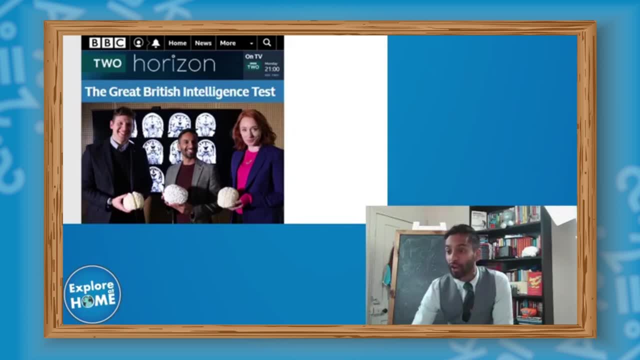 It's called The Great British Intelligence Test. If you have a look on BBC iPlayer, you'll see BBC iPlayer. You'll be able to find it there, And then next week I'll be able to give you an announcement when my new TV series 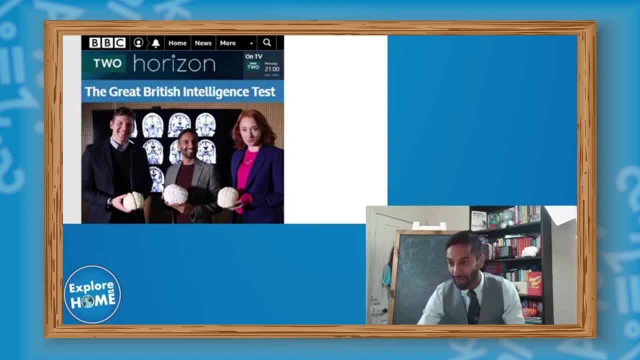 comes out. So it's Monkman and Seagull's Genius Adventures, And that's coming out very soon. So I've got a few announcements to make. So also on that, if you want to see me being very positive, 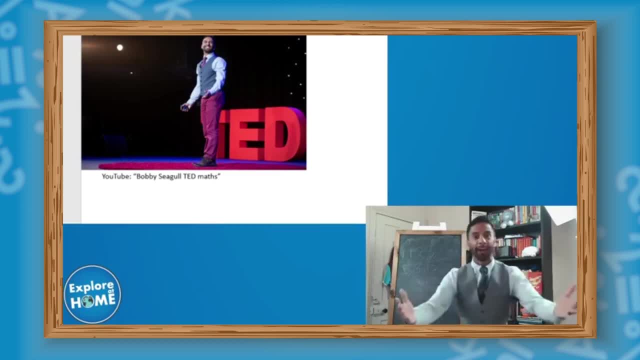 again. if you go to my Facebook- facebookcom- forward slash, Bobby Seagull. do follow me there and you'll find all my positivity. So one of the things that I'd love you to look at is my TED talk, And it's called. 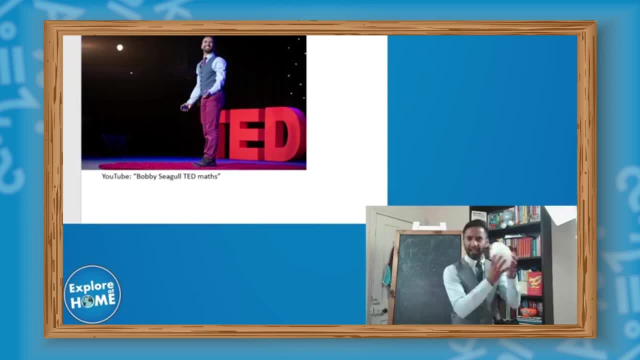 The Magic of Numbers, Why Everyone Loves Maths. As you can see, I don't think it's about your brain. I think it's about your attitude, your heart. Do you really want something? And in my talk, it's worth watching. 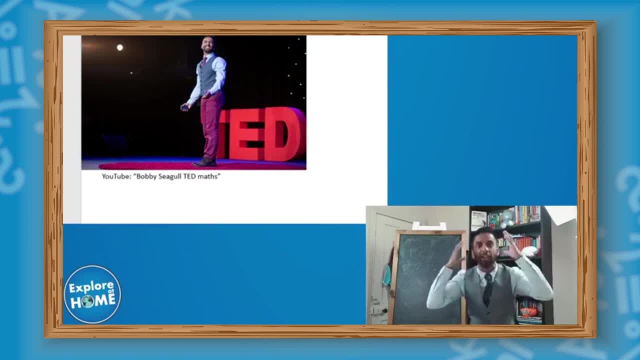 Maybe even after this. it's about how actually your mindset is the most important thing to being good at maths, science, English, cooking, dancing- All things need a positive mindset. So here's a question coming from a parent. A question coming. 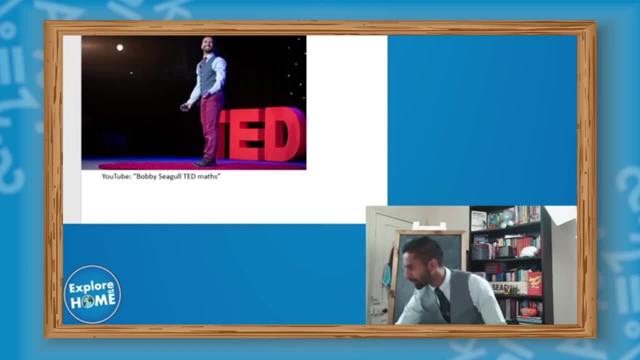 from a parent. So the question is: let's have a look. So the question was: we're finding it hard to get through all the activities set by the school. What should we do? And that's a great question, because there are 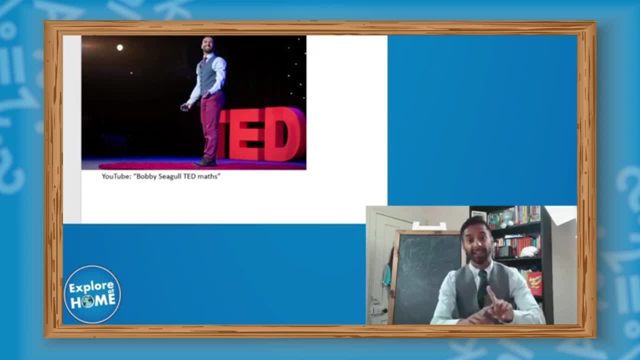 lots of things that you should be doing, lots of activities, And I would say, first thing is perhaps speak to your school. Maybe speak to your form teacher if you're in secondary or if you're in primary school, speak to your class teacher. 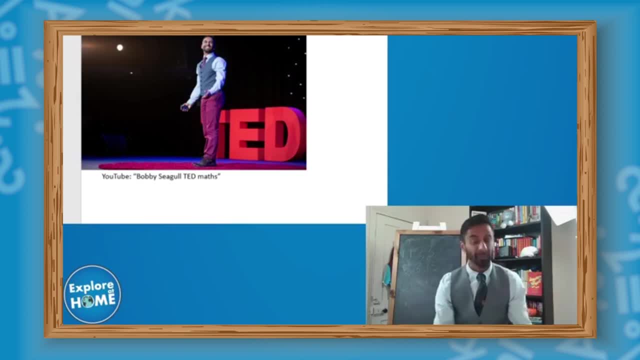 And then the second thing is: don't put too much pressure on yourself, because normally in school you know you go to lessons, the teacher will check up on your work, they'll come round the classroom, Whereas now you're at home. 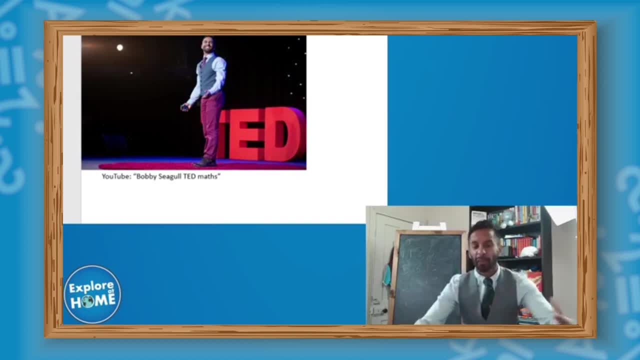 and it's more difficult for that to happen. So I would say: don't worry too much, Don't put too much pressure. Try and do as much as you can, but if you don't make as much progress as you want, it's okay. 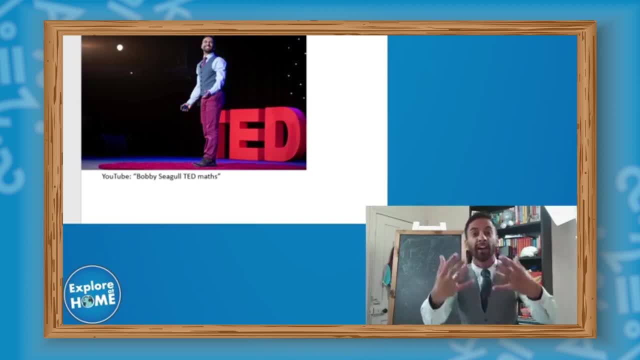 We are in unusual circumstances And again that's why we put on these live lessons for you In these difficult times. So again, someone said they follow me on Facebook. So again facebookcom forward slash. Bobby Segal, Again I'm on Twitter. 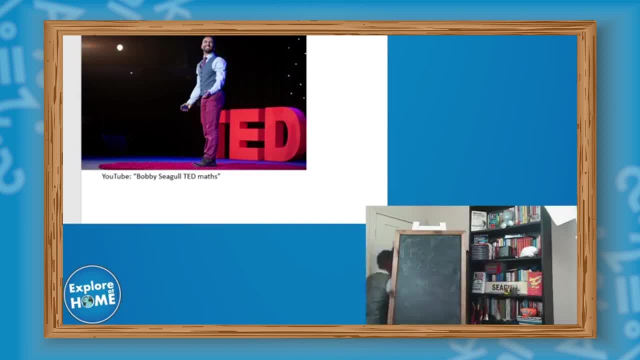 Instagram, YouTube at Bobby underscore Segal and on TikTok. Let me bring back the banner, So we're about to look at the last few messages. Last few messages. I'll bring this back here. Bring this back here, Okay. 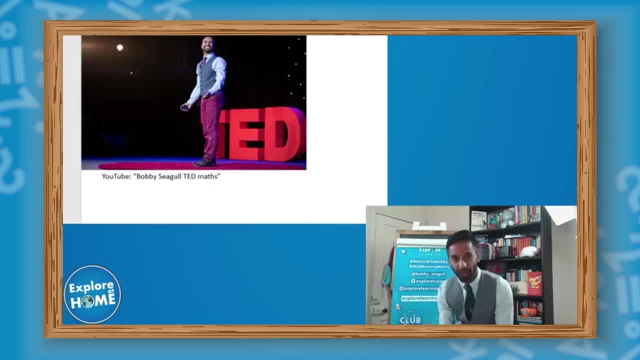 So let's see what else is going on. So obviously, Explore at Home has this new. it's really sparkling. It's a great website. It's not a new website, but let me bring up the main scene so you can see. 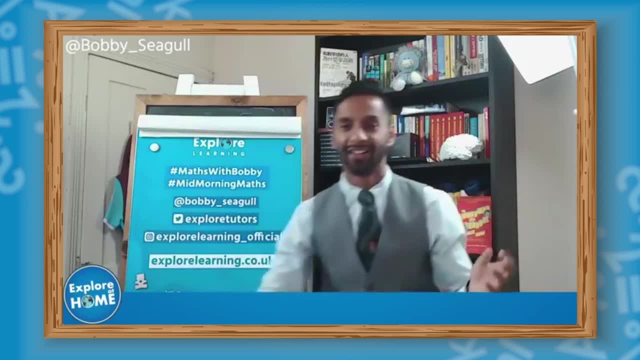 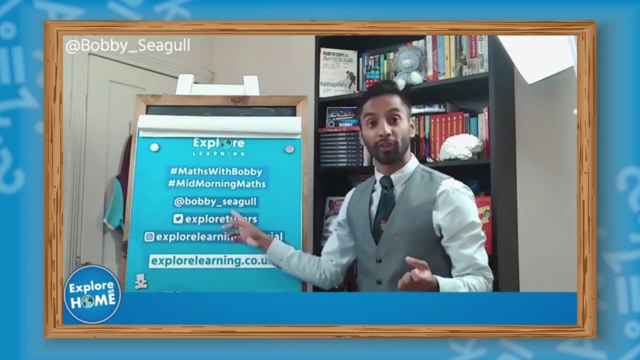 So there you go. So we've got my TED talk. I'd love you to see. So again, hashtag Maths with Bobby at Bobby underscore Segal on Twitter, Instagram and Facebook. you can find me YouTube as well. We're at. 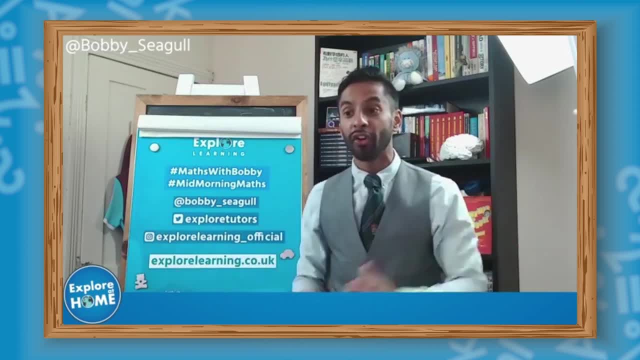 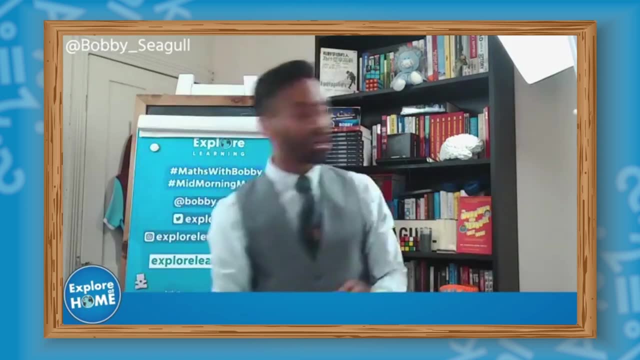 Explore Tutors and we're at Explore Learning of you doing lessons. Ellie says it's her birthday this Saturday, So happy birthday to Ellie. Sam wants to know where you can buy my book, So, Sam, let me show you a copy of my book. 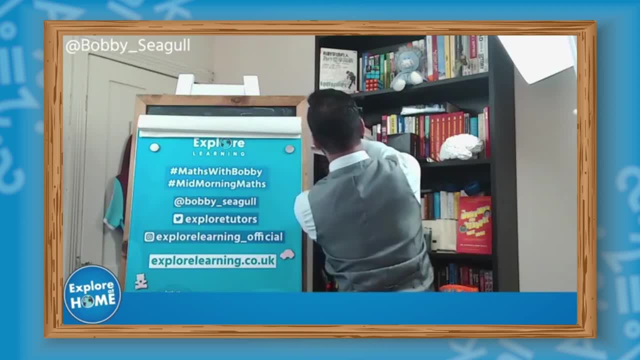 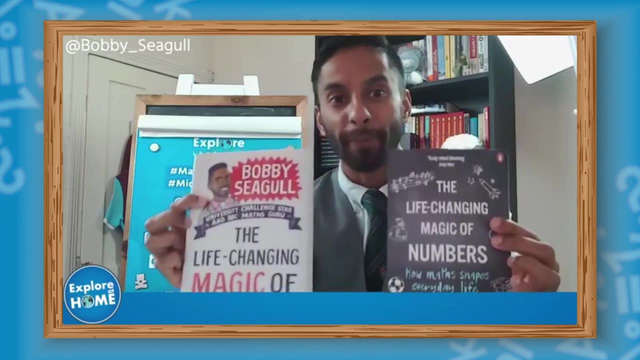 So, Sam, if you actually go to again, if you check Twitter or Instagram or my Facebook, a lot of details are there. So I've got it's the same book. This is a hardcover, This is the paperback. 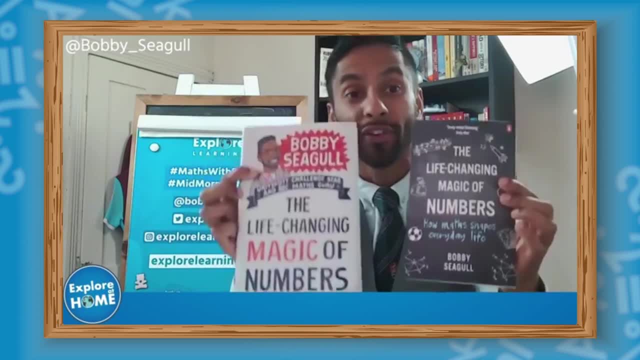 It's called The Life Changing Magic of Numbers. All of us can do maths. You can see my face, Smiley face, Smiley face. So that's the paperback, or the hardback as well, So you can get this on Amazon. 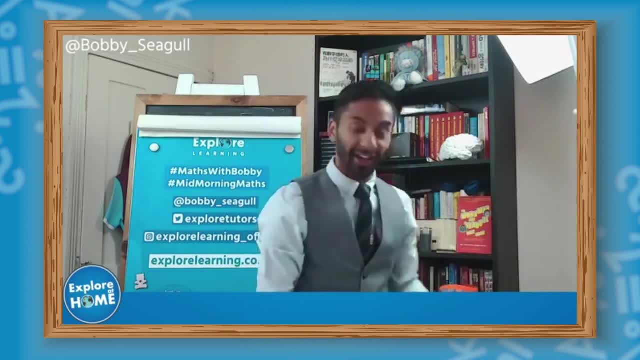 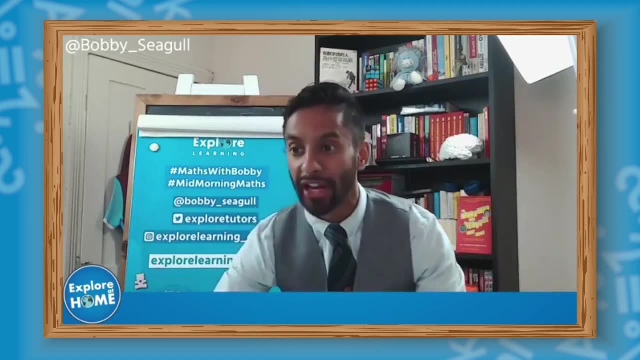 It's called The Life Changing Magic of Numbers. Happy birthday to Leah, who turns nine, Who turns nine on Saturday. Lots of birthdays, Actually. one other thing: I'd love you to get involved If you love maths, if you love learning. 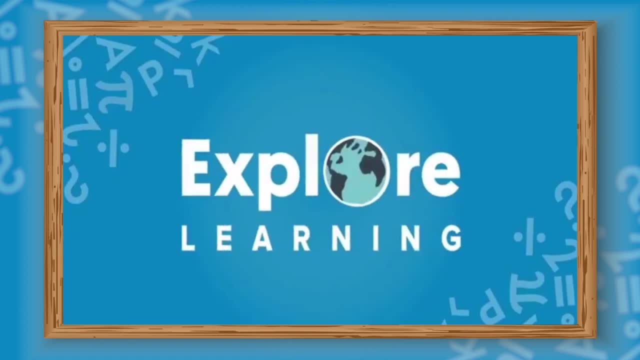 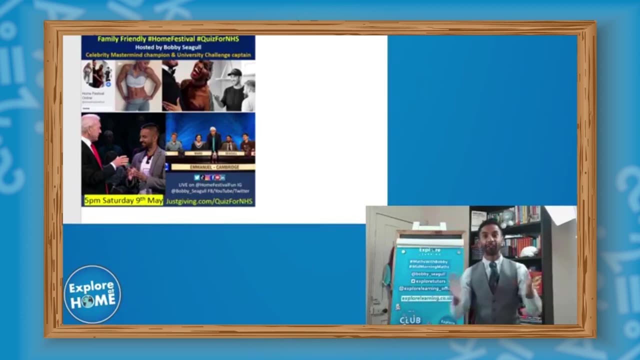 come along on Saturday, Let's get this back. Come along on Saturday, So I do family friendly quizzes. So I do family friendly quizzes. There's maths, There's primary school maths questions. There's charades. I act out. 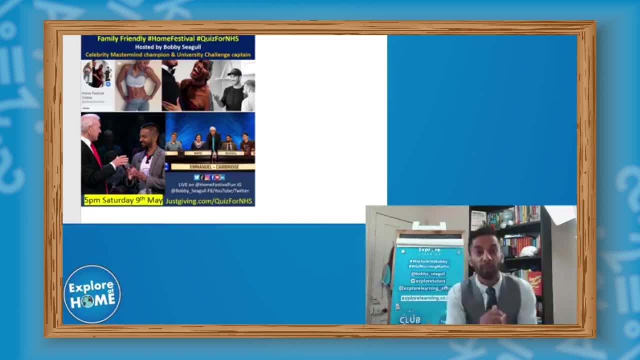 You can see I'm crazy with my boxing routine. I do a music round, I do a pitches round And even if you're a fan of Strictly, some of the Strictly dancers do charades for my quiz. So it's called. 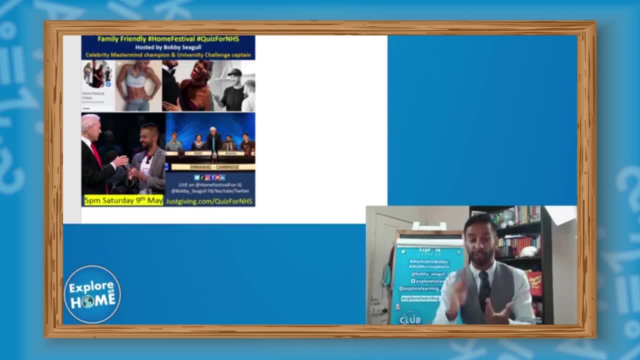 Quiz for NHS. If you go and check my Twitter, my Facebook, my YouTube- all details there- And we have lots of members from Explore Learning that take part, So that's wonderful. So please do join in on that on Saturday. 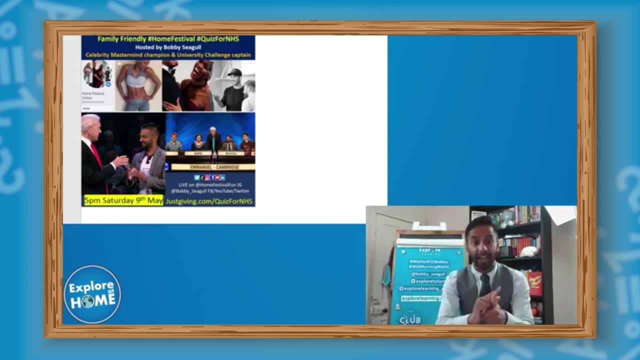 So let's have a look. We're going to look at the rap we learned today and we're also going to have a a look at a few shout outs towards the end. So the rap today was about Fibonacci. Remember? Fibonacci went 1. 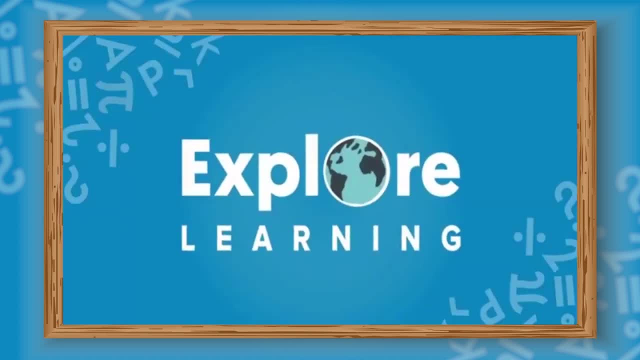 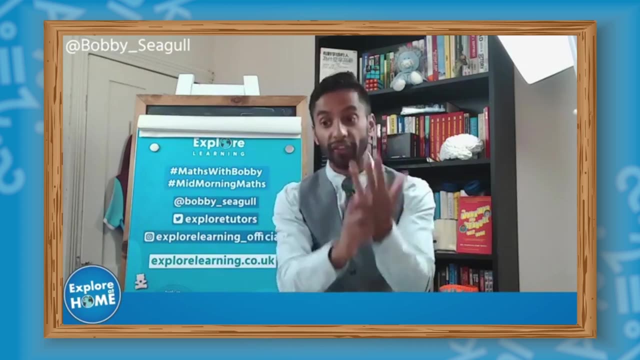 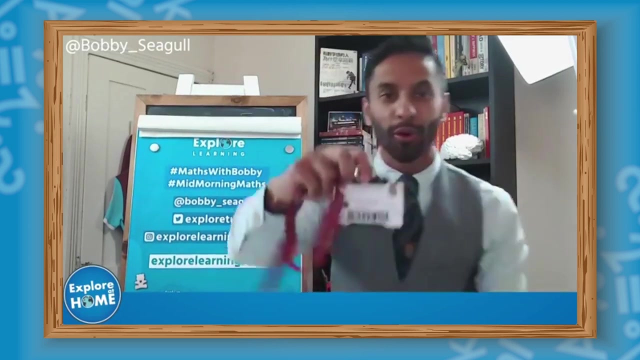 1. I'll pause there for a second, So Fibonacci goes: 1, 1, 2, 3, 5, 8, 13, 5 8 13, 14, 15, 16, 17, 18, 19, 20, 21, 22. 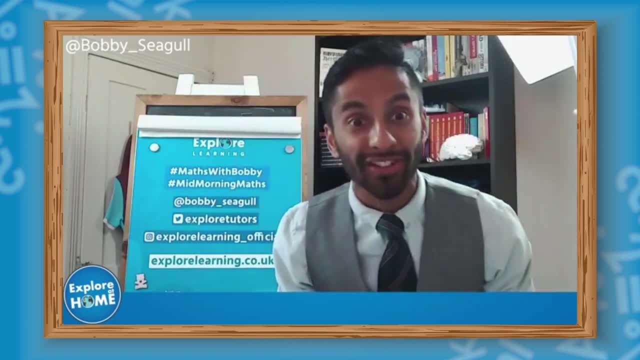 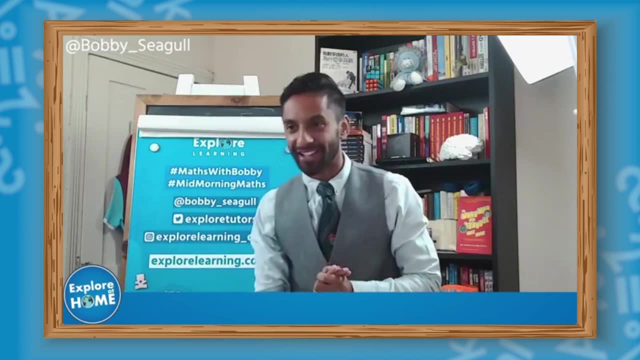 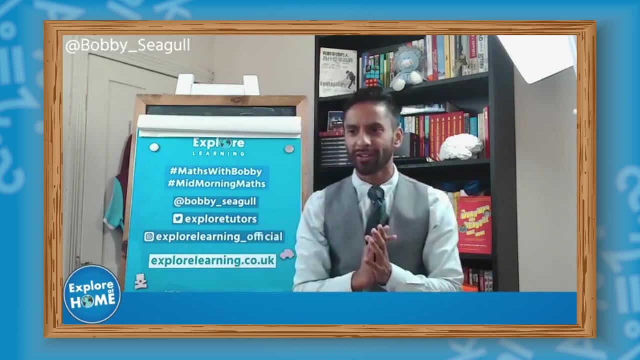 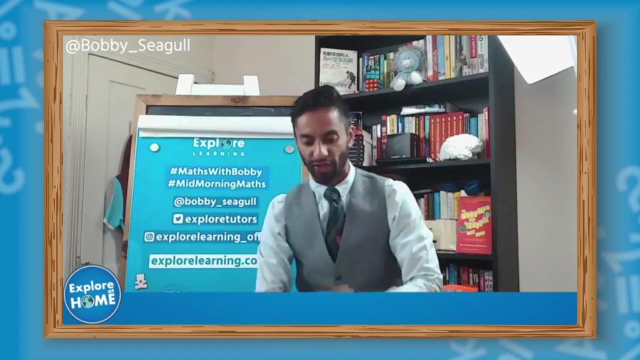 23, 24, 25, 26, 27, 28, 29, 30, 31, 32, 33, 34, 35, 36, 37, 38, 38, 39, 40, 41, 42, 43, 44, 45, 46, 47. 48, 49, 50, 51, 52, 53, 54, 55, 56, 57, 68, 79, 80, 81, 82, 83, 84, 85, 86, 87, 88, 89, 90, 91, 92, 93. 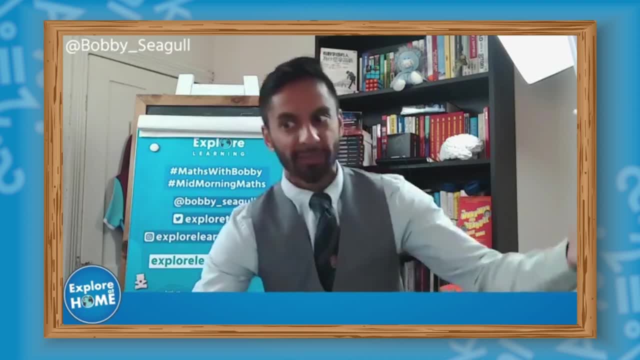 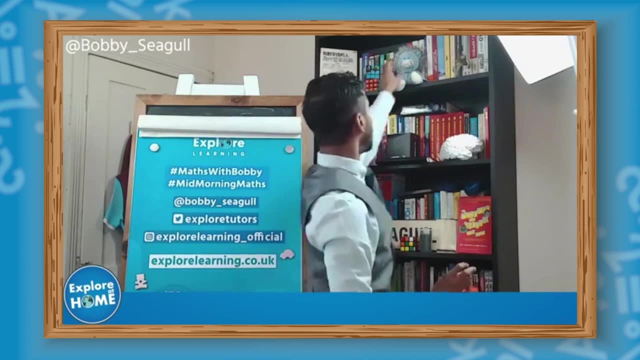 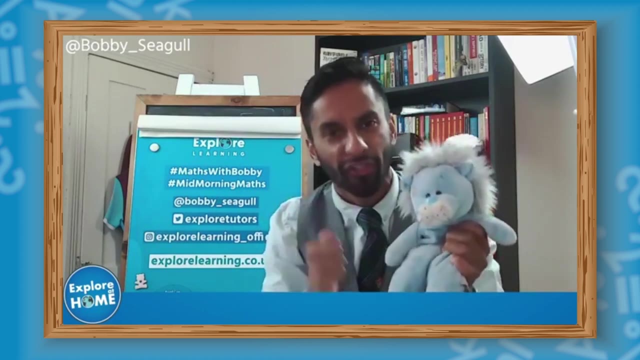 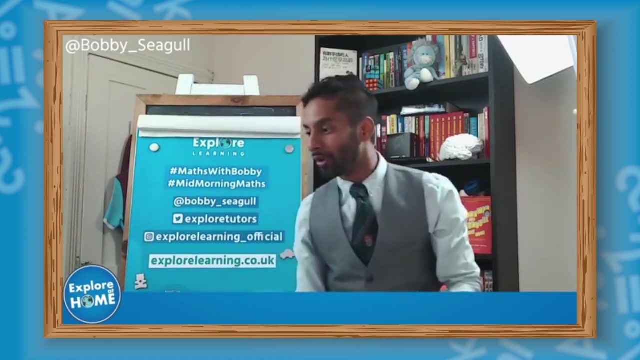 94, 95, 96, 97, 98, 98, 99, 100, 100, 10, 10, 21, 24, 25, 26, 27, 26, 27, 28, 29, 30, 31, 32, 33, 32, 33. 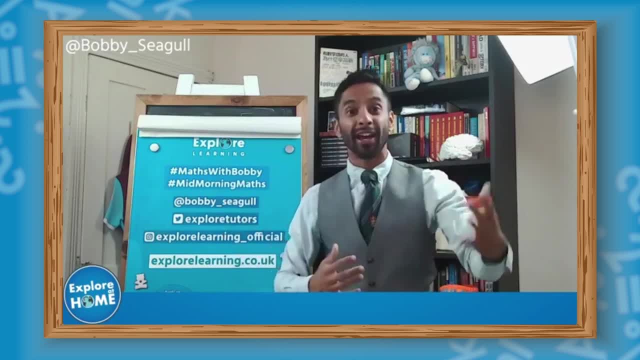 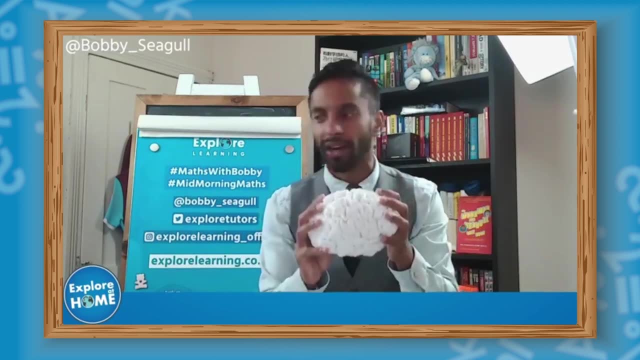 34: Explore Learning. we're all about Amir, about fearlessness. Remember, people look at my brain and go: Bobby, is your brain naturally smart? We're not. It's not about being naturally smart At Explore. it's all about being fearless, trying things. 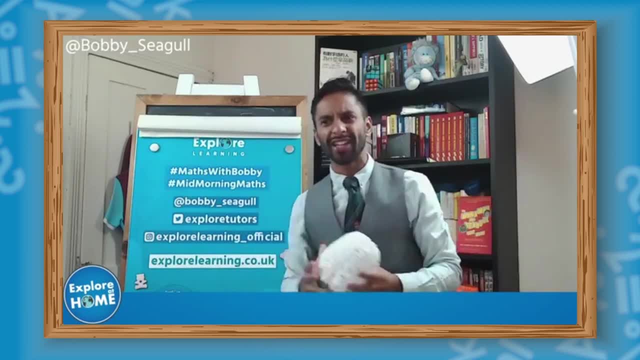 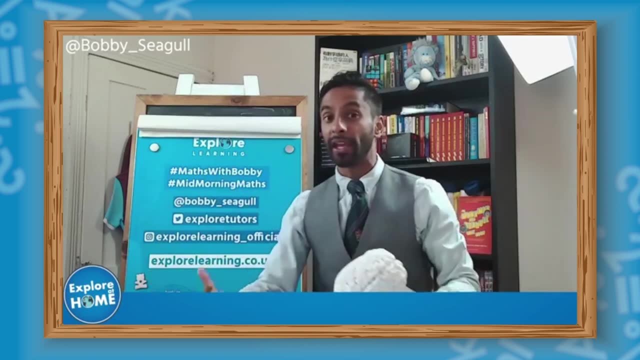 out And a few of you today looked at the golden ratio and said that's quite tricky. I'm not sure what's going on, But if you're fearless, you keep going, you come back, maybe watch the video again, maybe speak to parents. check out YouTube. 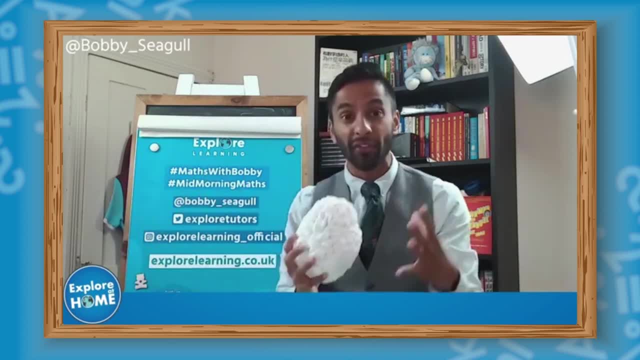 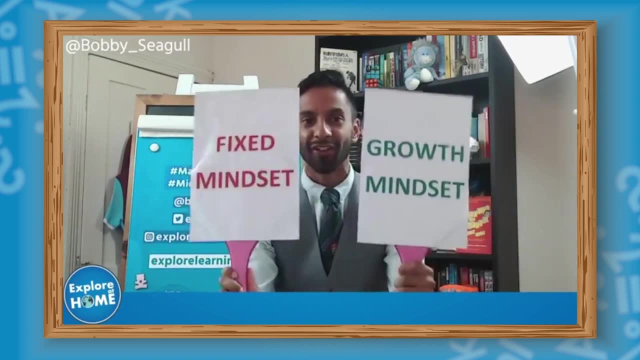 videos, check out, Explore Learning's website and try and keep delving in, because maths is all about your attitude. Remember we need, we need- if you look at these two guys here: we need growth mindset, not fixed mindset. we need. 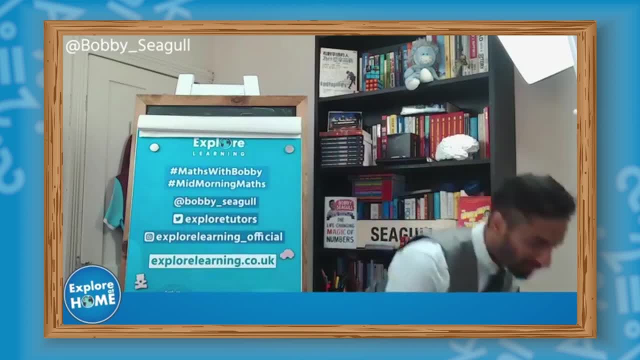 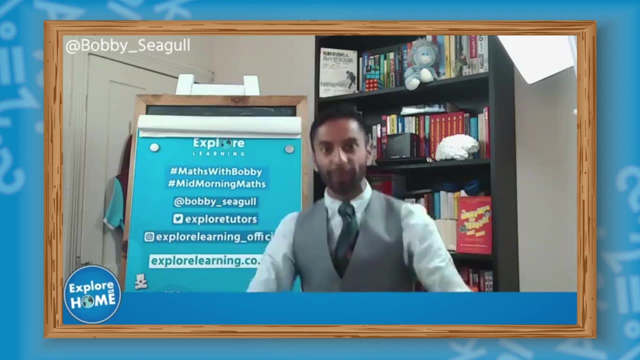 growth mindset. That's what we need And all of us can do that. So thank you all so much. So we are back on Friday with Key Stage 3.. So if you want to progress with sequences and we do some fun stuff next week, on Wednesday is National. 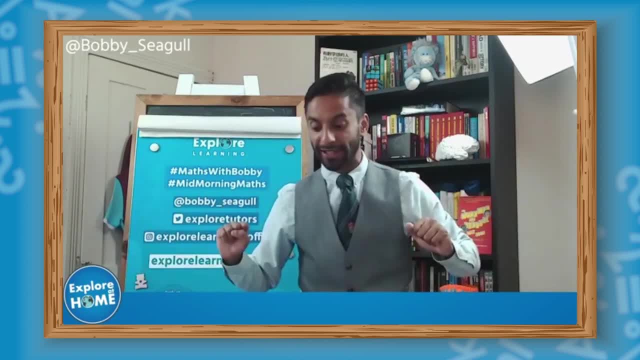 Numeracy Day, So that's gonna be amazing. We're gonna have new people join us for that particular day. And again, make sure you've got Explore Learning- ExploreLearningcouk. You can find a free trial about how to book an online. 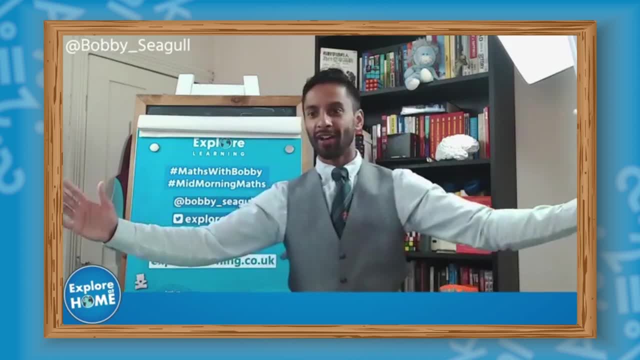 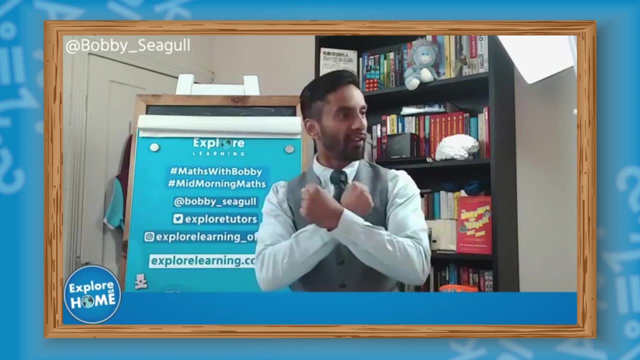 session with us. So do please, do that. So, Harry, we're about to end, We're in stoppage time. We're in stoppage time, And stoppage time means it's time for our rap, A rap. So, Alexander Gabriel, let's do this. Sean Shivan, Hannah's new Kia. 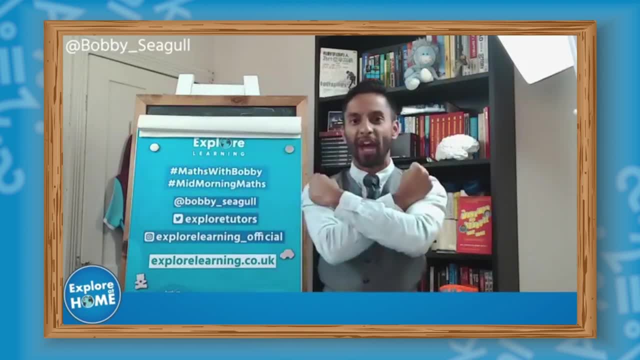 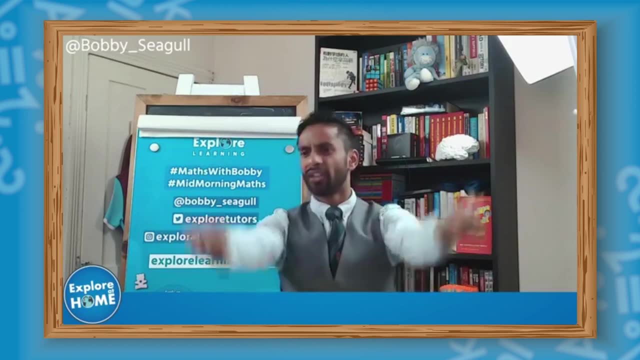 Misha Bianca, let's get involved with our maths rap. So here we go. One, two, three go. Yes, I can do maths. Yes, I can do maths. Yes, I can do maths. Two more times, Salaam, let's do it. Three, two, one go, Dilarah. 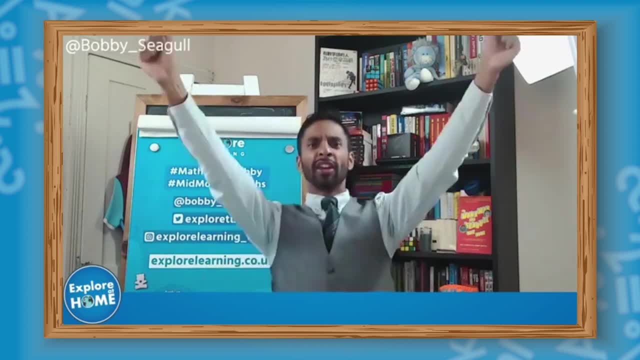 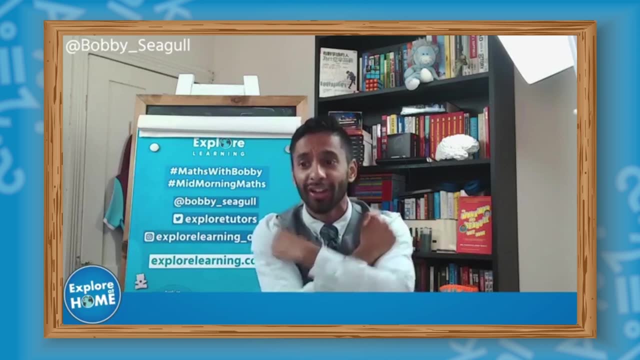 yes, I can do maths, Yes, I can do maths. Yes, I can do maths. And the very last time, let's give it three, a two, a one, One, two, three go. Yes, I can do maths, Yes, I can. 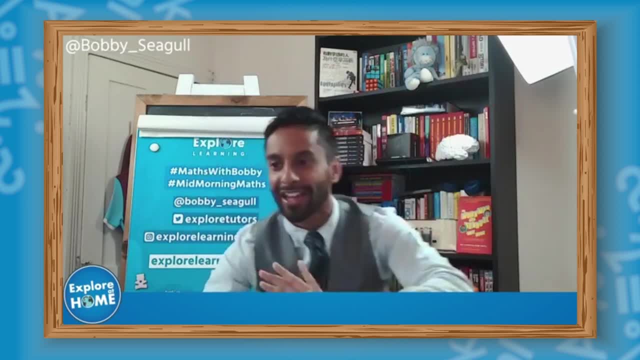 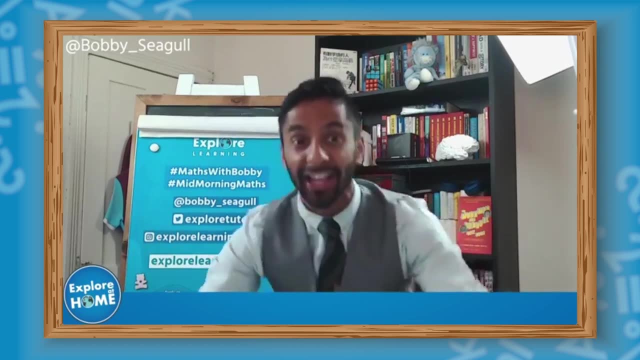 do maths. Yes, I can do maths. Thank you so much. Thank you, Bo, Thank you Beatrice, Thank you Foster Cara, Karen, Zach. You've all been wonderful today. Happy birthday And again if you tweet me.